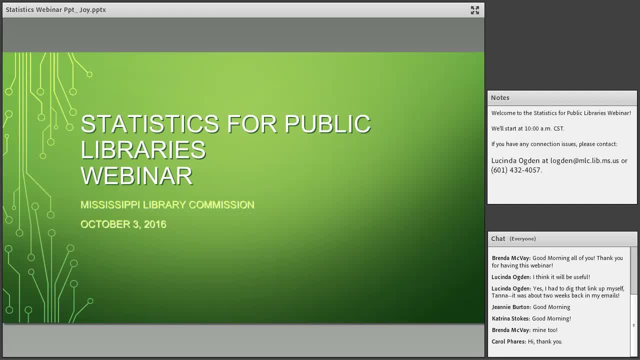 got for you, including the PowerPoint and a reference form, as well as a form about the way to count databases. As always, this webinar is made possible by the Institute for Museum and Library Services, And if there are no questions, we'll go ahead and get started. So today we will. 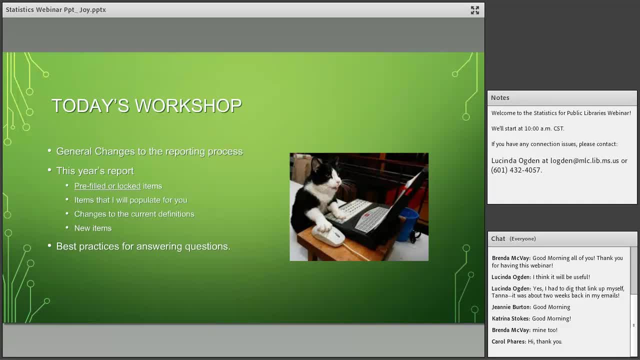 talk about some changes to the reporting process. Those of you who were at the workshop will find much of this familiar, but if there might be something that we went over during the workshop that you did not catch or that you were unclear on, so you're welcome to ask any questions while we go through this today. 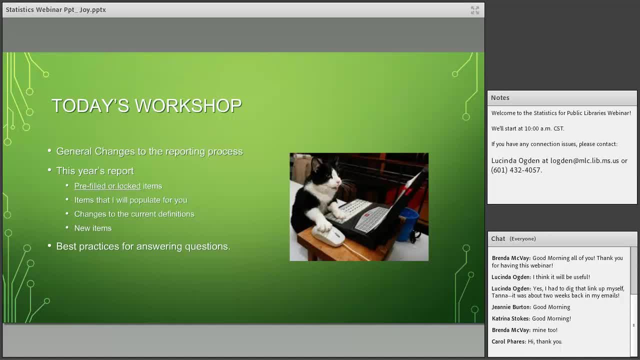 We're going to talk about this year's report. We'll look at the pre-filled and locked items. We'll look at the items that I will populate for you. We will look at changes to the current definitions and we'll look at some new things that we'll 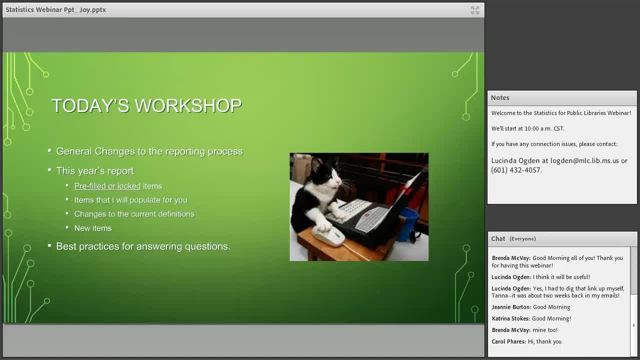 be asking. I'm also going to give you some best practices for answering questions And we will actually look at the report and we will go step by step, and that might be the most helpful thing for you, because you'll be able to see exactly how the report works, If any of you do not have. 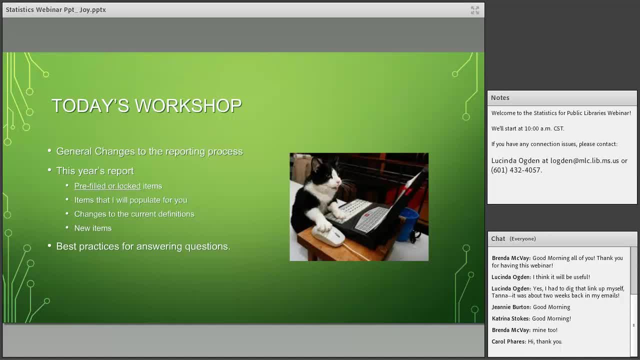 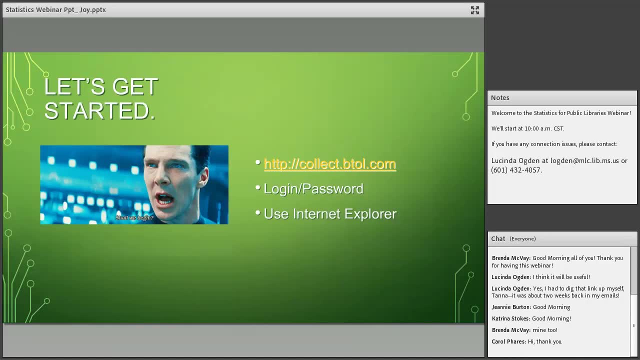 have your username and password for the annual report. please let me know, and I can email that to you after the workshop today. So we're going to get started. I'm going to go to collectbtolcom and just pull up the screen. so if you'll, 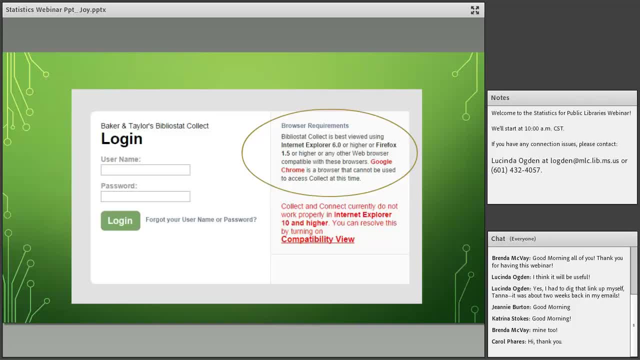 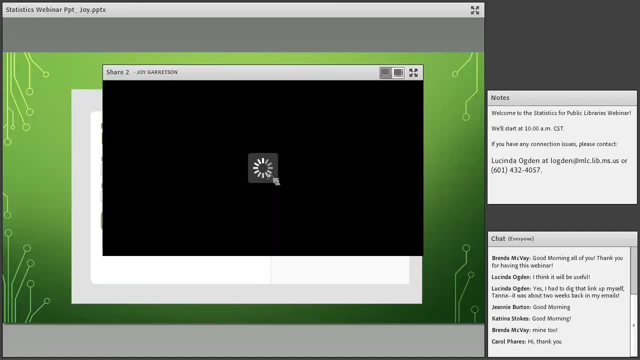 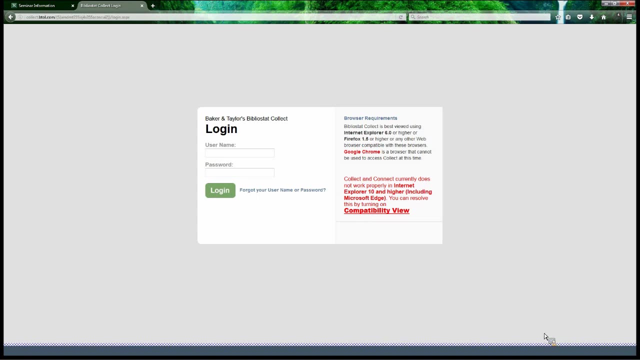 give me a minute. it will take just a moment for us to switch over. Okay, I'm hoping that everybody can see this. You'll notice that on this screen we have the browser requirements and it says that BiblioStack Collect is best viewed using Internet Explorer 6.0 or higher or Firefox 1.5 or higher. Google. 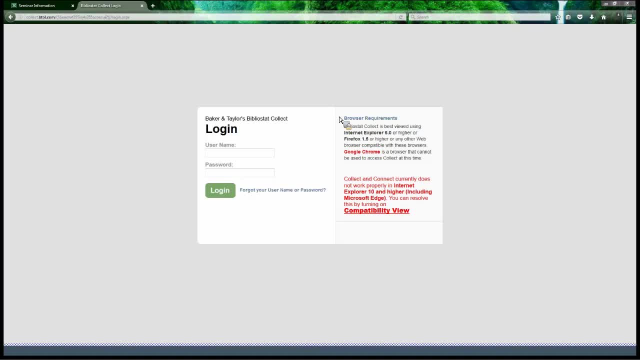 Chrome is not a browser that you should use for this. so I'm just be aware that if you do choose to use it, you might- your information not might not- be saved, and it's not going to be as smooth of a process as if you use. 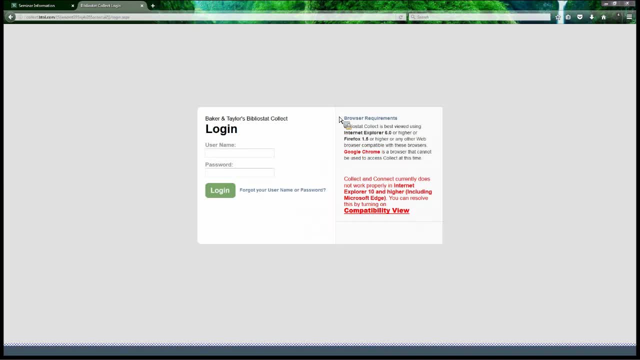 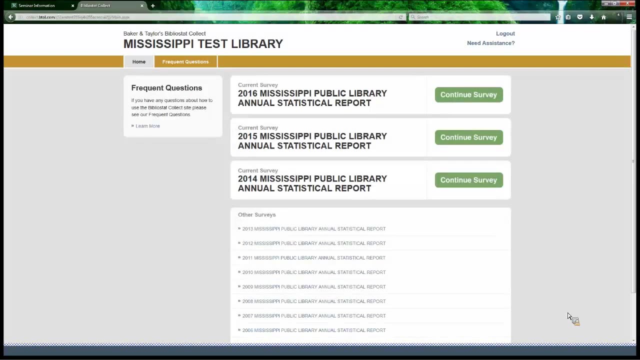 Internet Explorer 6.0 or Firefox 1.5. So I will go ahead and log in here. Okay, Katrina. thanks If you will let me know. if you have any questions, I'll be happy to answer them. If you can hear me, I'm turning my microphone up just a bit, Can everyone? 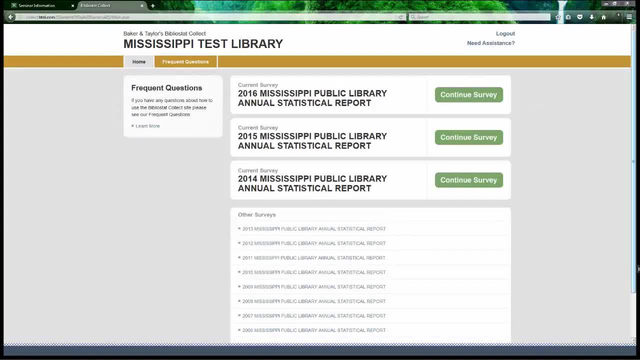 hear me. Okay, that might have come from my switching pages, So y'all just keep me posted on on the audio. So, as of today, the annual report is open for everyone. I will be looking through a test survey, so it won't have as much information. 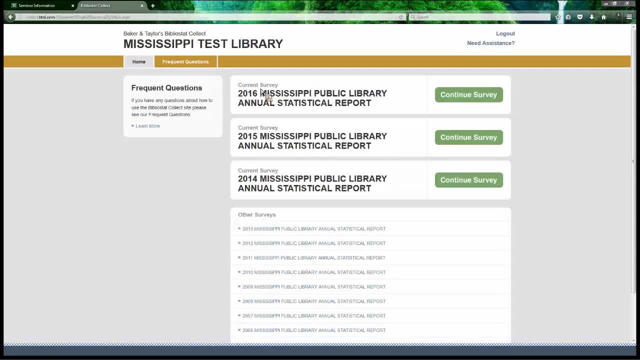 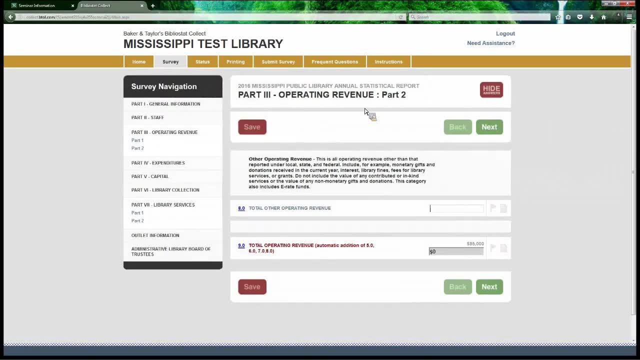 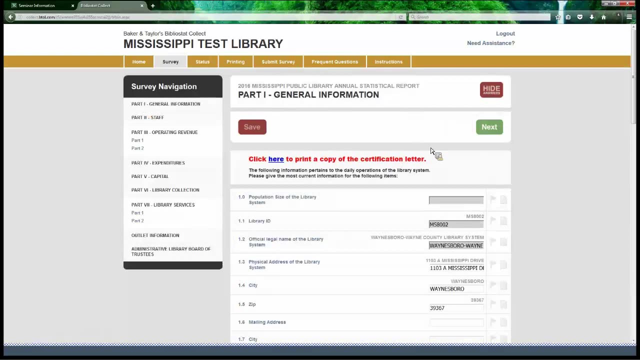 pre-filled, as yours does, But it should look exactly like what you will pull up when you log into the survey. So we will start with the general information And a couple of things. so this year, because we had so many issues last year with people forgetting about- 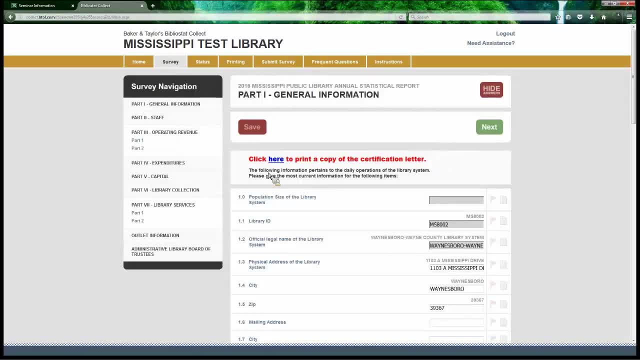 the certification letter. i made sure to put it in bold and read at the top of the survey. So if you want to, you can go ahead and click here at the beginning of your survey process so that you'll have have this printed out. but if you forget and you aren't able to get it before you, 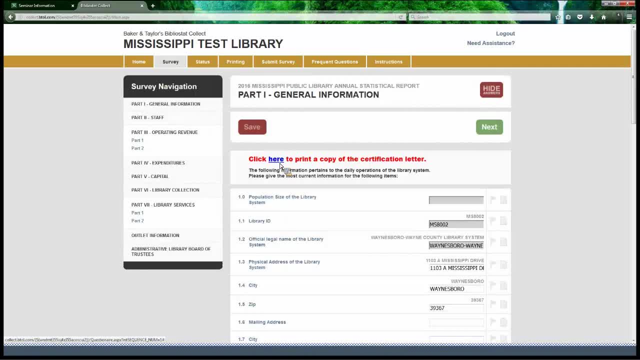 submit your survey. that's okay. I can still send you a copy. I will also let you scan this in to me this year. you don't have to mail it unless you want to. another thing I wanted to mention to you is that some people like to print their 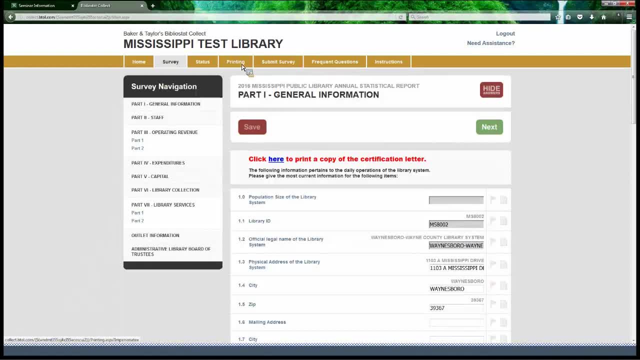 surveys before, before they fill them out. so they'll print a copy of the survey, answer the questions and then come back in and fill them out. you're welcome to do that as well, okay? so, looking at this, there are a couple of items that are always pre filled. on the first page you see the population size I enter that. 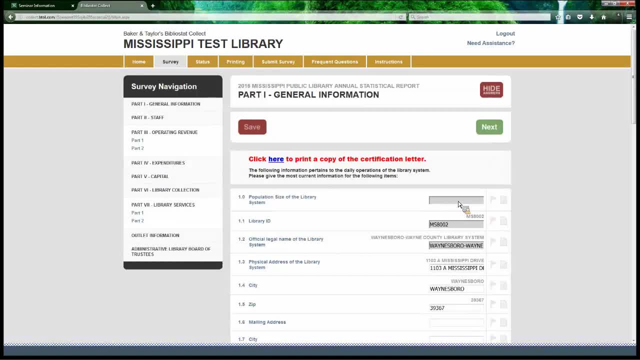 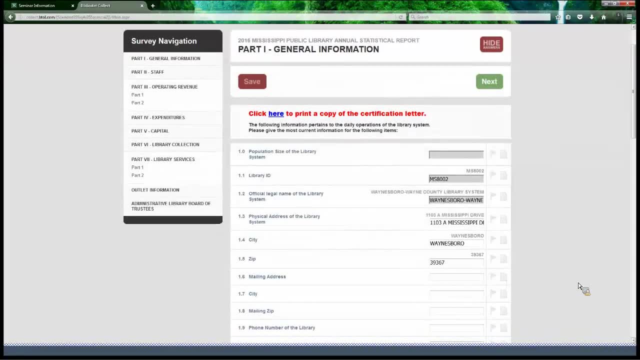 information in at the beginning of April every year. we like to pull our census numbers at the same time every year so that they're consistent. okay, so we also put in your library ID and the official name of your library system. I did Waynesboro, Wayne, тайpsc spring school. 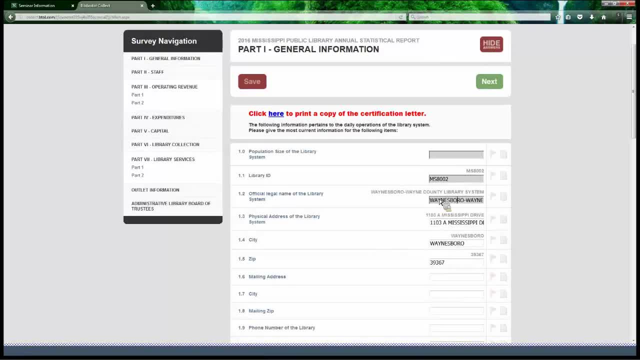 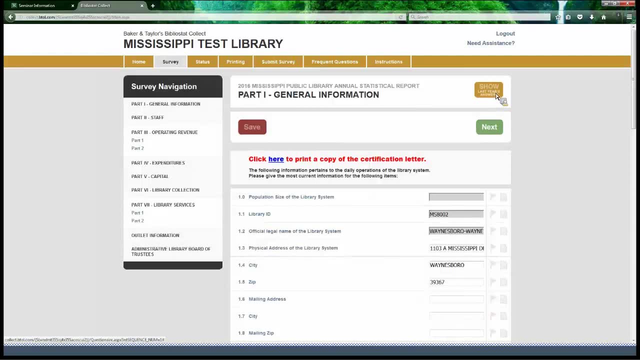 County as a sample a couple years ago, and so that's what comes up in there. I also want to mention to you that you can show last year's answers or hide them. I would strongly suggest that you show the previous year's answers so that you can. 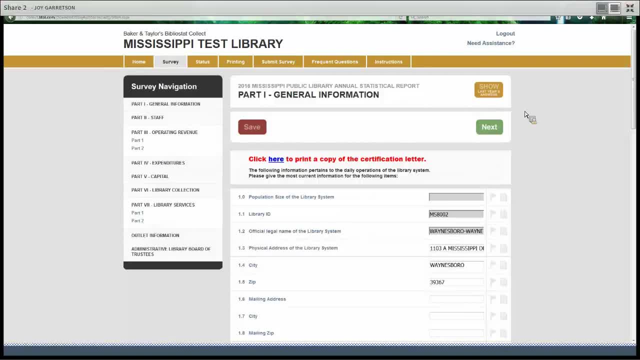 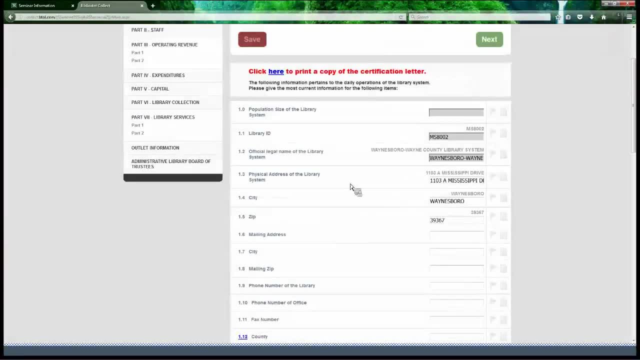 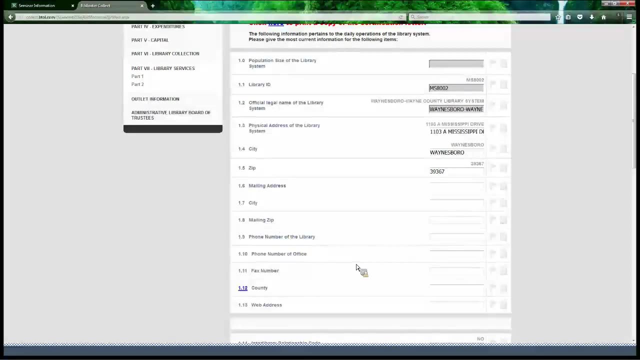 see how much your numbers have changed from this year to the last or from last year to this year. So I just click that here. Okay, most of this information is going to be pre-filled for you here: your mailing address, city, zip, phone number. so. 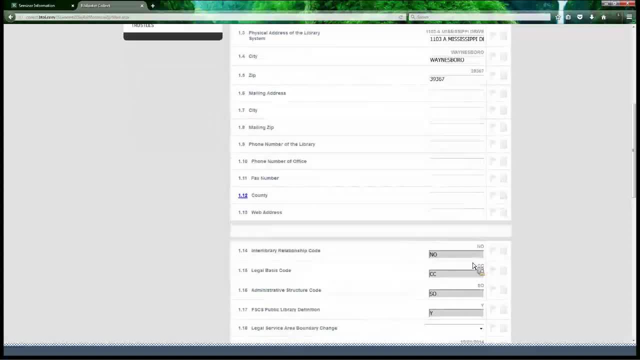 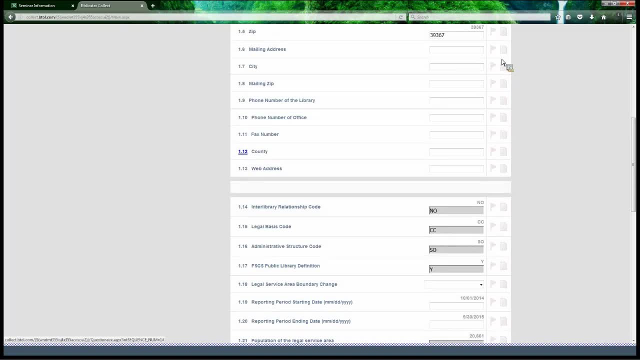 you will not have to change that. Let's see. and if you do decide to change it from the previous year, please just leave a note for me in one of these little note boxes. We did have some questions about where to type all of these notes. 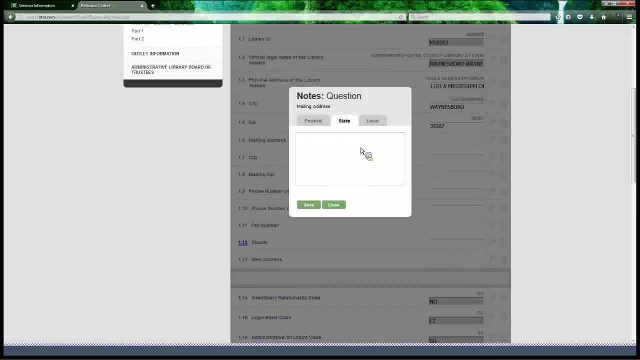 and I would say: just go ahead and type it. You can make your own personal notes for your use in the local tab. The state tab is for me, so I will be looking at especially at the state tab and anything that we need to move over to the 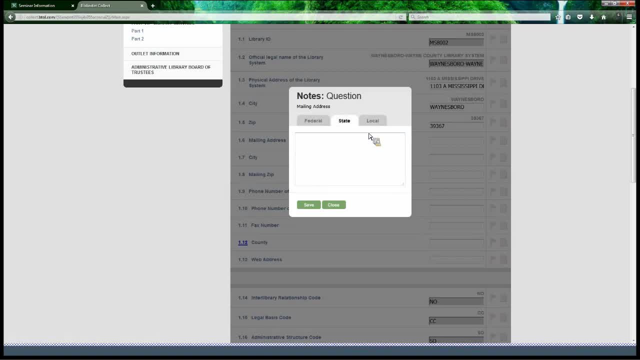 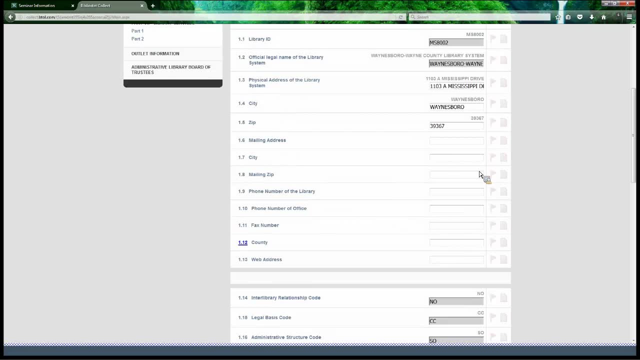 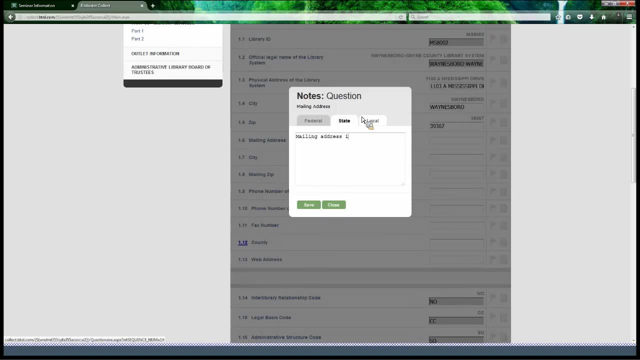 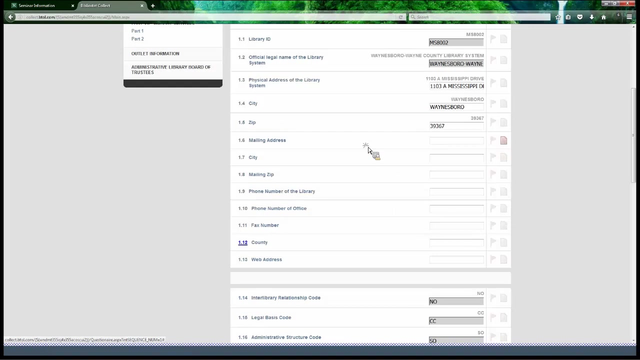 federal tab. I can help you do that. So any major notes that you might want to make would go into the state tab. So here, if I were to write a note, I would save that and then I have a note here in the file. Okay, as we. 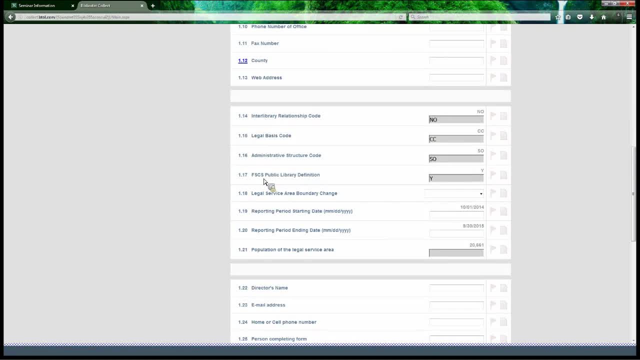 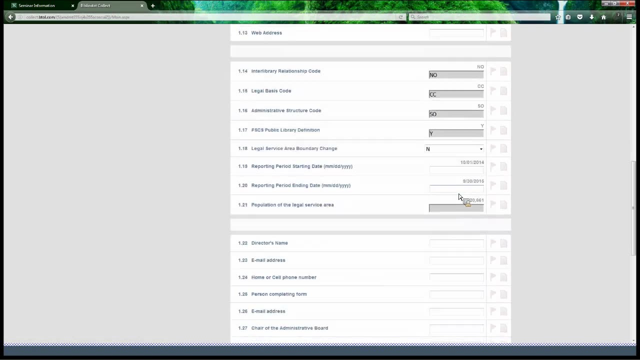 scroll down interlibrary relationship code, legal basis, admin structure and your public library definition. these are all pre-filled and locked from the previous year. You should not have had a legal service area boundary change and if you have, please let me know in a note. That would be very important for me to 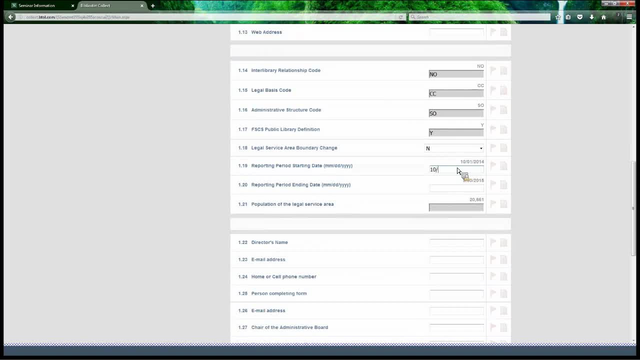 know Your reporting period starting date would be 10-01-2015 and your ending date would be last Friday, 9-30-2016. and again, I will put the population of your legal service area right in here. Okay, so this? 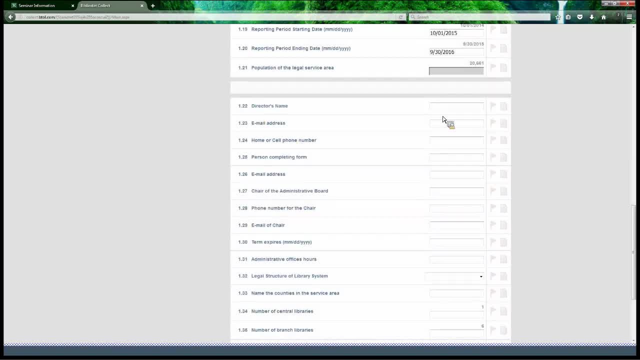 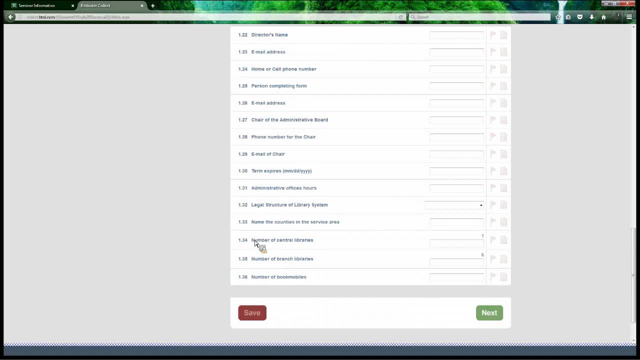 information is also going to be pre-filled, unless if there has been a change, you'll change it. otherwise you'll be fine. And then your central libraries and branch libraries. This is one area that we always have a little bit of confusion. So if you have five libraries in your system and one of them is the, 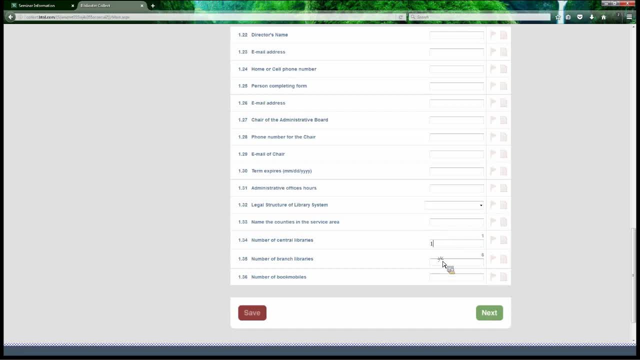 central branch, then you would put one central branch and four branch libraries. That'll have the total of five outlets. but it won't duplicate anything And once you get to the bottom of your page you will want to make sure to save If you. 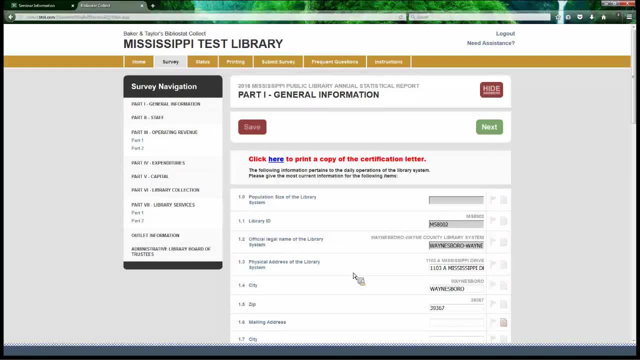 don't save, your information will not stick into this form, So I always like to save it and then scroll down just to make sure that everything looks good. If you don't save, your information will not stick into this form, So I always like to save it and then scroll down just to make sure that everything looks good. 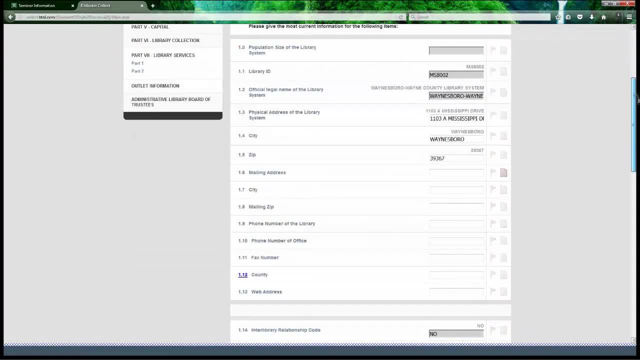 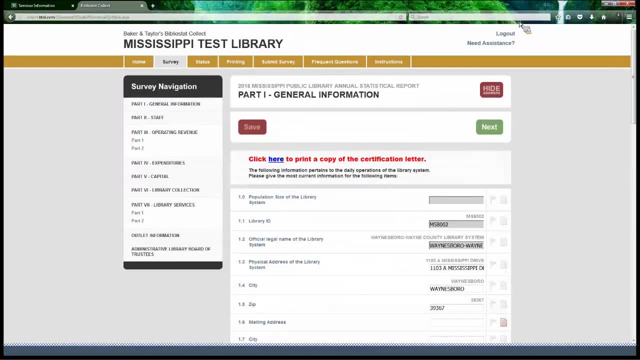 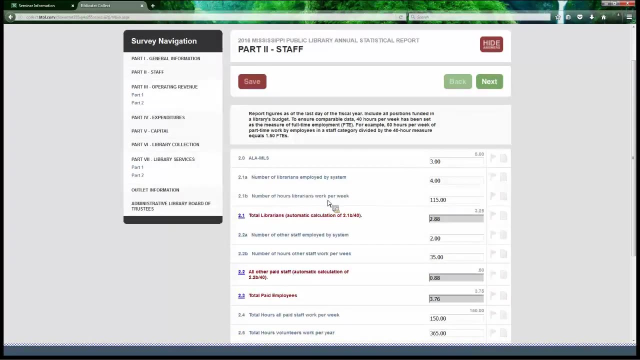 little bit like I want it to look. Okay, my information is in there, Save, and I'm going to go to the next page. There is a little bit of a change on this page. I realized that just asking you to give me your full-time employee numbers was not. 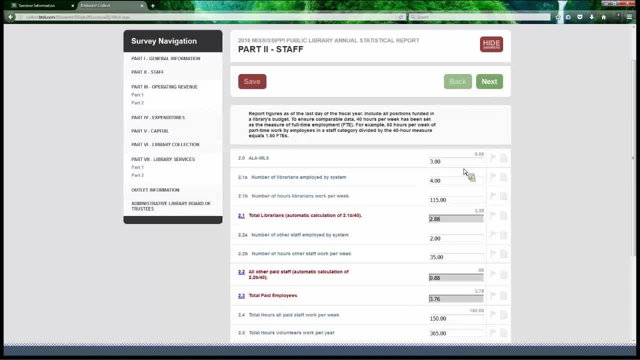 showing me how many people you had employed in your libraries. So I tried to put a little stopgap in there for that. So I'll go down these one by one. but there are a couple of changes. First I'm gonna go to the main page and then go to the 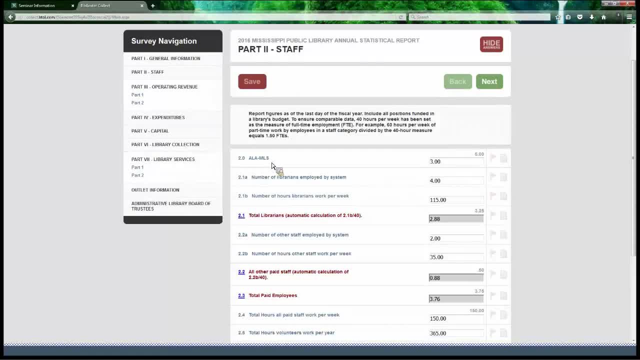 when you put in your ALA MLS employees. you don't have to worry about full-time employees here. This just is a measure of how many people that you have in your system that have the degree. So if you have three people in the system with the 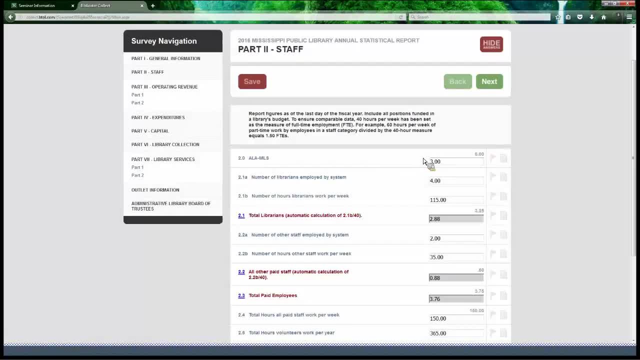 degree, no matter how many hours they work. this doesn't add in anywhere else. We're just interested in this information. It's a national question, so you'll put in how many people in your system. Notice that here. my previous year I had five people in the system. If there's a big change like that, I'd 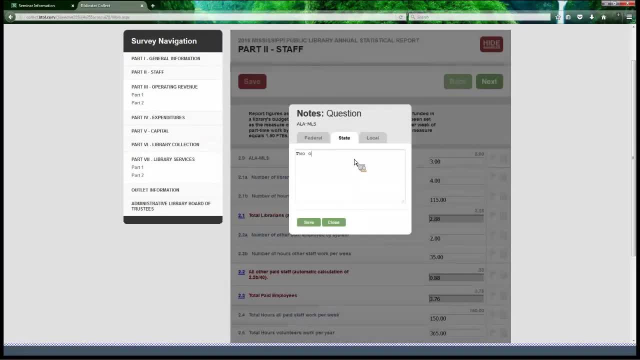 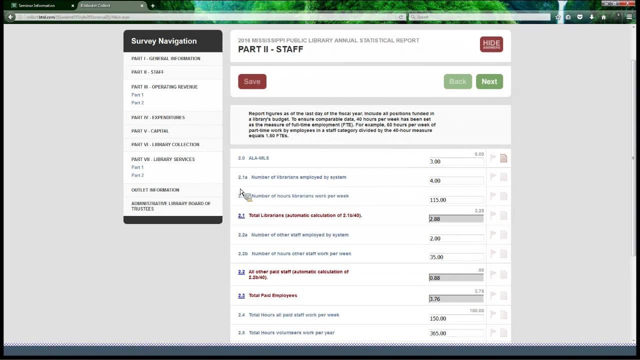 probably make a note to have our ALA librarians moved to Hawaii. You don't have to see that specifically, You can say that they moved out of your system. Okay, so for this next question, last year I had you look at the number of hours your 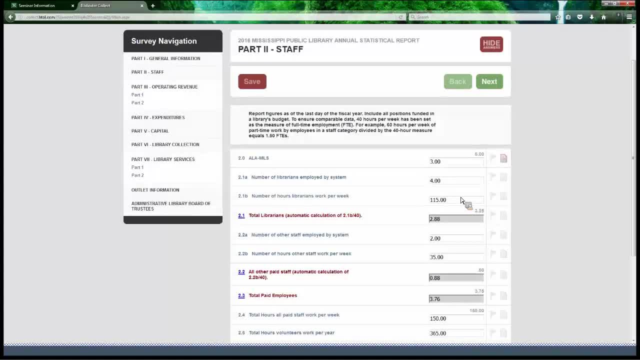 librarians worked per week and then do a little bit of math. This year we're taking a little bit of math for you So to get a sense of how many hours your a different, a different tack. so I'm going to erase out of here and just let 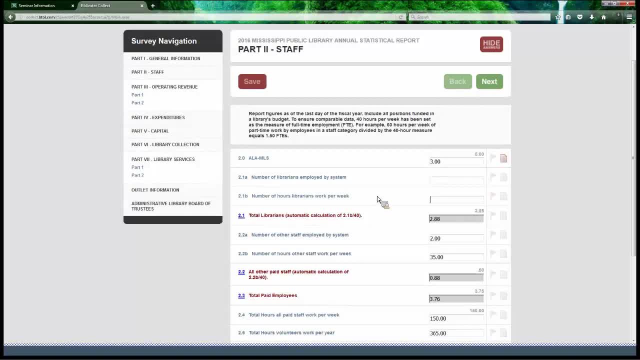 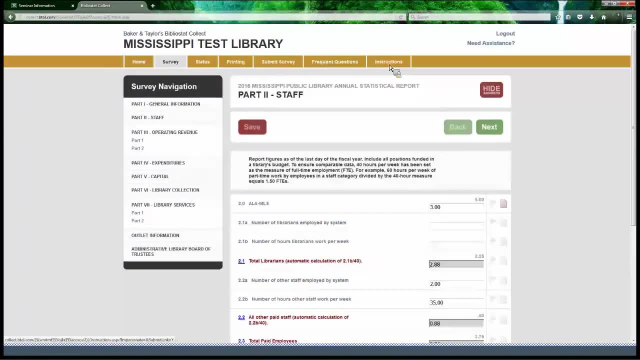 you see what we're going to do. so, according to our instructions, which you can actually print off right up here, this is going to have the way that you should answer every question. according to our instructions, I say that a librarian is anybody who does library work. circulation clerk reference. 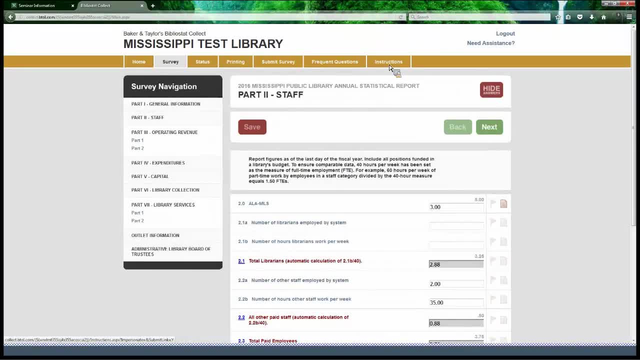 librarian, children's library and youth services, the people who are doing library work in your library, regardless of whether or not they have the degree, you should count them as librarians. think of how the public might view them when they come in and they see somebody working at the circulation desk. they 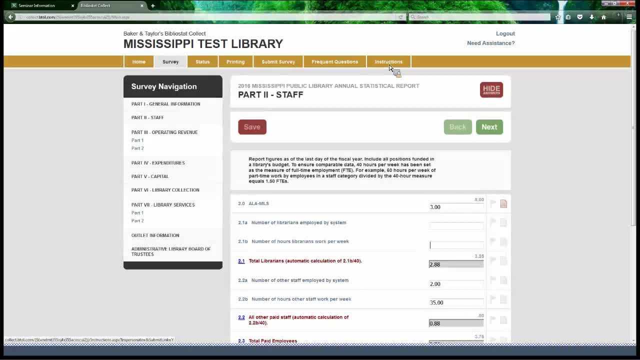 don't know if they have a degree or not, they just know that that person is able to help them find books, it's able to check them out, etc. so here, if I have three circs staff, a youth services staff, a director, that would be five people. now this is. 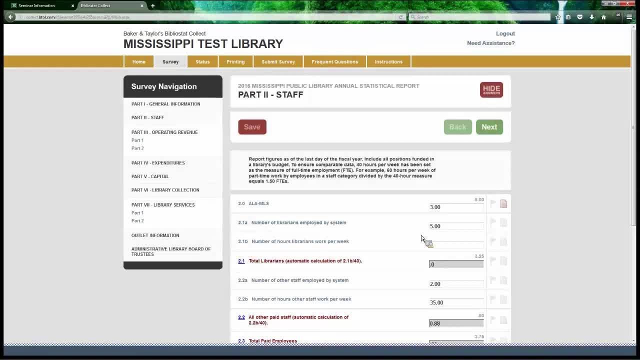 not really connected to the number of hours they work per week. so once we have this number here, we will now look at the number of hours that they work per week. so you're going to add up the total number of hours all of your librarians work. so say that that total number, including yourself. 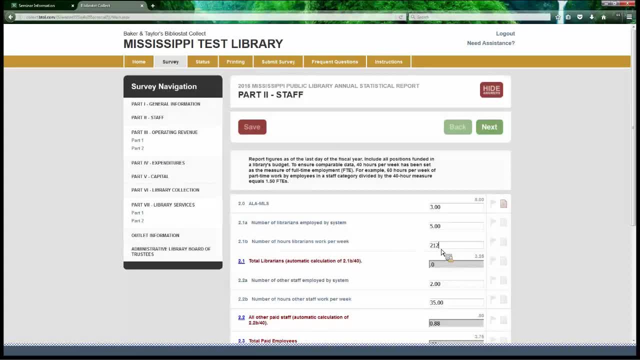 is 212 hours a week. that would mean that you have 5.3 librarians- total librarians. this is an automatic calculation of your full-time employees. does that make sense to everybody? you'll just put in their total number of hours here and then it's automatically calculated here. 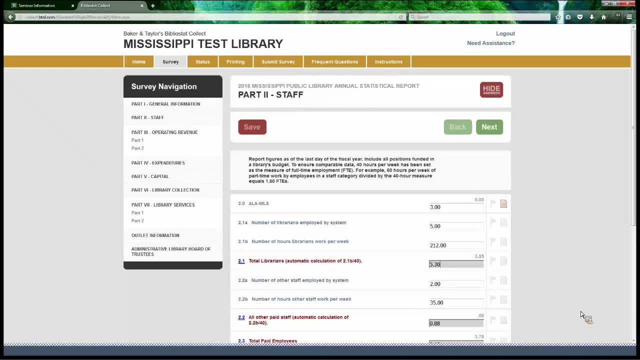 just answer in the chat box. if that is clear. ok, I'm going to say that one more time. ok, good, if you put the total number of hours that your librarians work for per week here, you just add up the total number of hours this program is going to. 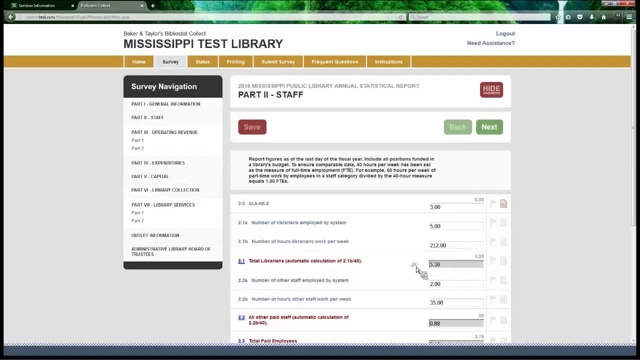 do the math for you and divide that by 40, so you'll have your. you'll just add up the total number of hours this program is going to do the math for you and divide that by 40, so you'll have your full-time employees. so next year, when I publish the tables, we'll be able to say: 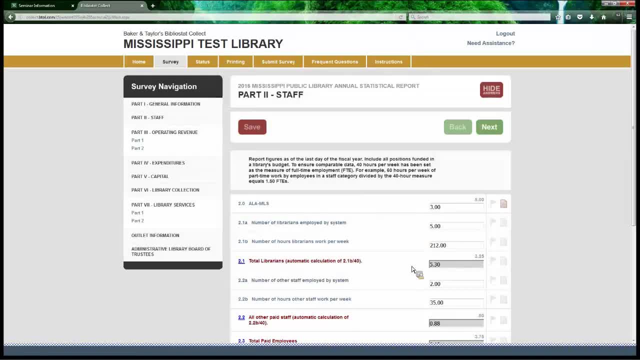 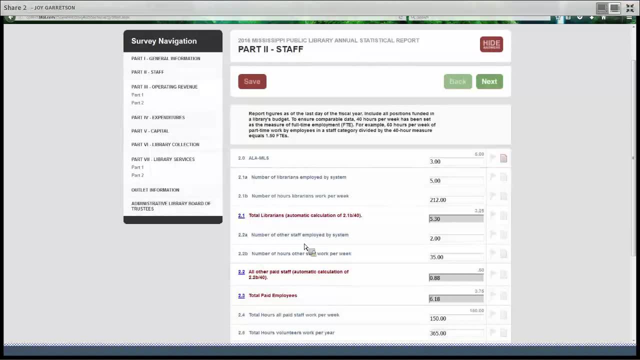 how many people work in your system and then how many full-time equivalents work in your system. okay, so going down to the other staff in your, in your system, other staff would be anybody else. you might put shelvers in this area. sometimes they just do very basic shelving work and you could put them in the other staff, unless. 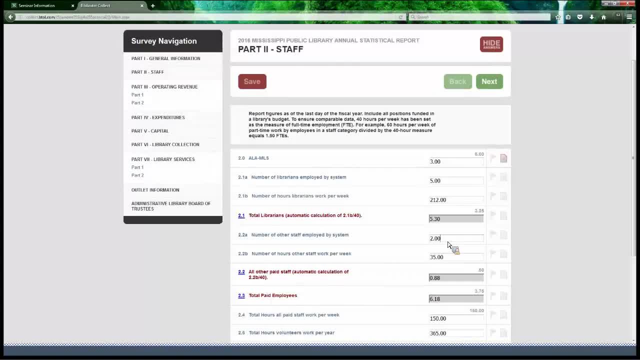 you feel like they also do librarian work, which is fine. this is kind of your call. but other staff might be a business manager, it might be a janitor. if you employ a janitor, this might be somebody that you have come in and do paperwork filing that kind of thing. so here I just put two and then I said they worked. 35. 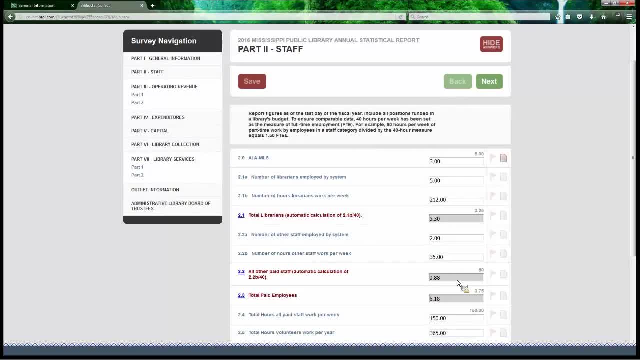 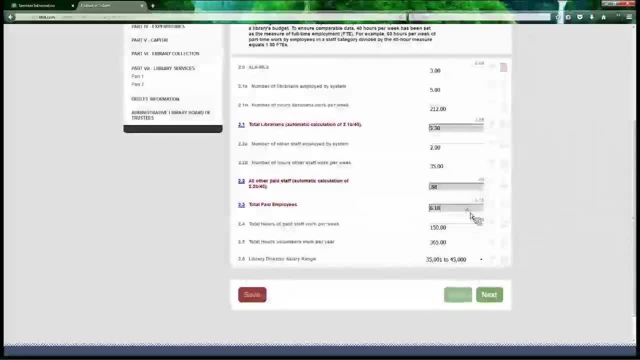 hours a week and that's going to be 0.88 full-time equivalents. okay, so now I have my total paid employees. this automatically adds up your total librarians and your other paid staff and you'll notice that. so if this were a real report, this is. 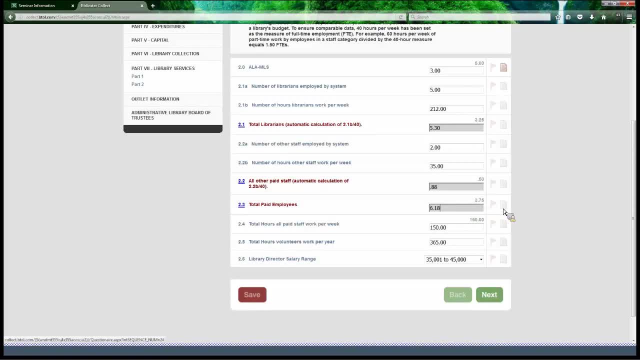 quite a difference from the previous year. so if you do have a big difference, please go ahead and make a note about it, because I will most likely have to ask you: this is? this is about a 50% difference, so I wouldn't need to go in. 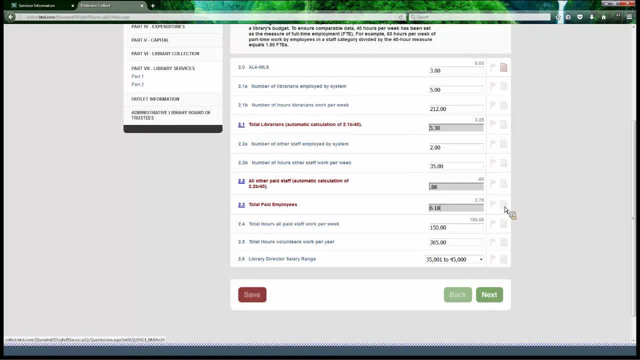 and ask you: you know what happened, what was the change at the workshop? I let everybody know that I've worked with the people who do the software so that this year, if there are any major issues with your answers, if your numbers are very different from the previous year, they'll 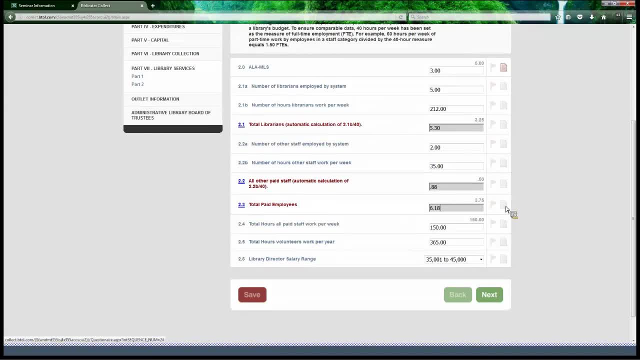 go ahead and flag all of those questions and you'll need to address them. so I'm not going to have to do quite as much follow-up as I've been doing in the past couple of years with the very small changes. so hopefully that'll be easier. 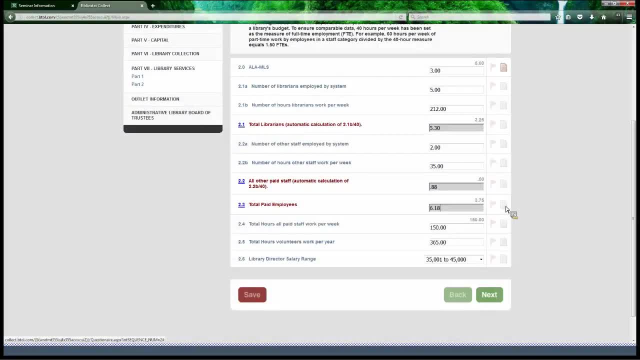 on you. you won't have to go back and answer so many follow-up questions for me, okay, so now we're going to look at the total hours our staff work per week. that's 212 plus 35, that's 247, okay, total volunteer hours. then you'll do your library director salary range and I fixed it so that now. 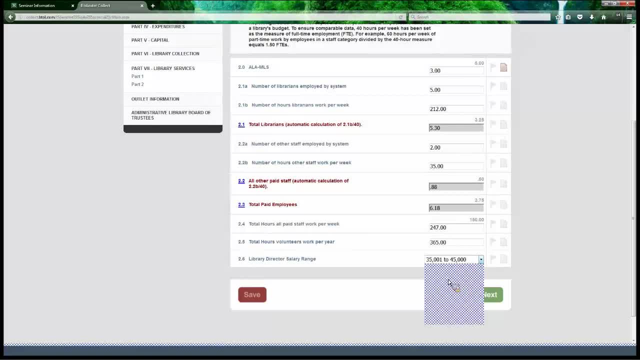 you don't have two 25,000 and two 35,000, so it's 15 to 25,000, 25,001 to 35,000, and so on. okay, once I've answered this set of questions, I'm going to push save. 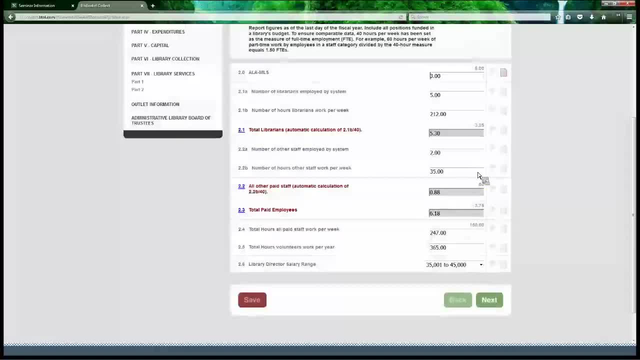 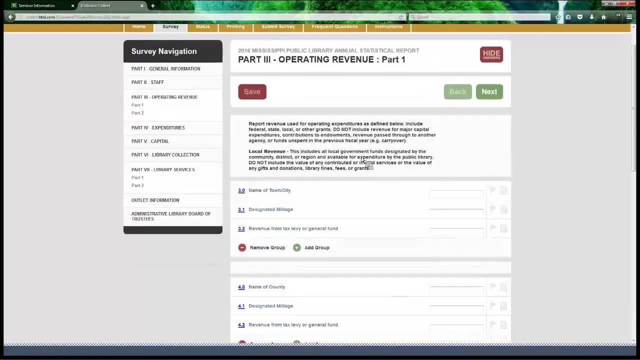 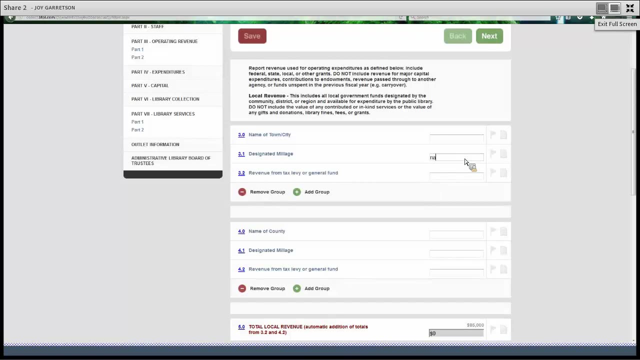 and move on. ok, this next part is your operating revenue. you will enter in your town and city income. if you don't get in millage, you just put in a. then you can put in your revenue. so the total amount of money that you get from your town or 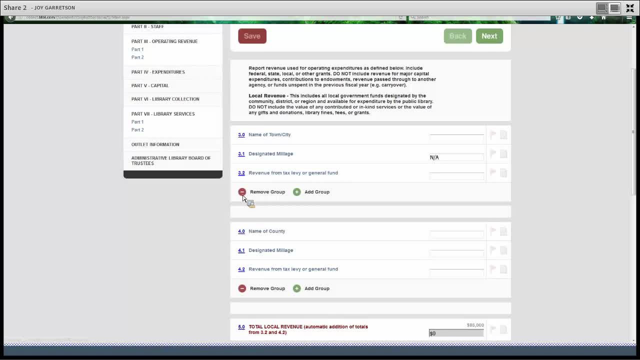 city if you need to remove or add a group. if you're getting money from a town that has a previously given you money, then you would add the group. if you town that no longer gives you money, then you can remove them. So we also have that. 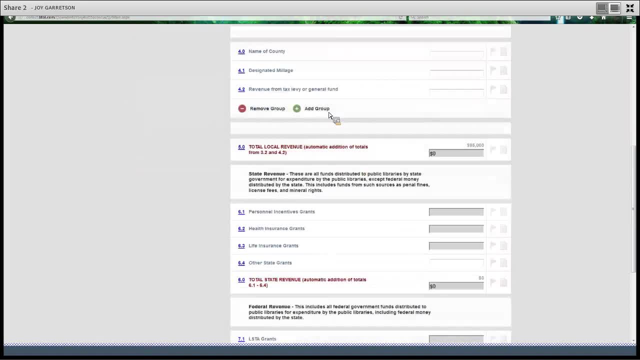 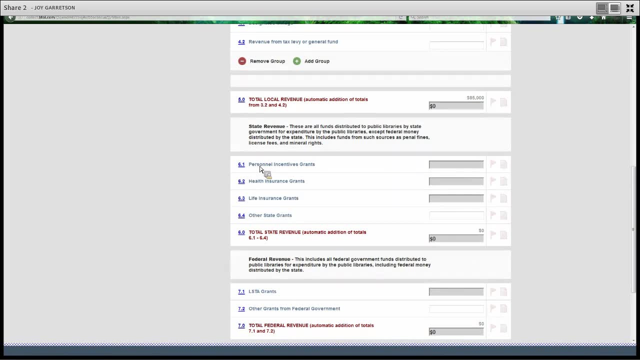 same information for your county and then that's automatically totaled here For state revenue. this year I will be entering in your personnel incentive grant numbers, your health insurance numbers and your life insurance numbers for you. You can check back on those. once I've got those in, I'll start putting. 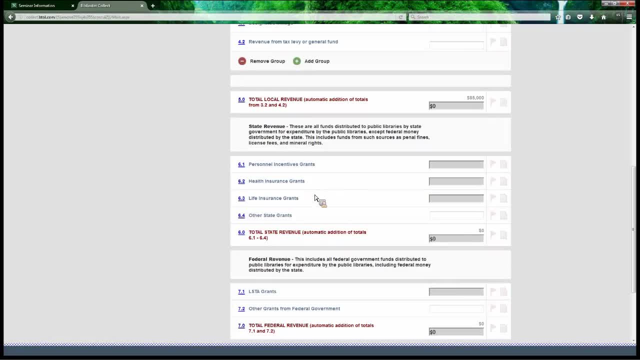 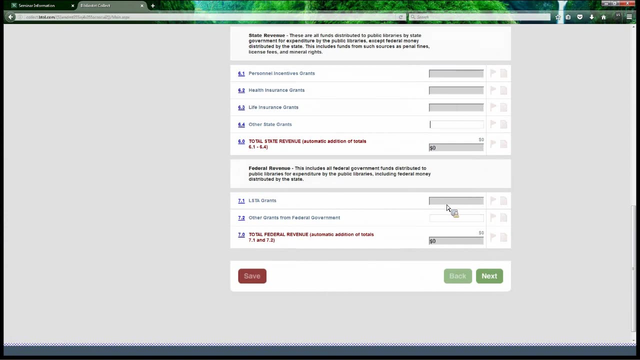 those in as soon as David gives me the reports. So if there are any discrepancies or questions that you have about them, just let me know. If you get any other state grants, you'll enter that in yourself. And this is the same with federal revenue. I will be entering in the LSTA grants the amount of 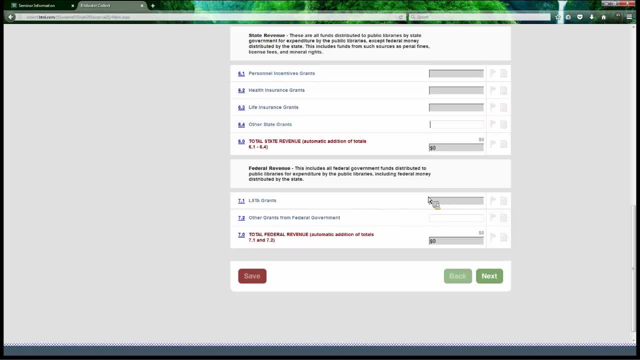 reimbursements that you asked for from David. So that will go right here and this all is going to come straight from those reports that you get every year, so hopefully this will not be a surprise to you. If there is an issue, like I said, just let me know. Other state grant. 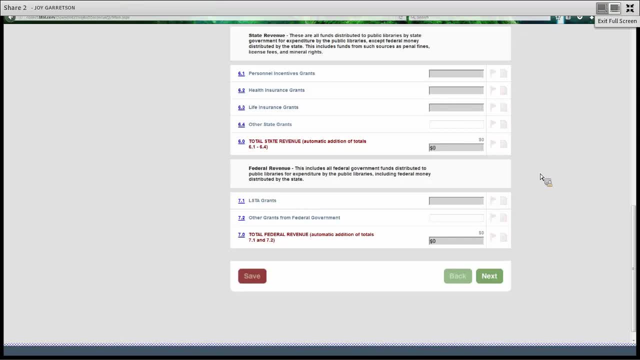 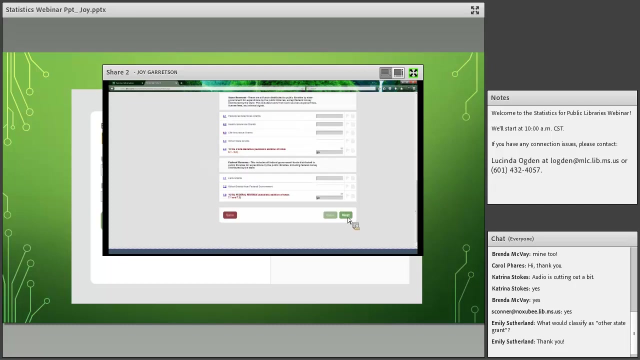 so maybe you got money from the Mississippi Arts Council, or maybe you got money from the Humanities Council- or actually I'm not sure the Humanities Council would count as a state grant- but any other money you get not from us. yeah, Okay, once you have this information, you will save it and go to the next page And 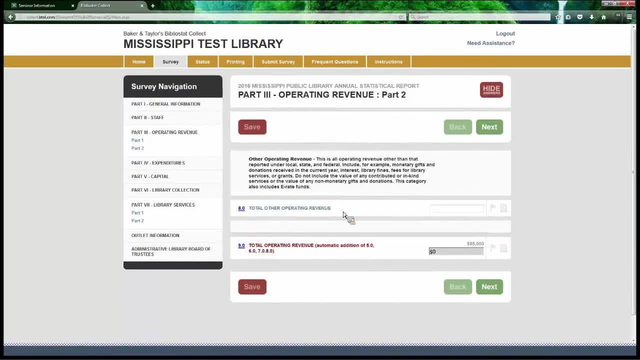 here's where other other total, other operating revenue goes. This category does also include your E-rate funds, So you would enter in that information here. This is going to be your monetary gifts and donations, interest, library fines, fees for library services, grants, etc. That's all going to go here. 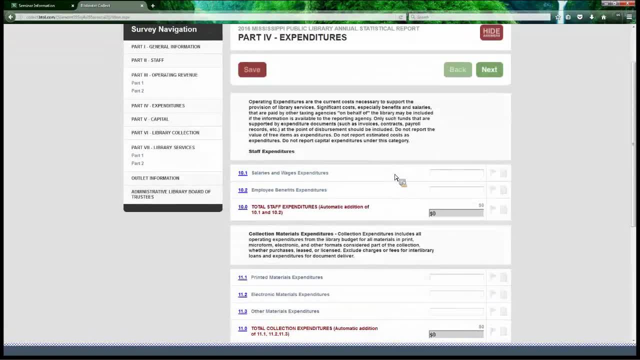 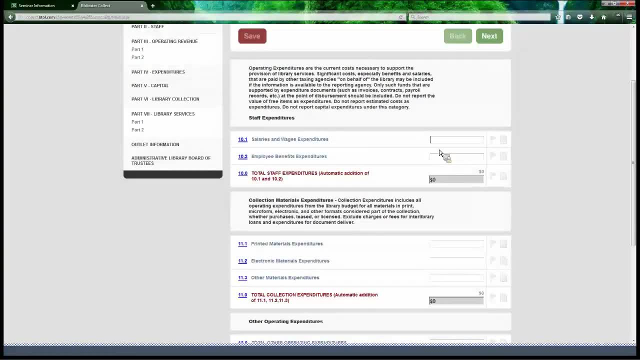 And your expenditures Again, if there are any large changes- and there might be this year, because we all know that we have lost a good deal of state funding. So if there are changes here, just make a note And then we'll get to our collection. 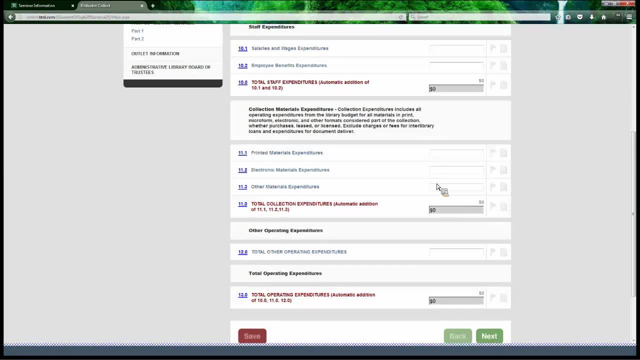 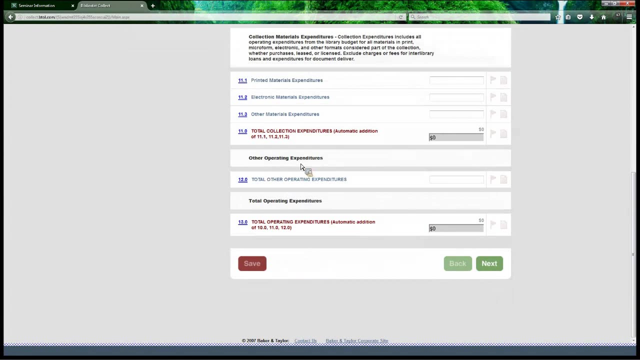 materials expenditures. A lot of times there are some kind of major changes. if you move a significant portion of your budget from printed materials to electronic materials, Again, just make that note in this little section And we have total other operating expenditures. and if you don't have your E-rate funds, Here we go. 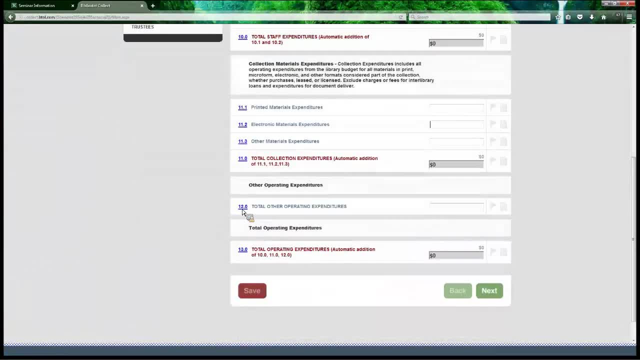 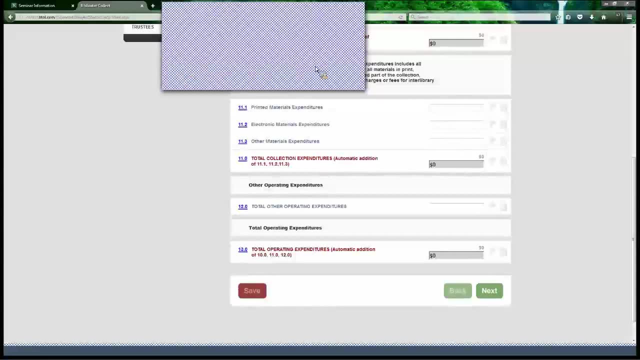 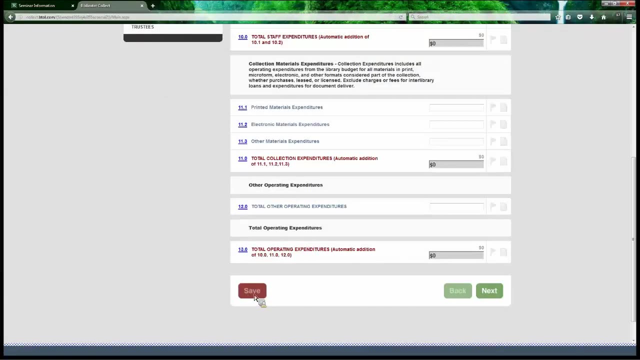 instructions printed out. You can also click on this button and it will give you the way to answer the question. So this is all expenditures other than those really reported for staff and collections, And we'll save that and go to the next page. I'm flying through this early part, so if you have any questions, 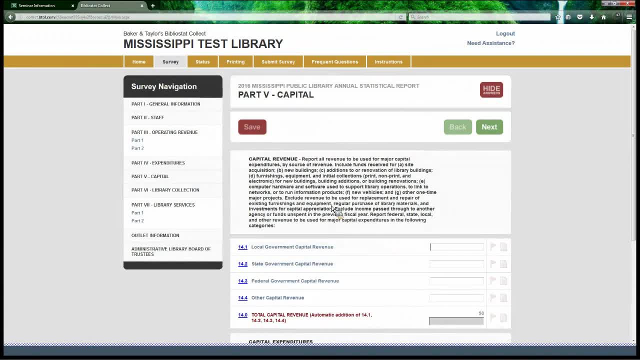 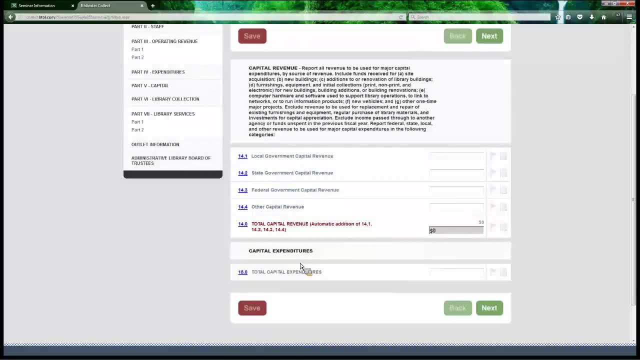 please stop me. Okay, here we have our capital revenue. One thing I wanted to say is that if you do spend some capital money from a leftover fund that you had in previous years, but you don't have any revenue, so you weren't given any new. 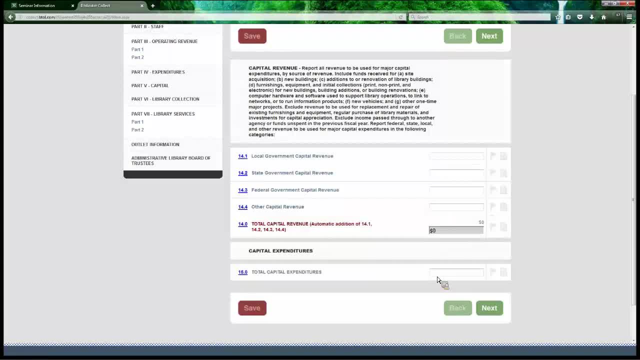 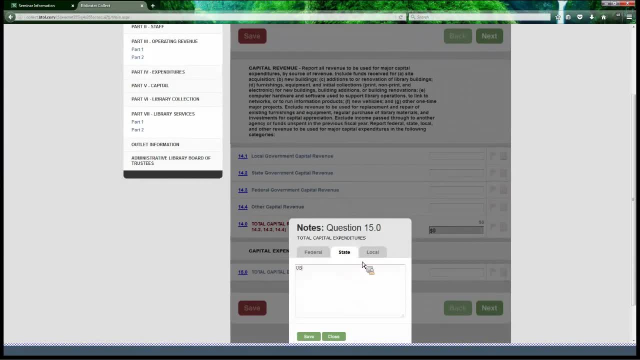 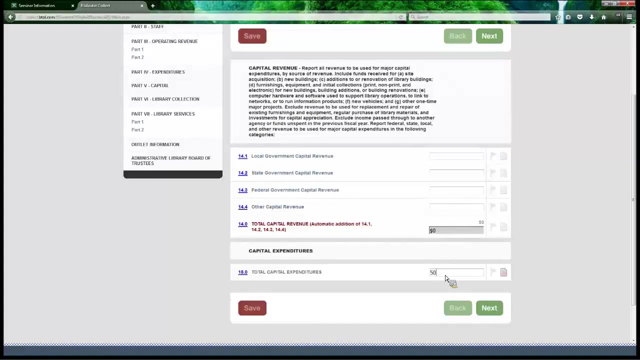 capital money. but you were able to spend some old capital money that you've got. just make a note to that effect: used Is that you save this? So say you spend $50,000 on some part of your building. you could just make that note there And also here. if you don't get any revenue you will put. 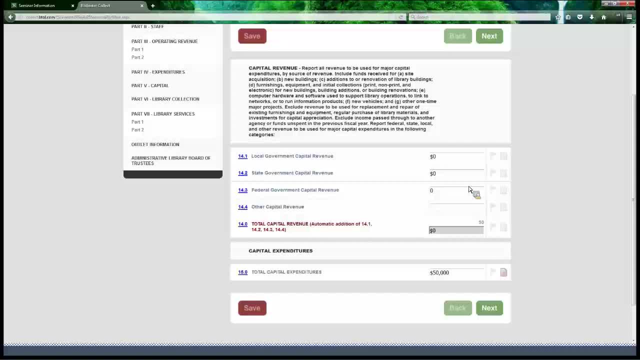 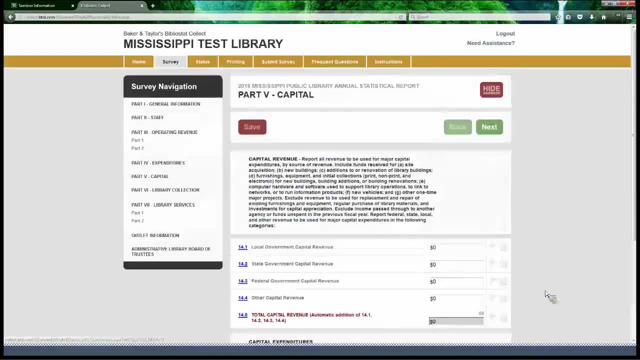 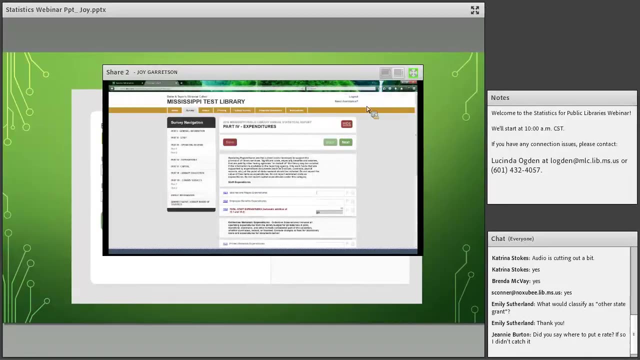 in zero, not in A. Okay, save that. Oh, E-rate. I'm sorry, Janie, that's going to be back. If you don't get that one in zero, that's going to be back, And then somebody will take your total. 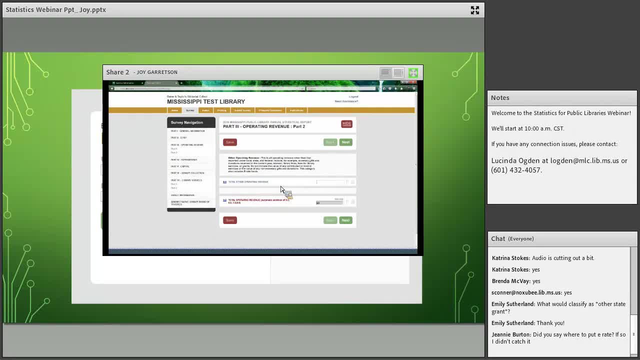 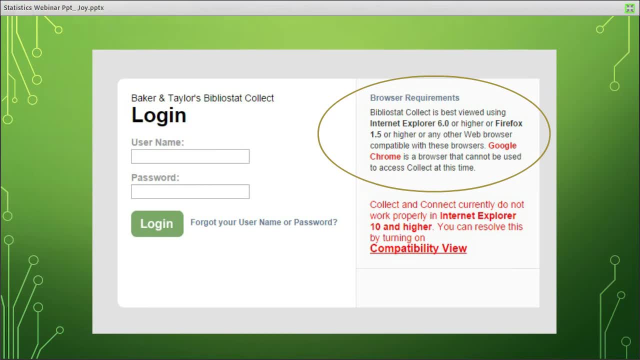 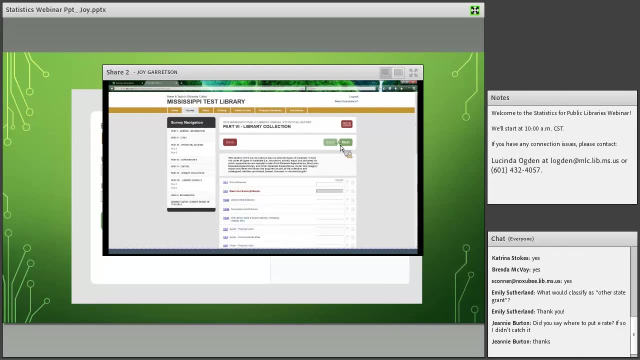 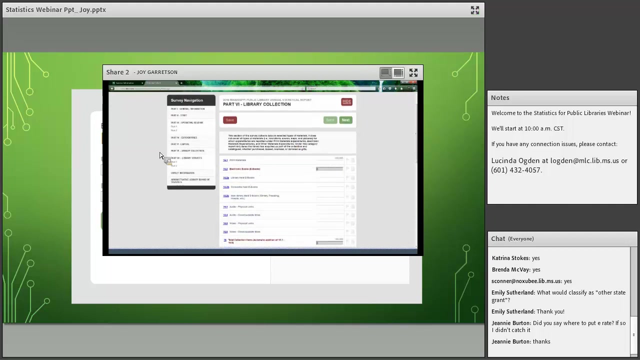 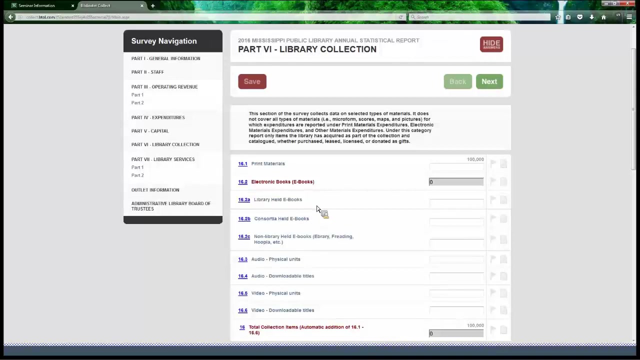 operating revenue In total. other operating revenue: Okay, Okay, so we are gonna go forward. Okay, good, okay, number of items that are in your collection do not just put. do not just put the new items that you added this year. okay, so, any print materials or 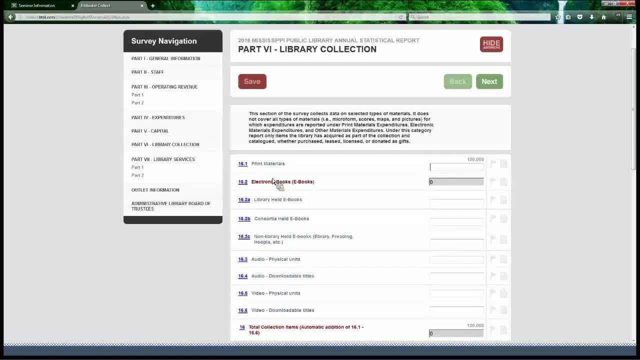 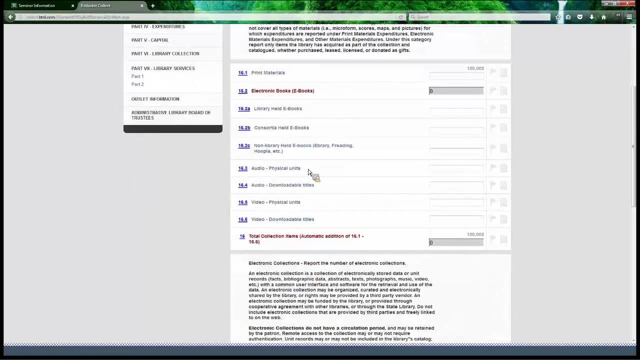 physical items that you have. that would be print and I would say I don't have a place to put cake pans. go ahead, if you have cake pans or a strange thing that is not print. I need to make an other category, but for now you can put it in. 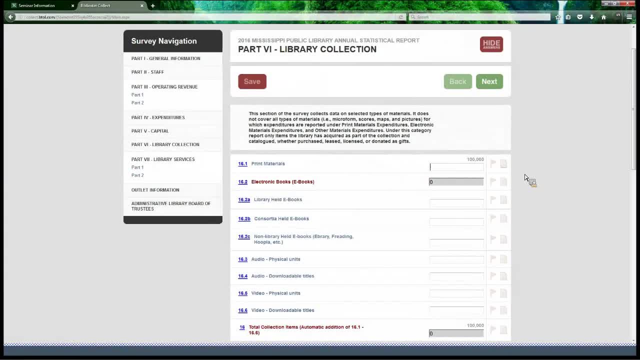 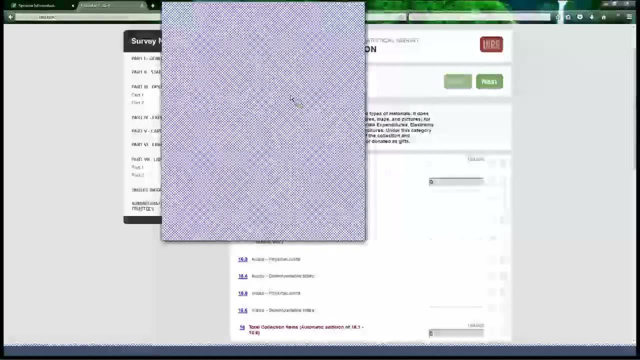 the print section. okay then for your electric electronic books. we discussed this at the workshop. if you have ebooks from access 360, overdrive, that kind of thing, I have a big note here about how to answer all of this if you have just regular ebooks that are in your permanent collection. 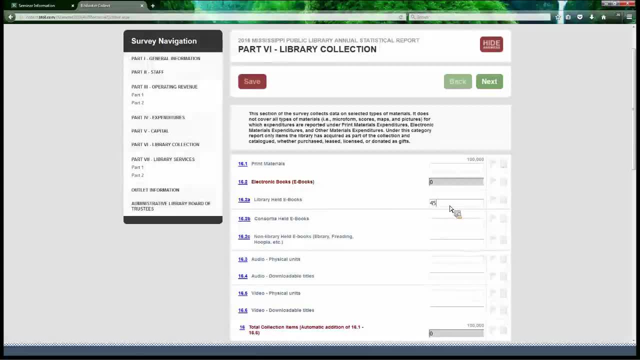 so if you have regular ebooks that are in your permanent collection. so if you have, so perhaps you have 450 ebooks in your in overdrive. you'll put that answer here. if you are part of a consortium, you can put your number of ebooks that you have. 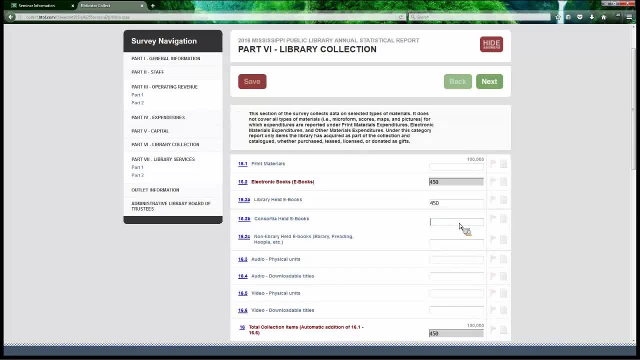 in your consortium. here some people, there are a couple of library systems that are in consortiums and if you have a consortia and if you have a question, just let me know I can help you out there. then, finally, your non library held ebooks. this would be items from ebrary Frieding, hoopla. 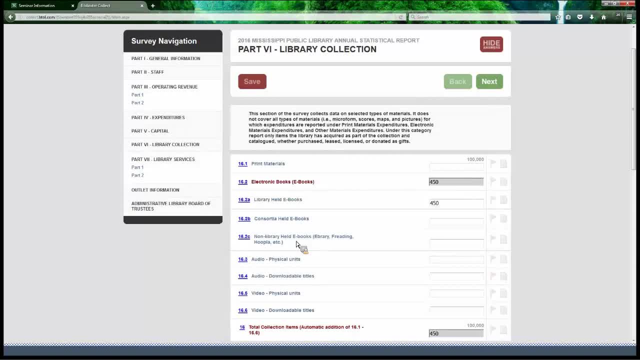 and so on. here, what I'm asking that you do is you're gonna count one use as one item. so if one person checks out a Frieding book from you, then that would be one item in your collection. I've seen several Frieding reports and you get at. 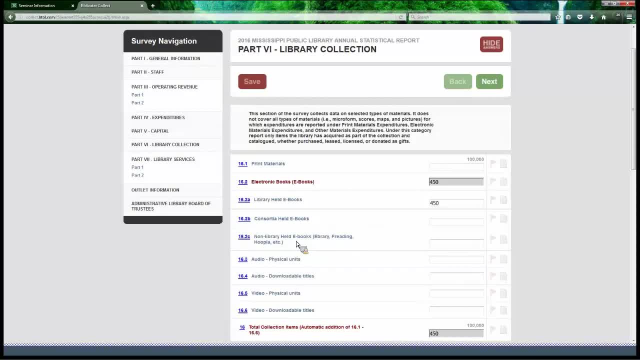 the end of the month. however many checkouts you've gotten, you would count that as the number of books in your collection. does that make sense? this one is a little bit difficult. some people want to say: well, Freeding has got 40,000 books in it, so I have 40,000 items in my 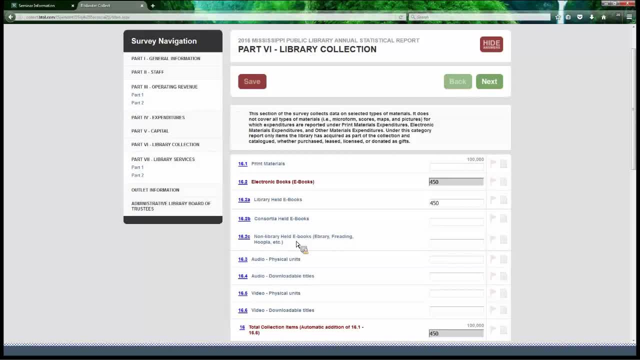 collection and while that would be great to be able to say, I don't think it's an accurate representation of what you actually have in your collection and I feel like it's more manageable to say we had 360 people access Freeding this year from our website, so you could count those 360 books here in this slot and 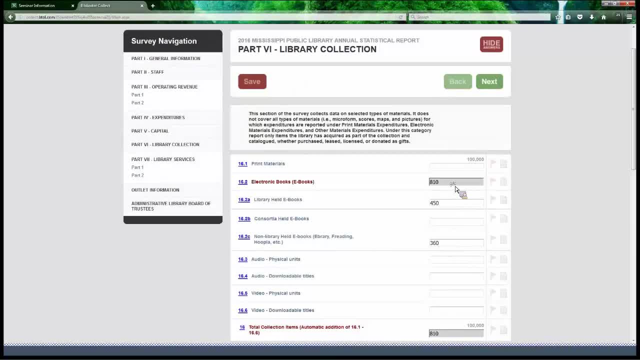 that's going to be automatically added up for you in in this electronic books area up here. are there any questions about that? if you aren't aware of the consortia ebook information here, that means you're not in one, so you're fine. okay, so for audio physical units, this is the same audio downloadable titles, video. 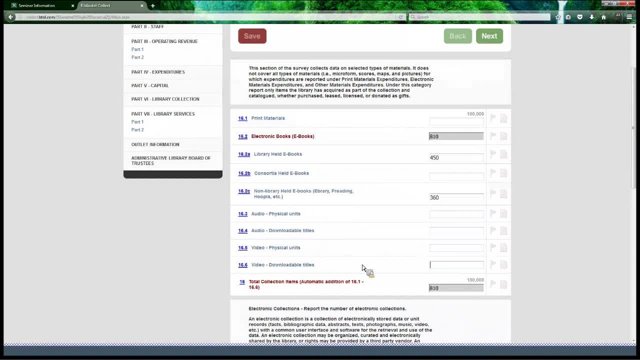 physical units and video downloadable titles. none of that has changed from the previous year and I'll put in the link in the description so you'll see down here your total collection items. it adds the 16.1 together: 16.2, 3, 4, 5 and 6, so these three little numbers. 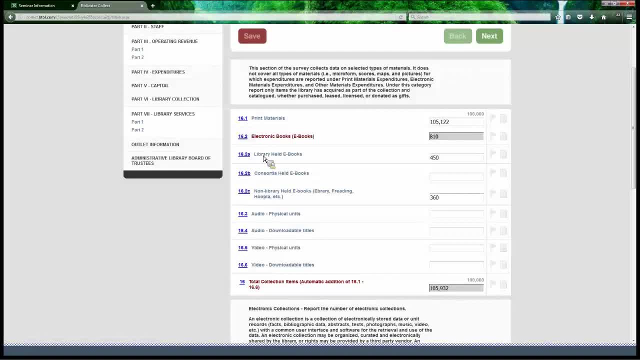 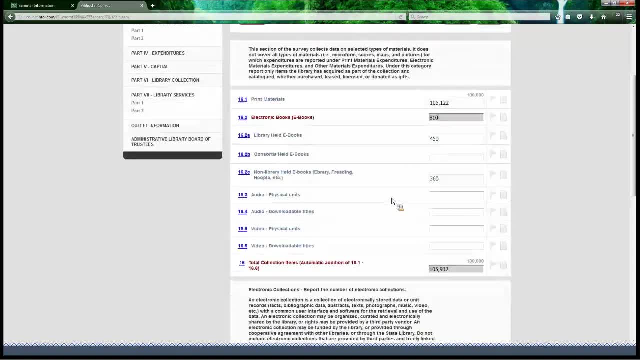 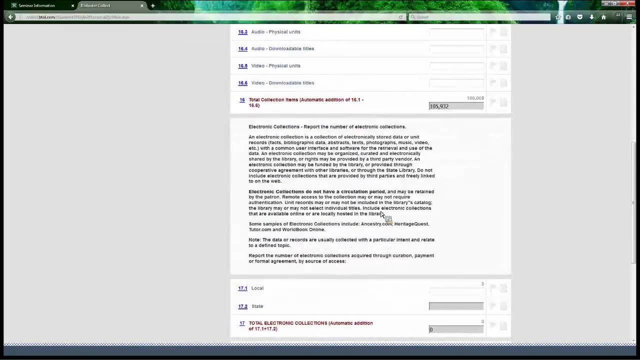 here 2, a, B and C are all. they're all subsets of 16.2. so they're, they're all automatically calculated into 16.2. okay, so, scrolling down, we're going to look at electronic collections. this is another word for database. we decided to change from database to electronic. 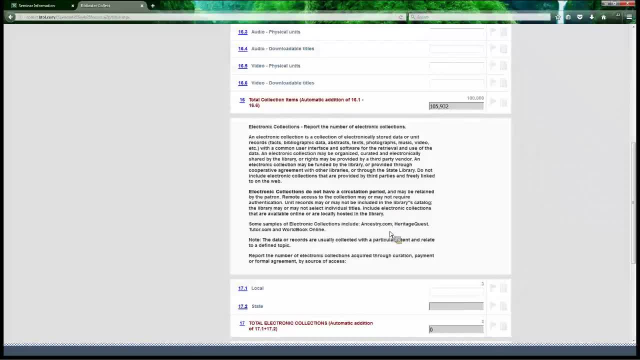 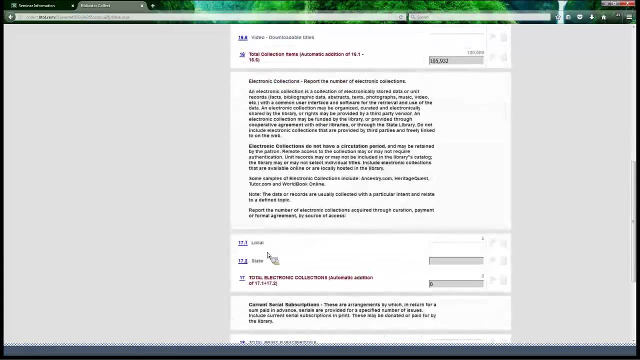 collections because- and we thought that more accurately showed what this is- so if you have heritage quests or if you have mango languages, that may not be what we would traditionally consider a database, but it definitely is an electronic collection. so here in seventeen, point one, we have heritage books and there is the And 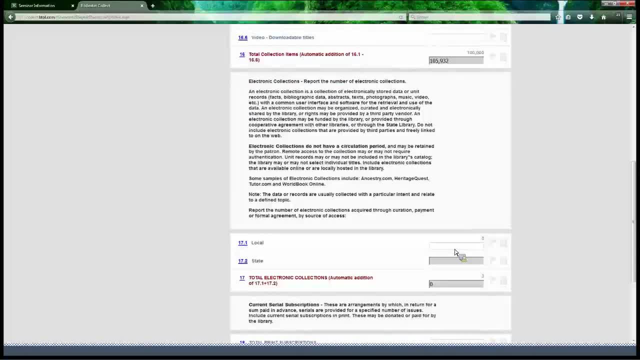 so we can see each of the collections and we can go through all of them and get together during. together we can find training in the course and so using our collection is prettier and paper speed. so all these colors and data, Sodom, and you're going to put in the number of local databases that you have, You may. 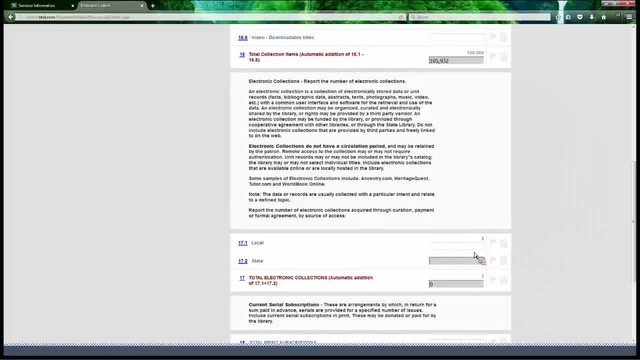 want to list them out here. I have a list that we're going to look at in just a bit of the way to count your databases- and I might not have one that you've got- I did go through everybody's website and pull information about all the databases. 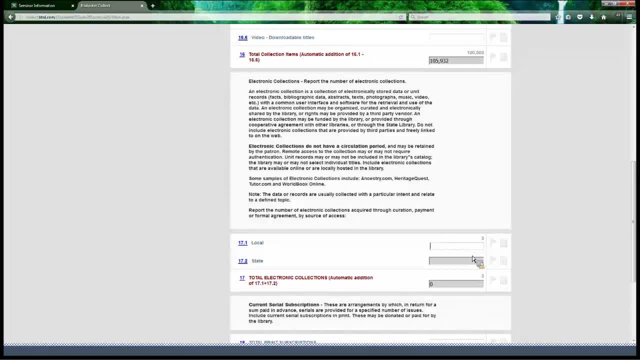 that I could find there. You might want to go ahead and just list out the databases that you have at your library system so that if there are any problems counting the usage of them- which we'll talk about in a bit- we can address those. I'm going to pre-fill state databases for you, or state. 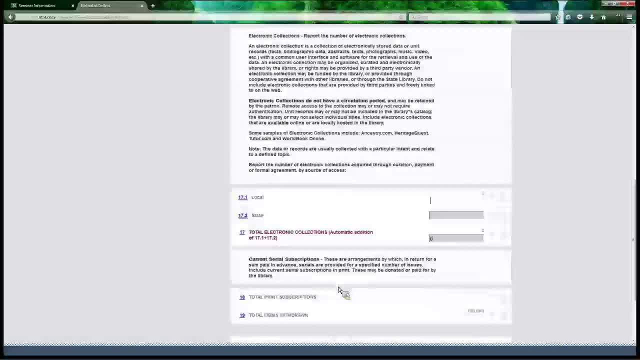 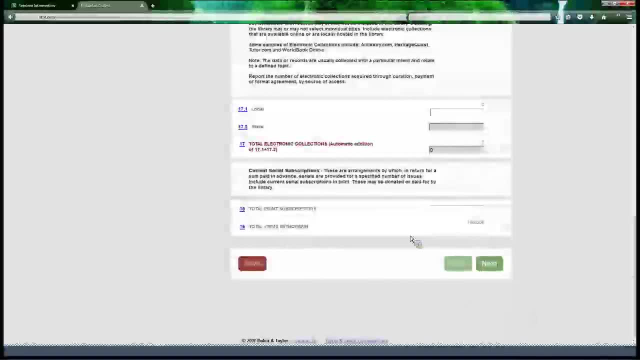 electronic collections. for you, That number has changed a little bit since this summer. Then we have our total print subscriptions and our total items withdrawn. For those of you who have Zinio, that is actually a database. That's not going to be something that you put in your collection. 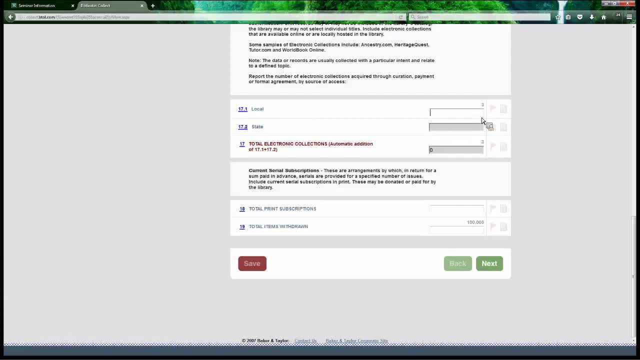 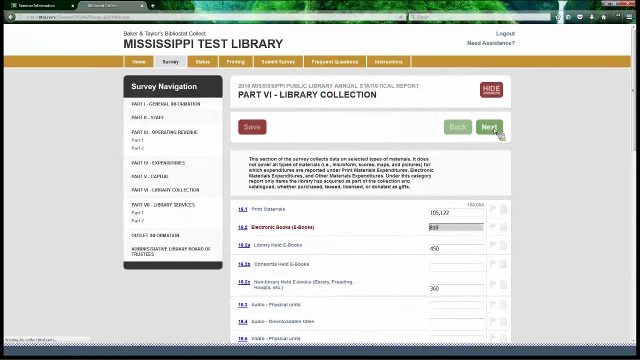 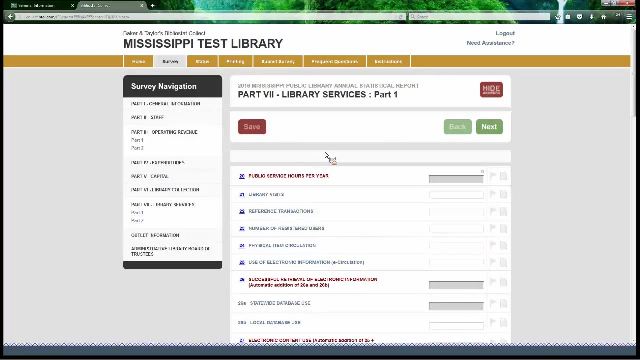 You would count that up here. Zinio is the database that gives people access to those great periodicals. You'll save this information and we'll move right on. In this next section. we have public service hours per year. Right, there is number 20.. This is going to be automatically. 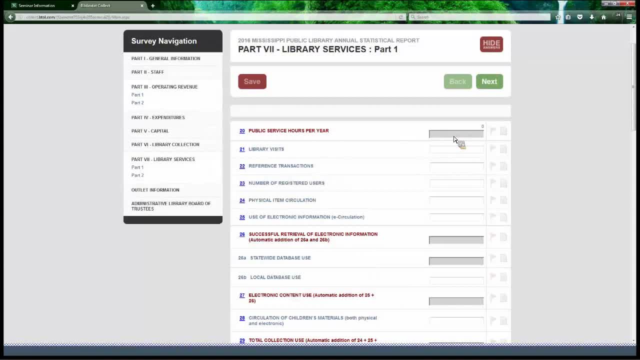 calculated from the number of hours that you report in your outlet records. You will not be able to put a number in here, but your outlet records are going to automatically populate this field. Then we'll do library visits reference transactions For those of you who have issues with your reference. 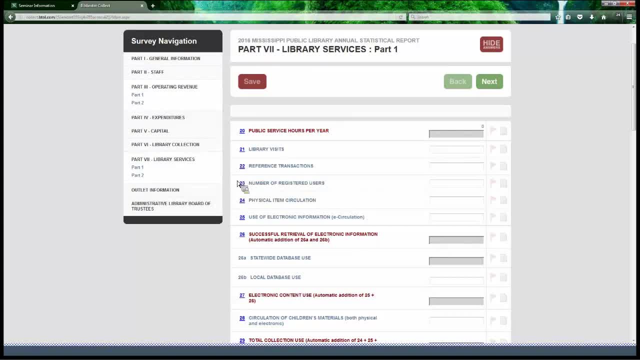 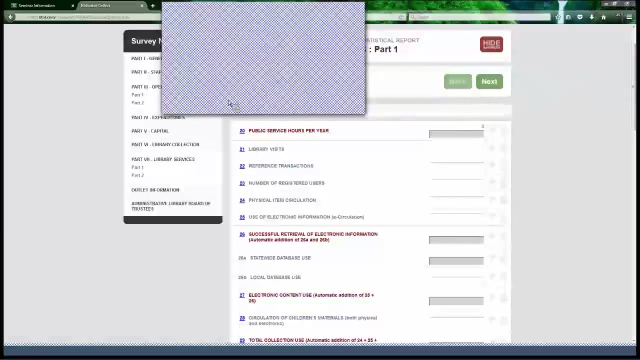 transactions and how to count them. I do have a helpful worksheet that you'll be able to download at the end of this webinar: Your number of registered users. In this number we generally suggest that you update it. You want to purge your files. within the past three years, I've had a couple of 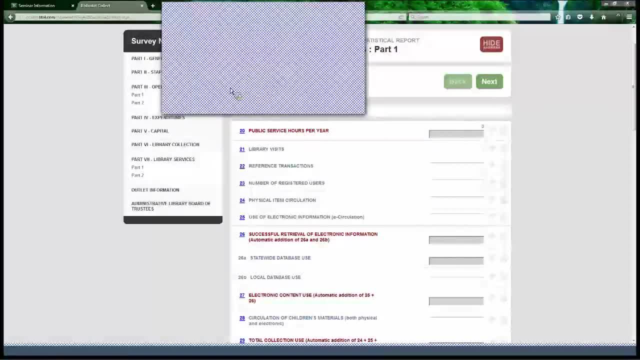 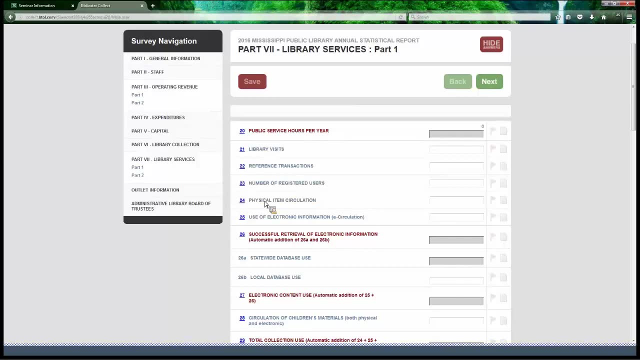 questions about what to do when you have somebody who's got just a huge amount of fines on their files. I can advise you about that individually if you have a question. Number 24 is a little bit different from what we've seen in the past. Physical item circulation. 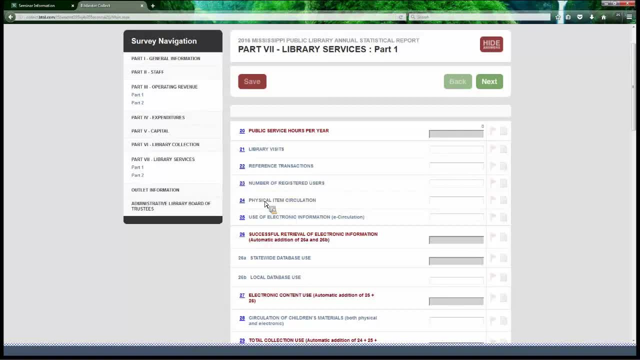 Used to be total circulation. We felt that it would be more representative of your collection to say physical item circulation, because it kind of clarifies that these items are physical items that people take out of your library. This could include books in print, it could include cake pans, it could include DVDs, it could include CDs. 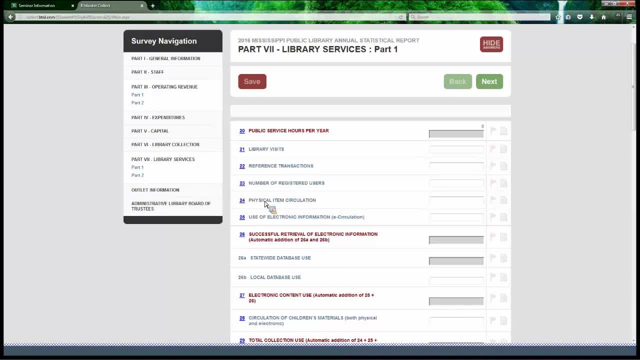 it audio books and Playaways. It's all the physical items that people can take out of your library. So if your physical item circulation, it might be- I don't know- 158,000.. We'll see in just a minute. These are all going to populate down here, So 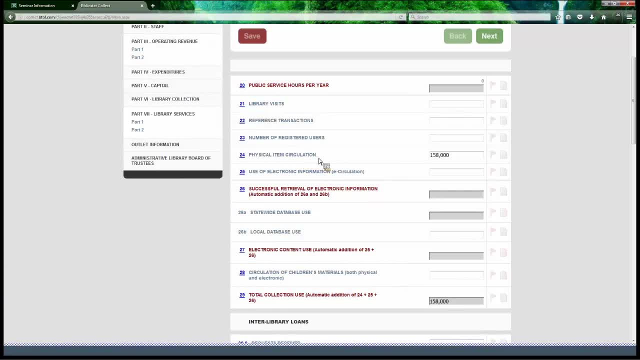 that's one new thing and that's the really. it's really just a sort of a renaming of the element. This way, we know where to put that weird stuff that we lend, like cake pans. The next one is going to be your use of electronic. 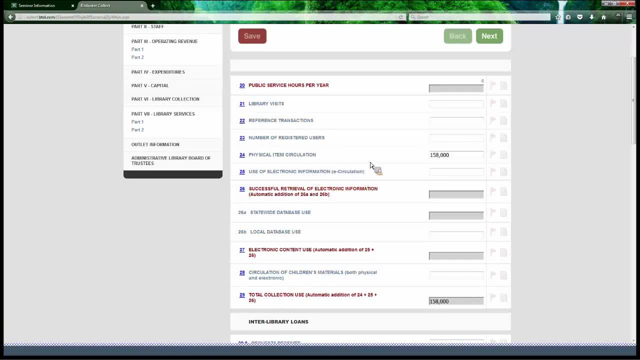 information. This is e-circulation. This is your ebooks. So this is where you add in however many reading checkouts you had and however many regular ebook checkouts you had. So I think on the previous page I said maybe you had 360. 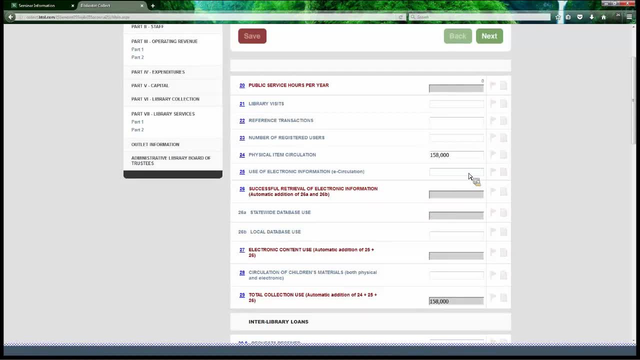 reading checkouts. So you would add that if you also have access 360 or Overdrive, You would add that together with those. Say you don't have access 360 or Overdrive, then you would just put in your reading number here. If you don't give access to any ebooks, then you could just 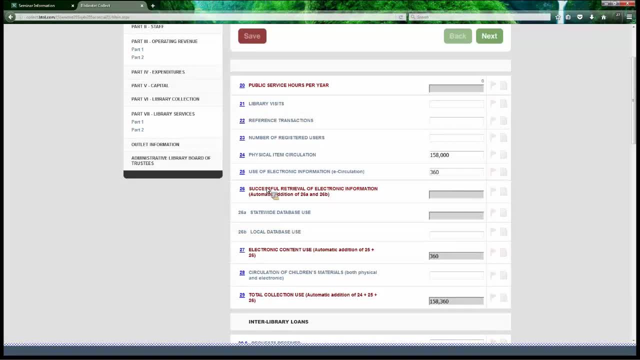 put zero Okay. and this next one is a new one and it is a little tricky, So I will just ease your minds now and say it's okay if it's not perfect this year. We have about three years to get this one right. We are all going to be working. 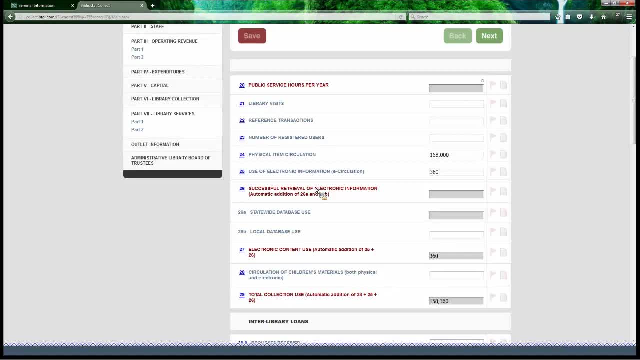 together on this and I'm actually going to jump to the PowerPoint in a second to discuss it. This is the successful retrieval of electronic information. This is basically your database use. So this is a good way for us to show how your databases and how your electronic collections are being used in your library system. 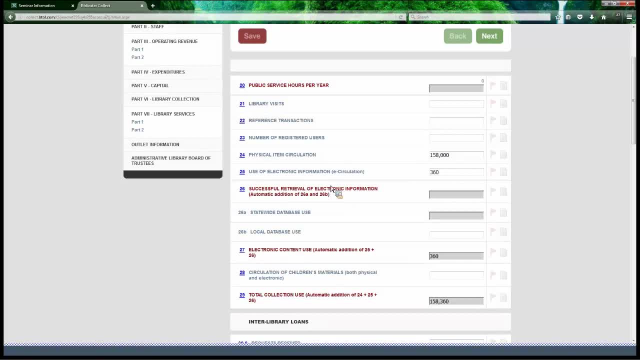 Previously we have not had a standardized way to count. you know, if you have a World Book and Mango Languages at your library, we haven't had a great way to show that to your, to your boards of students. So it's a great way to show that to your boards of students. 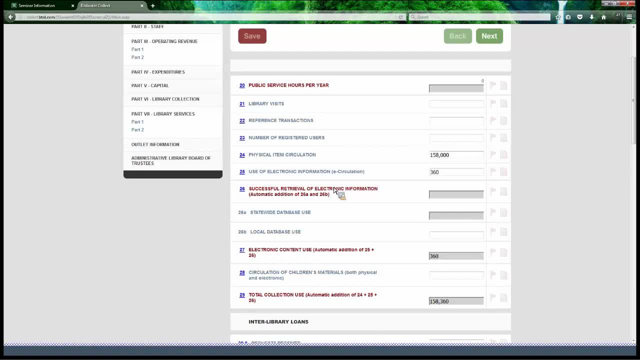 supervisors, or to your board or to your community. So this is an attempt to make this more easy to find. It's to help us standardize this question. So there are two elements here: The statewide database use. this would be your use of Magnolia. 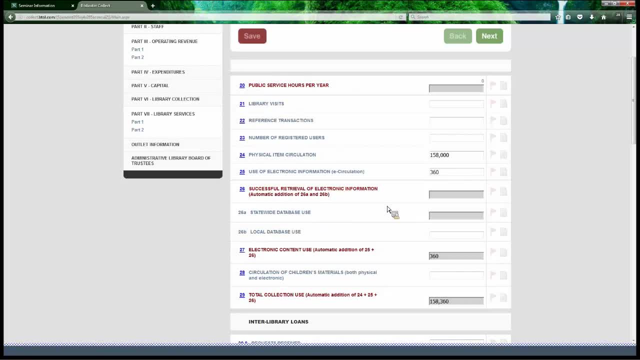 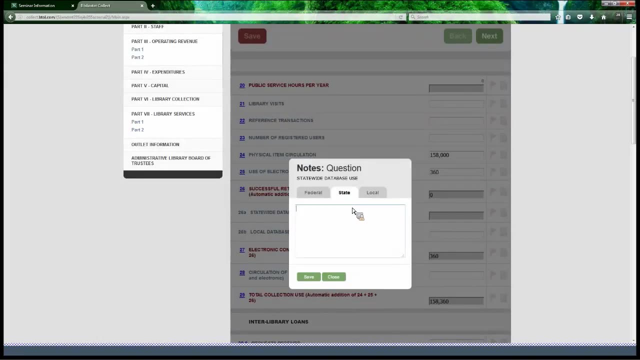 your use of Learning Express, your use of First Search, the other databases that the Library Commission provides for you, and I will populate this for you. What I'll also do is come in here and write for you. I'll say Magnolia, and I'll have: 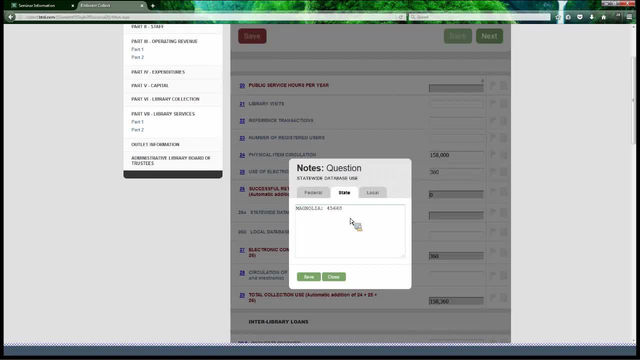 your number there, Then I'll have Learning Express and that number and I'll also have, if you use First Search, any of our other databases that you use on your library level. I'll put those numbers in here so you can see how they. 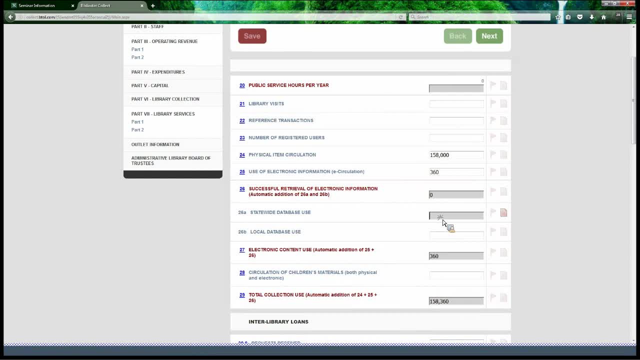 break down, But this number will be populated by me And then your local database use is what you will be populating yourself, And I'm going to pop back over to our PowerPoint for just a moment to show you how that works after I save this. 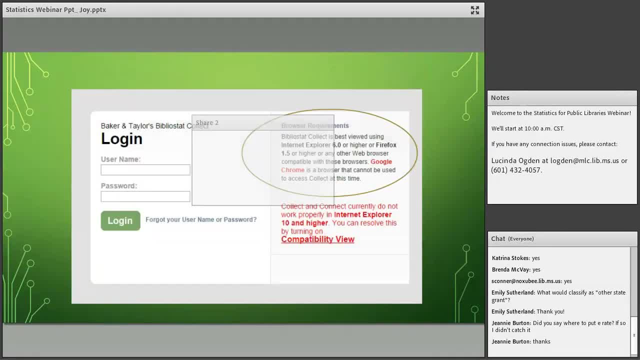 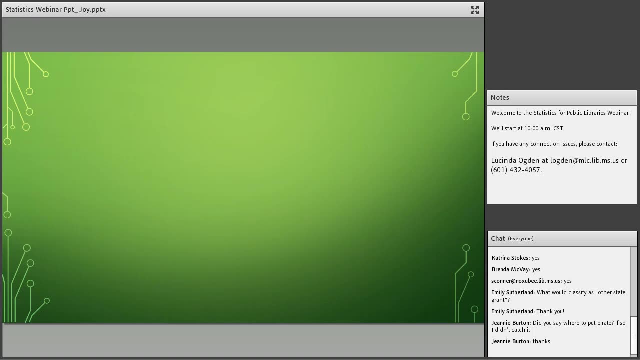 Okay, Let me see. it'll take me just a moment. Okay, So you see here that we have our most common locally purchased databases: Ancestry, Heritage, Quest, Rocket and Mango Languages, Cypress, resume, the Gale databases, World Book Online, Xenio and the ProQuest databases are the most. 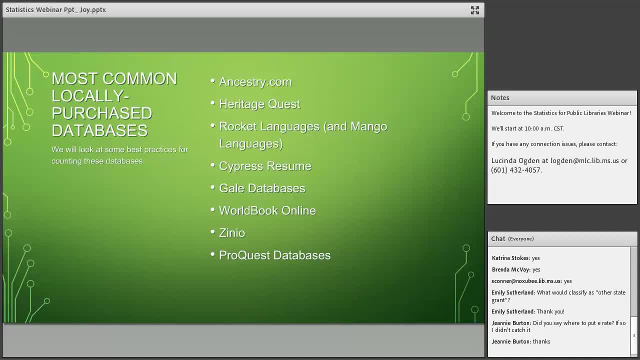 commonly used. So I'm going to show you how to count those, and then I'll also show you a spreadsheet that I've made for how to count them, And then I'm going to you a spreadsheet that I've made for how to count some of the other ones, and 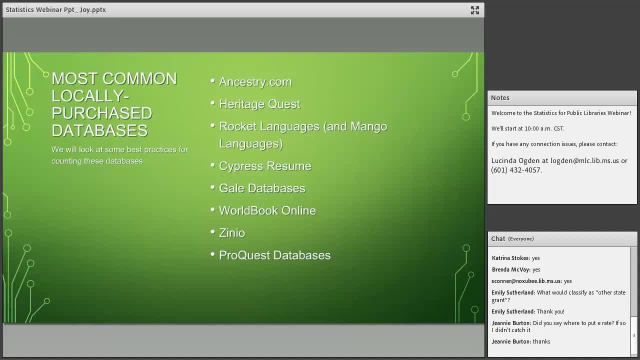 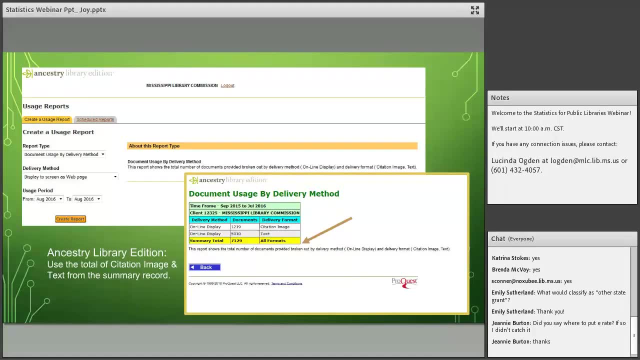 actually let me make this smaller because I'm not able to see your comments. okay, so here for ancestry, you're going to use the number, the total of your citation images and texts. so a lot of people want to just count searches, and the actual definition for this question says that this is the 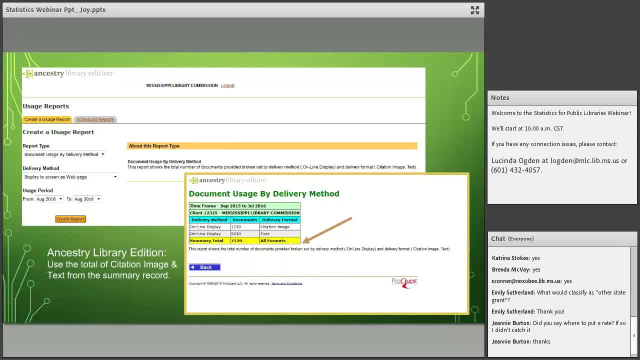 number of full content units or descriptive records examined, downloaded or otherwise supplied to the user from online library resources that require a user authentication but do not have a circulation period. examining documents is defined as having the full text of the digital document or electronic resource or a copy of a document and not a copy of the document or electronic. 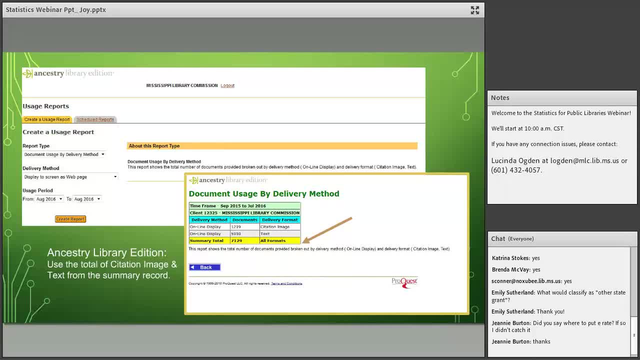 resource or electronic document, or electronic document or electronic resource downloaded or fully displayed. So the what we were looking at in this question is how much information your patrons are actually getting from your databases. So one search might yield 30 results and they might look at 30. 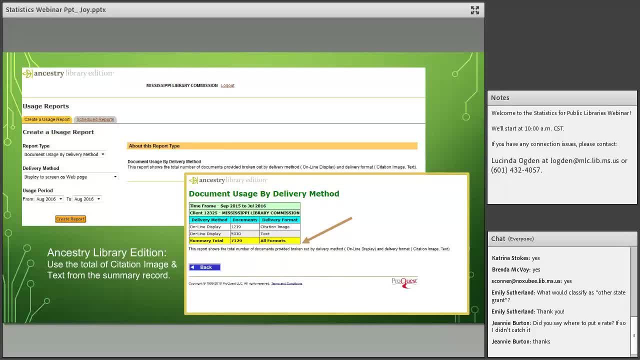 different results within that one search. So our goal, and most of these, what you'll see is we're going to be looking at the content views, the record views, the full text views, for for the majority of the databases that we have available. Some vendors do not allow you to do that, so I'll be discussing that too. But 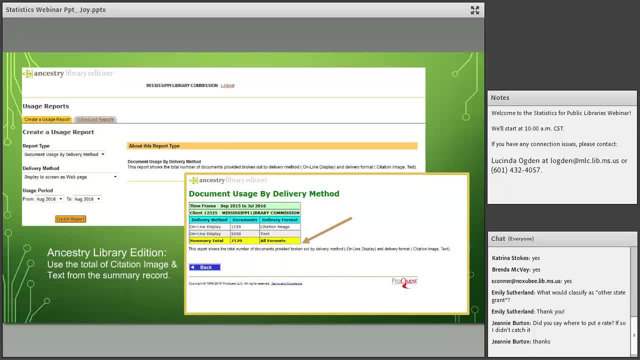 for Ancestry. you can create a usage report and our report type here is the document usage by delivery method, and I just did a usage period from August. This is just from August to August here, but you can choose your, your time frame here. You could run these reports monthly or you could just do one at the end of the 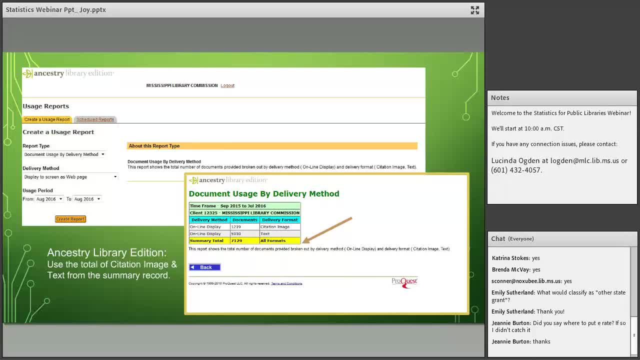 year And when you create the report, you'll see that you get a summary total for all formats and I'm actually gonna pop this back out so that we can see everything. So I've got my summary total right here. That's your citation images and your 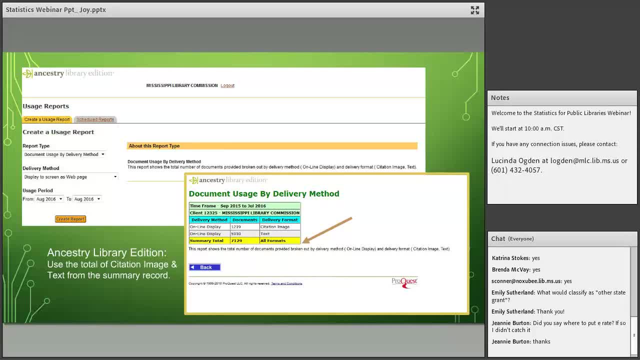 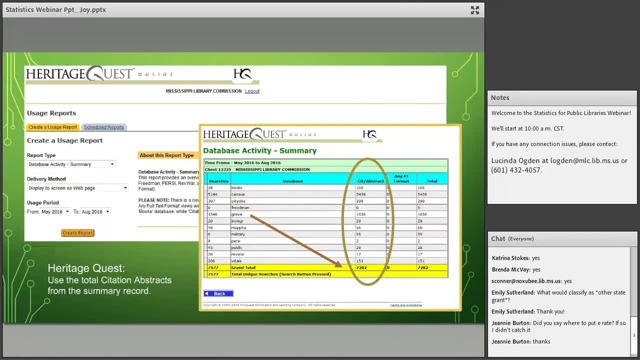 text format. So I would click that here and this is the number that I'm going to report. And for heritage quest, you'll see that we have the reporting type. it's going to be the database activity summary and I'm going to do my citation and abstract views. so you see, in this case, our searches and our views. 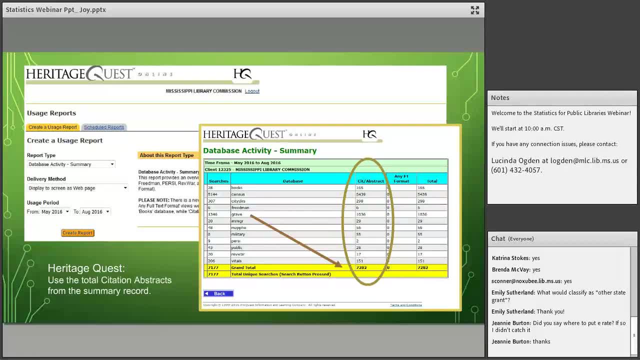 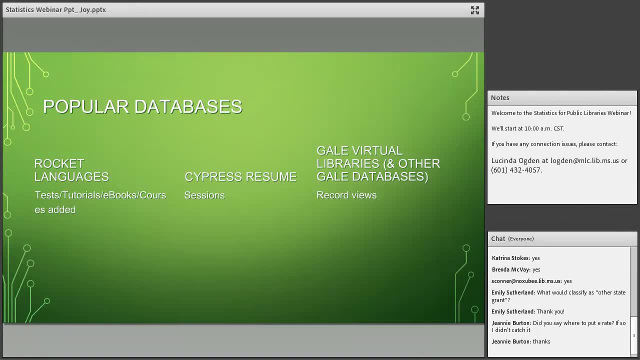 are not that different, but sometimes they are. they are a bit different, but you're going to put your citation and abstract views there for rocket languages. you will do your tests, tutorials, ebooks and courses added. so within one session a patron might get, might take a test, they may get some. 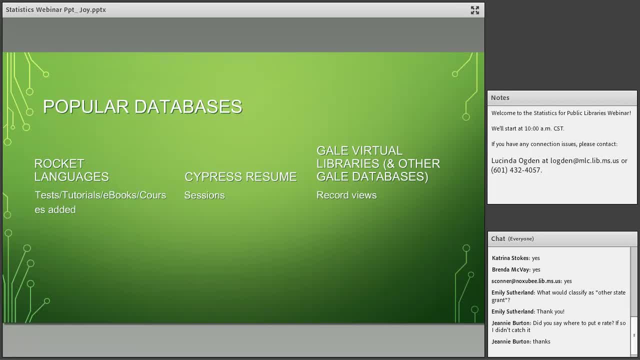 tutorials. they may download an e-book. this is a good way to show how much they're doing within the sessions. Cypress resume. however, can you can only see the number of sessions, so we just do the number of sessions there for the Gale virtual libraries and the other any other Gale databases that you might have. 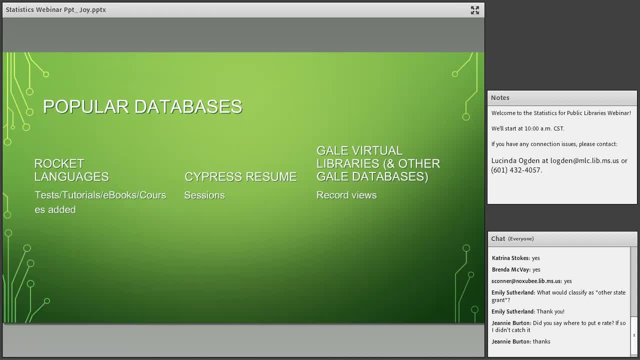 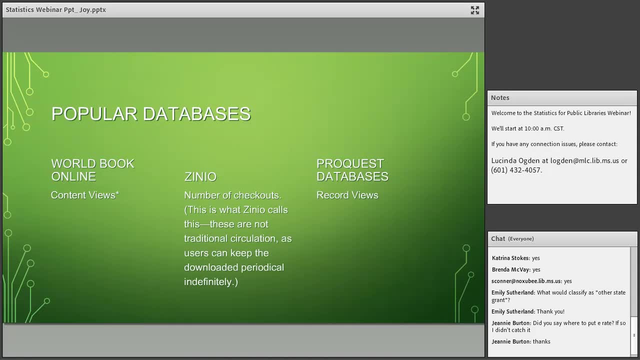 you'll do record views for a World Book online. you're going to do the content here views. I have a little asterisk there. pull that up. So the library that I got the information about World Book Online from. they count searches and that's a. 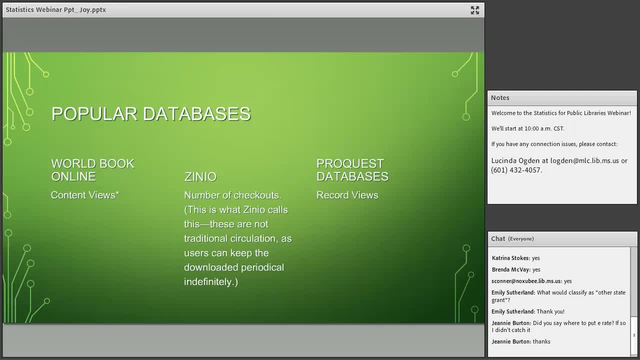 more conservative number than your content views. but here I chose to go with the content views because the definition of the element says the number of full content units or descriptive records examined, downloaded or otherwise supplied to the user. So to me the content views is a better picture. 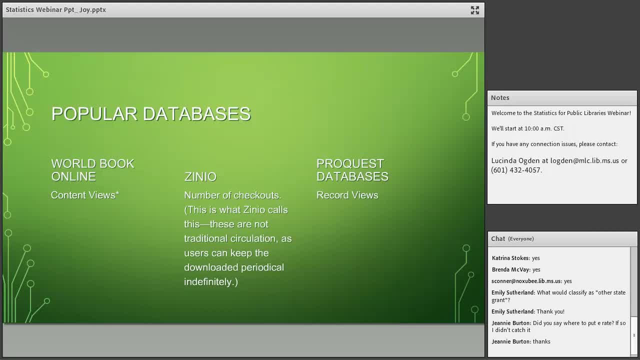 of what your users are actually doing when they're looking at World Book Online. So for Xenio we had a question because they call the use of their database. they call it a checkout, but it's not actually a checkout For Xenio when they say: 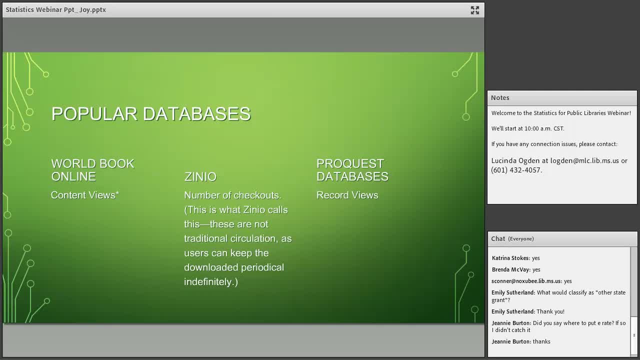 checkout, you can access the magazine and then you can keep it on your device as long as you want it. There is no return period, so it's actually a download. Therefore, the number that you count in databases for Xenio is your checkouts, and I recognize that. 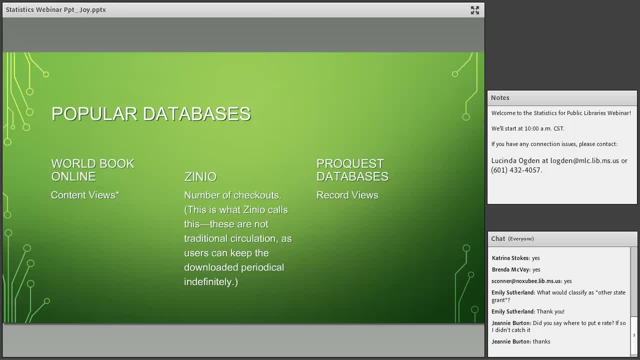 that's a bit confusing And if you have any questions about these, I will look at your comments in just a moment after I get through with the database discussion. So for ProQuest databases, you're just going to do record views, Pretty simple. 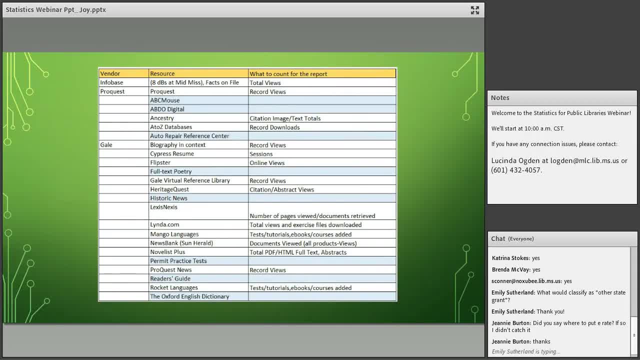 And then what I've done, and I will make this available on our website. I've gone through and I have listed a list of resources and I'll get to the question about Mississippi Digital Library in just a second. I've listed the resources. This: 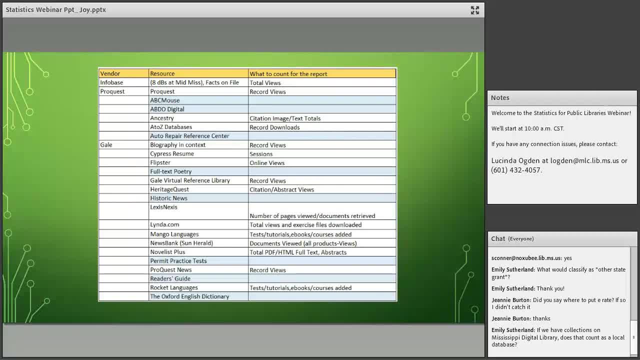 is an alphabetical order, and then I've listed what to count for the report. As you can see, there are several blue blocks where I do not have what to count for the report. I have not been able to get this information and I've asked several people to supply some of the information, and that's pretty much it. 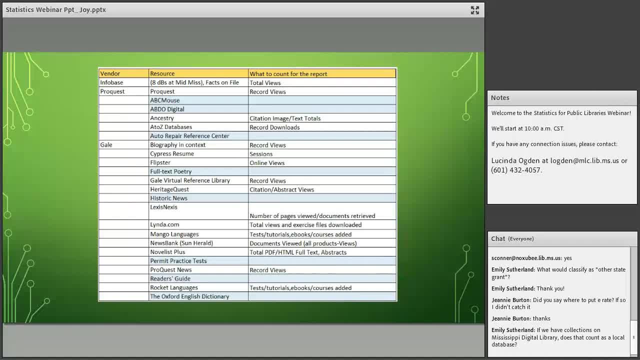 their reports to me. if you have reports for any of these, I would love to see them and I can go ahead and populate these fields for you. so, as I said, this is a work in progress. this first year is going to be a little rocky, so we may not. 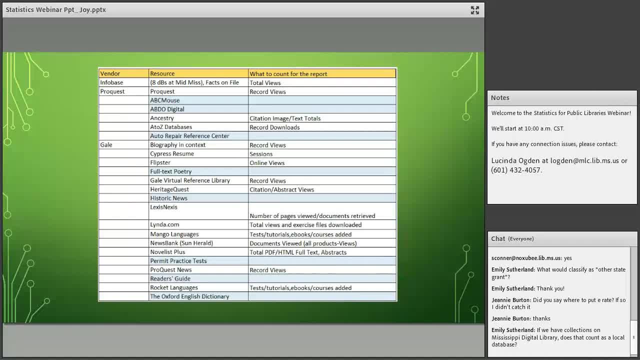 have the perfect numbers for everything. but that's okay, we're just we're getting there. so for ProQuest, you're going to do your record views info base. you're going to do total views, ABC mouse and ABDO digital. I'm not sure about those Ancestry. we discussed that. that's going to be citation images and text totals. 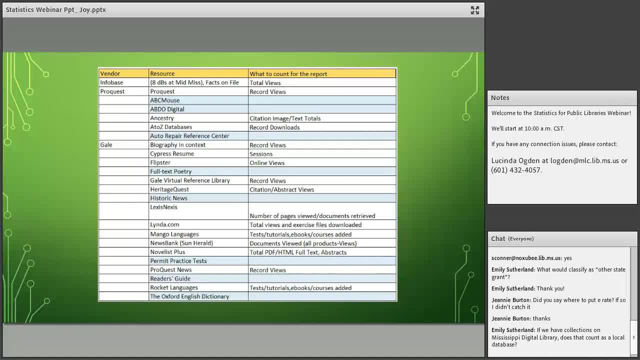 A to Z is your record downloads and I won't read through every single one but you'll see, for the most part we do our record views, online views, citation, abstract views for lyndacom and Mango Languages. we, for the tutorial kind of websites or databases, we're using total views in the exercise files or any kind. 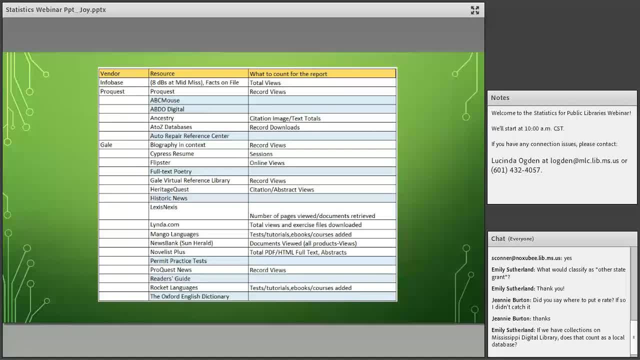 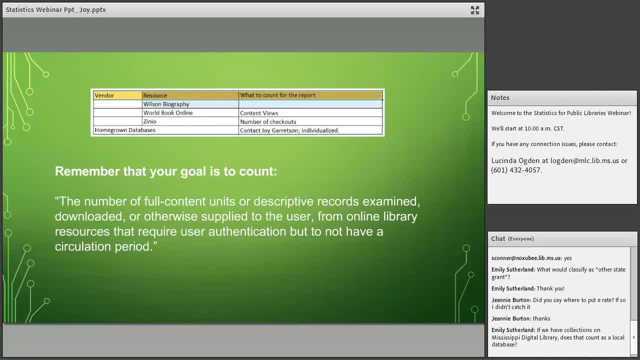 of tutorials and ebooks that they can use. let's see, and this, like I said, I am gonna post this on the website and I'll send it out in an email- the next page and we have Wilson biography. I don't have that information. rulebook: online content views. Zinio is going to be the 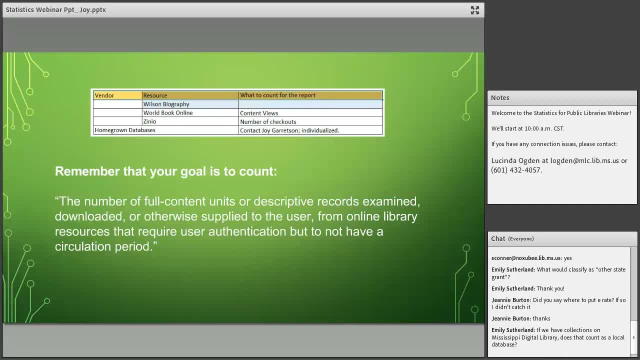 number of checkouts and then any homegrown database that you have. say that you created a history collection at your library. contact me, we'll figure out how to count that. and then likewise with your email account, whether it be the newsletters, your course欢¬¬££¢¶¢¢©¶¥®½©¸¥¥ª¸¢£ª½, ±½¥½©¥½·½©½¬½½¼¥½½¥ª½½¸, ©¬¬££¶¼½½½½½©¼½½¥½½¥½¦½¼ª¼¼½¼½½¼½¼¼¼½¥¼¼¼¼¶½½¥¼¼¼½¼¼¼¼¼¼¼� 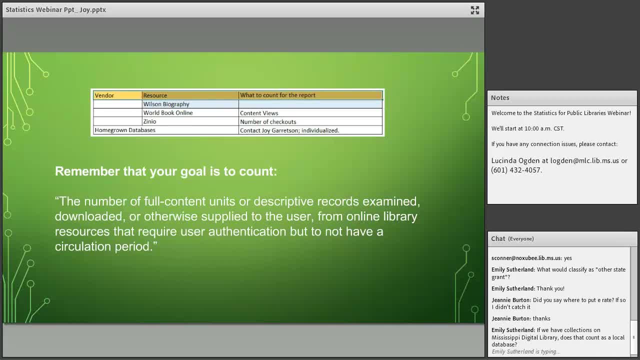 that they give you, and I guess my main question would be: are those numbers the total number of people at your library who have used Mississippi Digital Library, or is it just information about who has looked at the items that you have uploaded to that database? did you catch that, Emily? is it the total users? 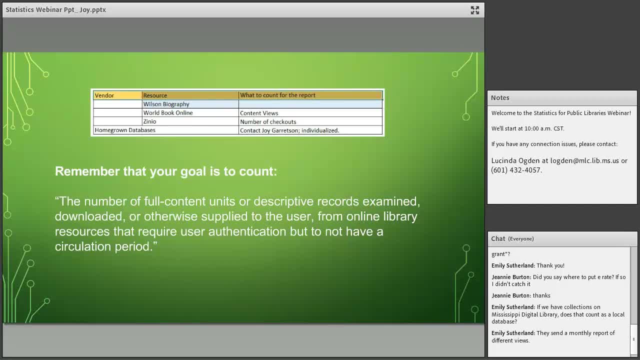 in your system, or is it just use of the items that you uploaded to the database, but it's one of? isn't it's the number of times one of your items is accessed correct, one of the things that you've uploaded? okay, I think that what we'll do. 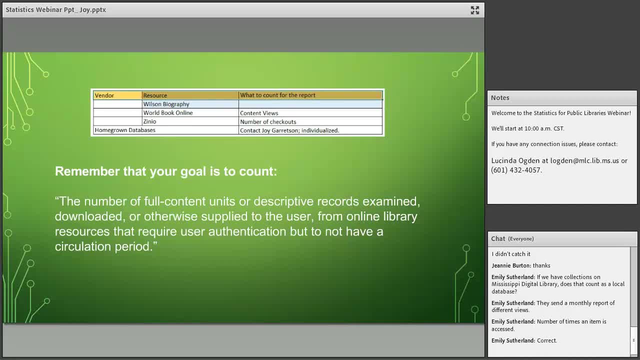 if you'll send me. can you send me a screenshot of you, what your database, what your report looks like? if you'll send me that screenshot, then I'll send out. thank you, I'll send out an email about it. what I think I'll do is have y'all go ahead and count those. I think there are nine. 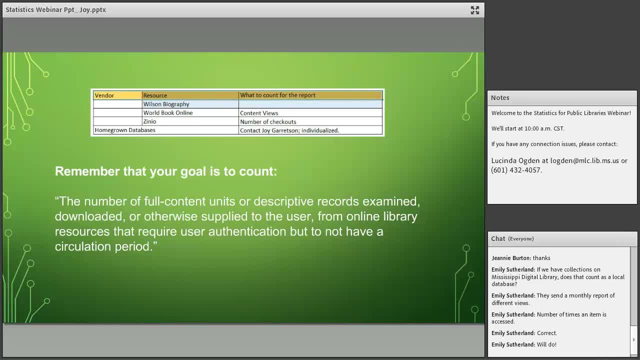 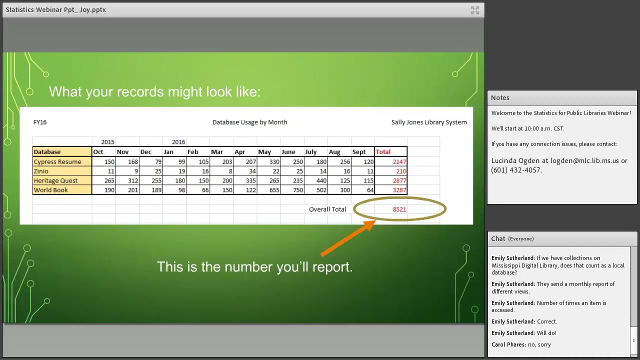 public library systems in the state that are partners in the Mississippi Digital Library. so it would y'all would be the ones who are getting those reports. so I will try to give you a standardized way to count those reports that they're Nós. okay, this one, all right. 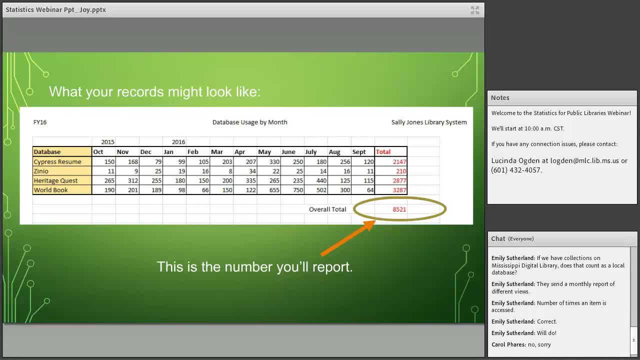 four databases at your library system and you might look at them- you know, monthly- just to see how they're used. So you could just put in your statistics every month for the different databases how many items are accessed and then you'll get your total for the year and then you're just gonna give me that. 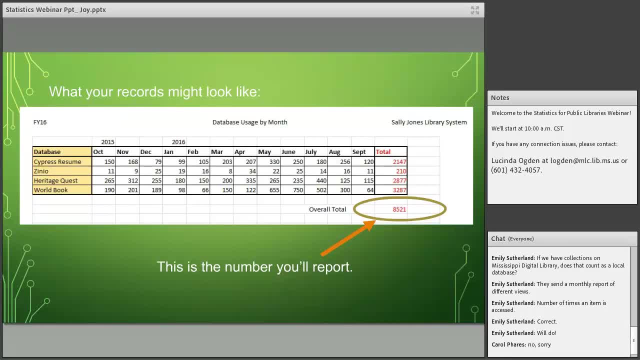 total number there. If you want to break it down in the notes section, you're welcome to do so. That would be fine, and in the future we may have a field where you can put in each of your databases and then put in the numbers. but for this, first year. we're just gonna lump them all together and we'll put the number here. I only saw one or two systems that had a you know multiple, multiple databases that they purchased locally. so for most of you, you're just going to be counting. you know three, four at the most, or you might not have any, and if you, 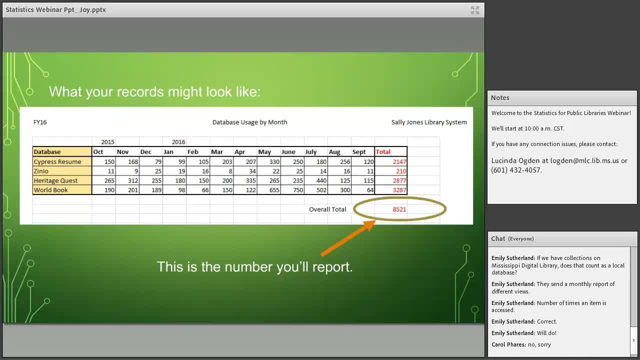 have none, then you don't have to worry about this question, though we will be putting in your information for Magnolia, But if you don't have any local databases, that's fine. However, if you do, you could just, you know, do a very simple tracking per month and then put in that. 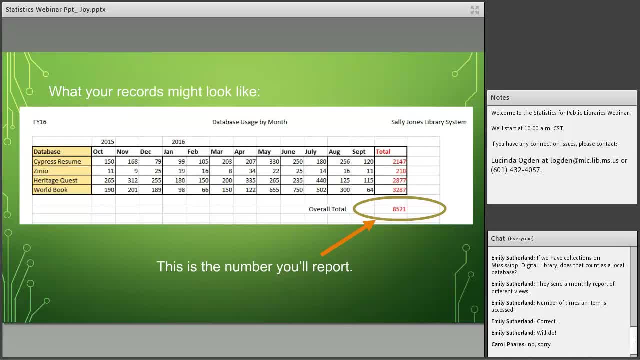 total number, And for those of you who are paying for these databases, you probably want to know how much they're being used, because I know they come at a substantial cost to you. So I hope that this is something that you're already doing. I hope you're already looking at your numbers from month to month. 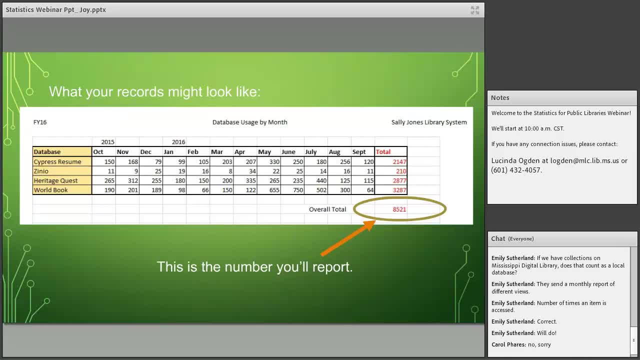 Does anybody have any questions about this? before we move on, I did want to say: some of you, we told you all about this database called Scola back in May, I believe, And a few of you decided to sign on and get it and we're paying for it for you for the first year, So this year, since we are 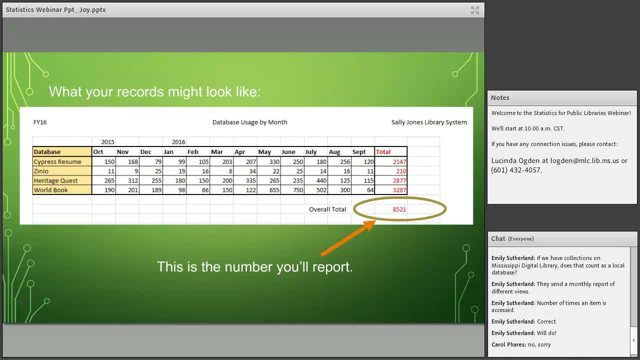 paying for Scola. we will report that to you and I'll put that in your little database note. But next year if you decide to go for Scola- you're not going to have a later database report to continue use of that database- then you'll pay for it and you would report. 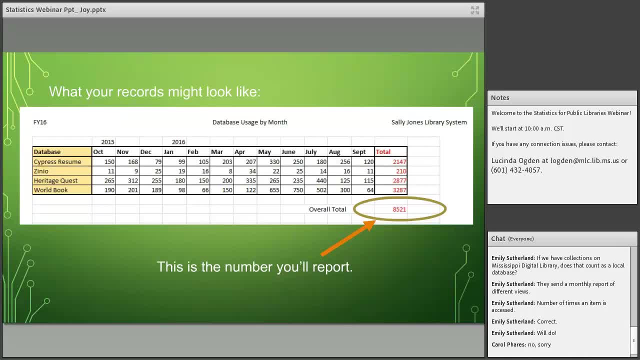 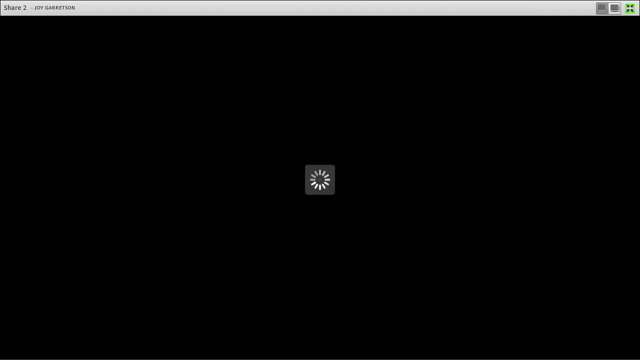 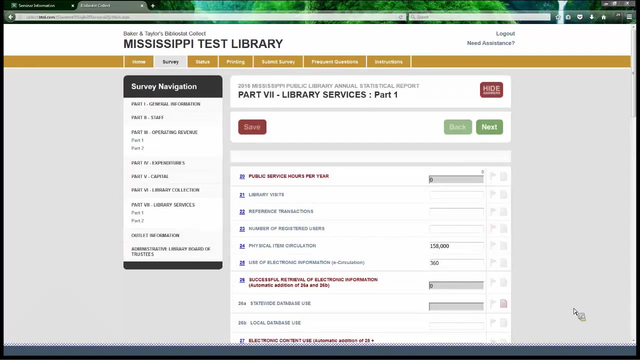 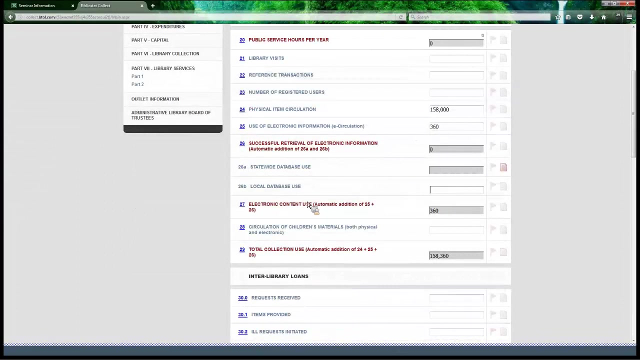 that number. All right, we are going to go back to the sharing other screen, so hang on with me while I make the switch And I hope y'all are all hanging on Again. let me know if you have any questions over here. So let's see, we left off here at local database use So number. 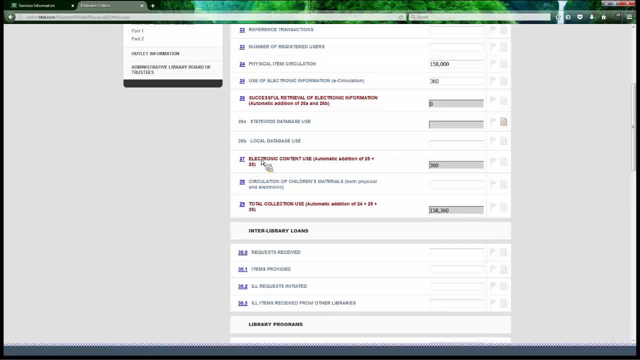 27,. this is an automatically calculated field. This is your electronic content use. This is going to be the total use of your ebooks and of your databases. You had 521 uses of your databases and 360 checkouts from your ebooks, So that 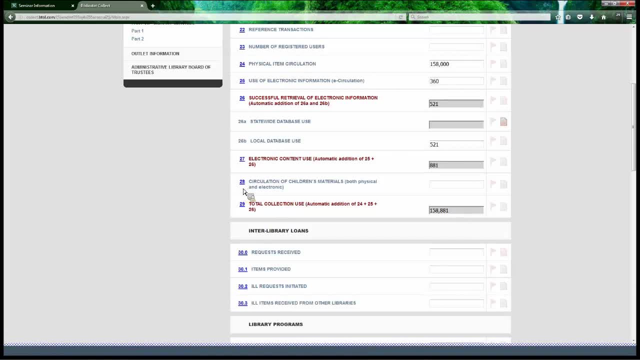 would be 881 there. Ok, so now we also have circulation of children's materials, and this is. this is a little bit separate from everything else. We realized the SDCs were talking about this in our little email group. we realized that we didn't. 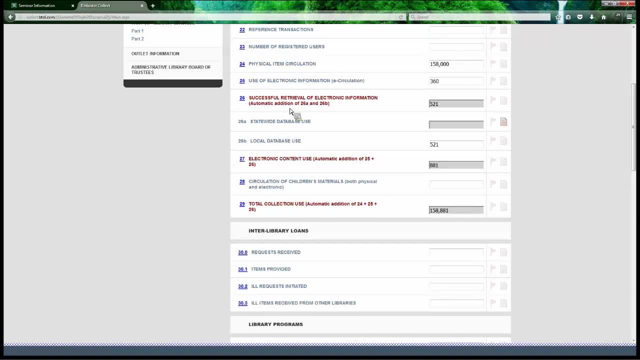 create a way for us to track the children's for each of these questions. so we'll try to fix that in future reports. but your circulation is here and this number is not going to be added to anything or subtracted from anything. your total, your total physical item circulation up here. this includes your. 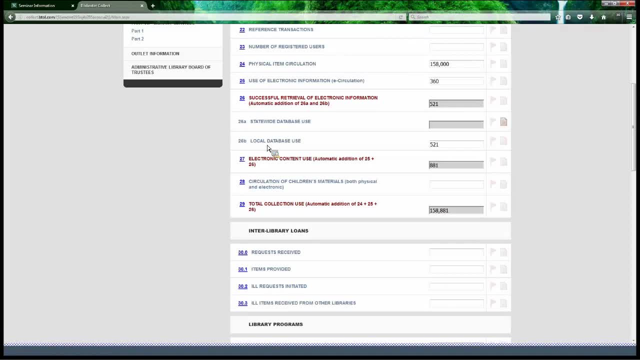 children's books. this includes everything. this is just a way for you to look at what has circulated from your children's collections. so you'll notice if I put you know, forty five thousand here, that's not going to go anywhere. it doesn't add to this number down here, it won't take away from this number up here. 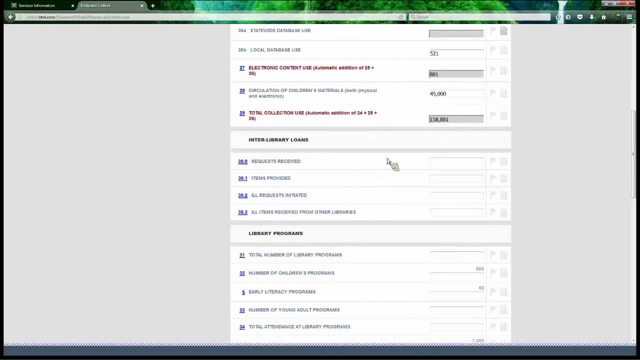 okay, so now we have interlibrary loans. remember that this is only items that are requested by a patron at your library, provided to a patron at your library or sent from your library to somebody else or from your library to somebody else, so these are things that go directly in and 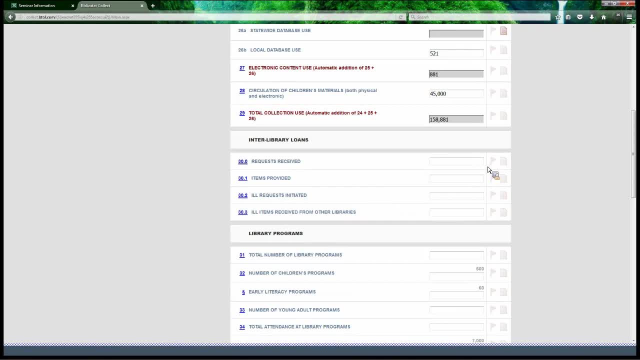 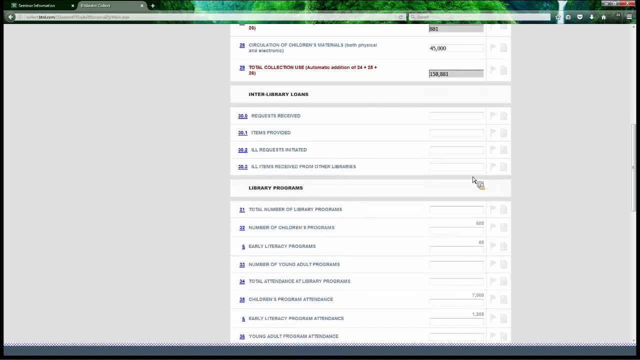 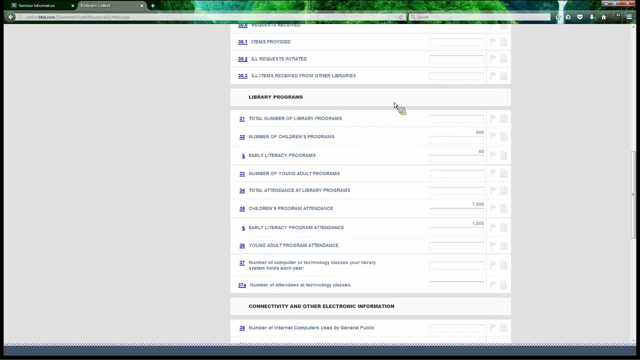 out of your library. if you are part of a consortium, do not put your full consortium numbers, just put the numbers that directly come from your library. okay, going down, we have our library programs really quickly. I just wanted to make a note. so say you have 500 total programs and 400 of them are children's. 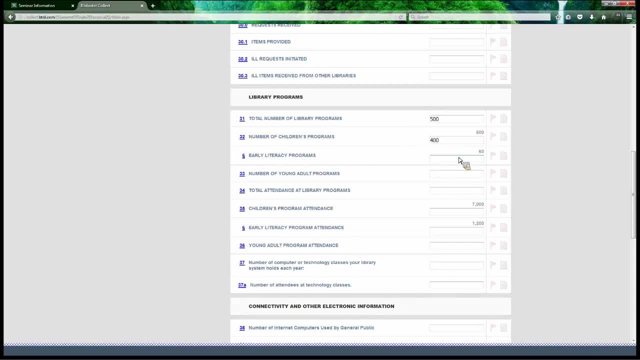 programs. early literacy is just a subset of this. it's not subtracted from it, it's just a subset. so of the 400 programs that you have for children, maybe 50 of them are early literacy programs. this is just a way for us to track what you're. 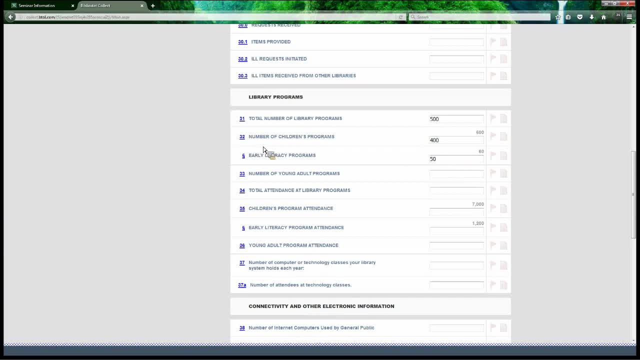 doing for early literacy. now young adult programs are separate from children programs- children's programs- so you might have 13 young adult programs. so if I were to look at this and I saw that you have 500 total programs- you have 400 children's programs and 13 young adult programs- I would probably 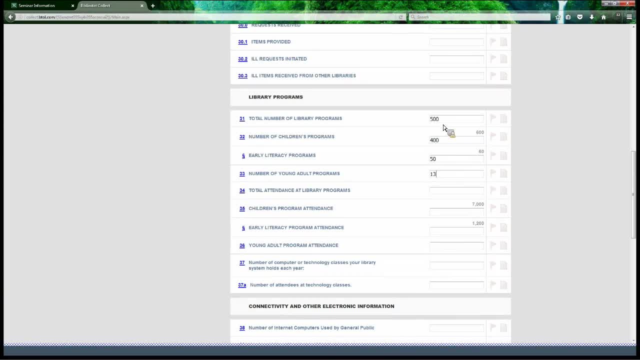 subtract 413 from 500 and I would say they have 87 other programs. possibly these are adult or family programs. that's sort of how I look at this. okay, then you have your total attendance at library programs, so maybe you have 10,000 people would be awesome. then you have your children's program attendance, which 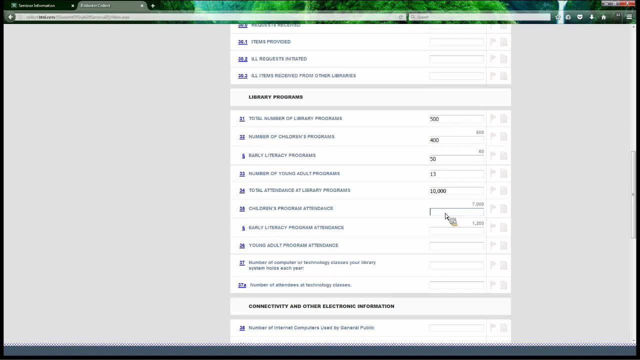 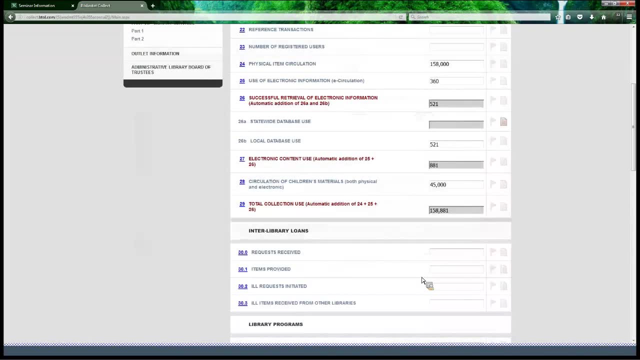 is going to be smaller than this. so if I were to put something like 15,000 people attended my children's programs, I will get a flag on this question. let me show you. you don't see it here, but when I'm trying to answer my questions we'll. 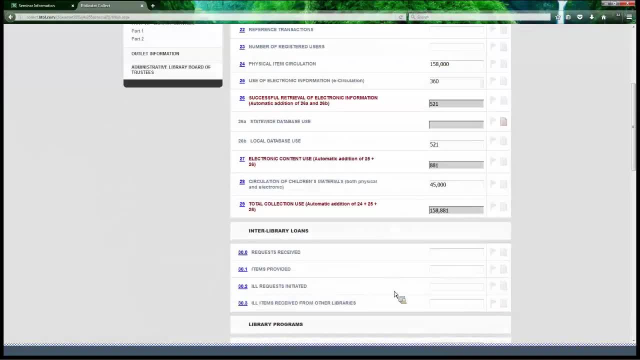 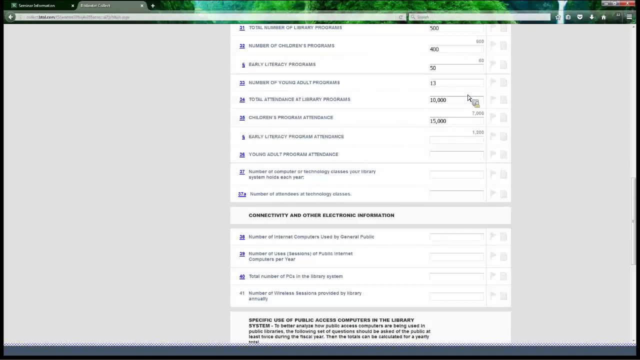 look at this. at the end, when I'm trying to submit the survey, I will have a flag, because you can't have more children's attendees than total attendees. your number has to fit within that number. okay, then we have the number of computer or tech classes your library. 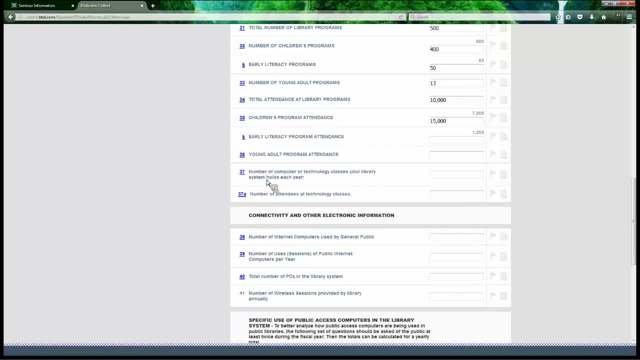 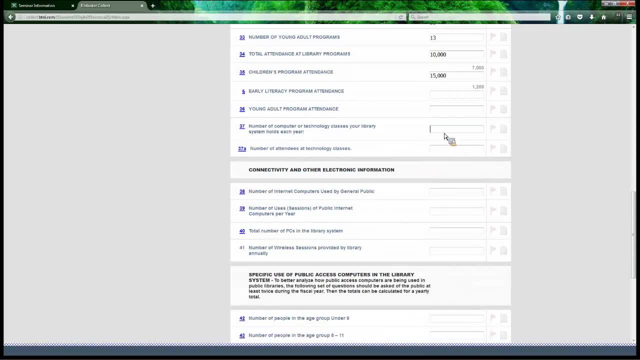 system holds each year. this is not a national question, this is a statewide question, but I felt like it was really important for us to be looking at this because this is such a huge service that we provide. so you could just put your numbers here. these are not added or subtracted to anything up here, so say, 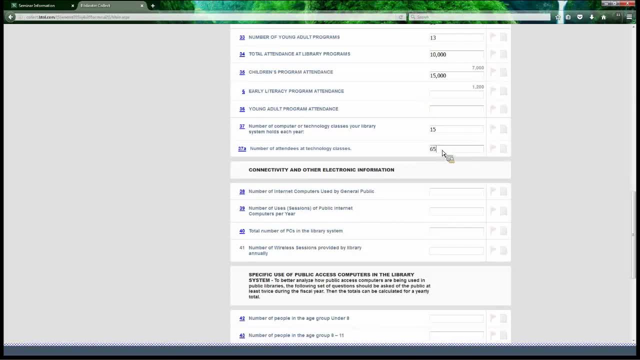 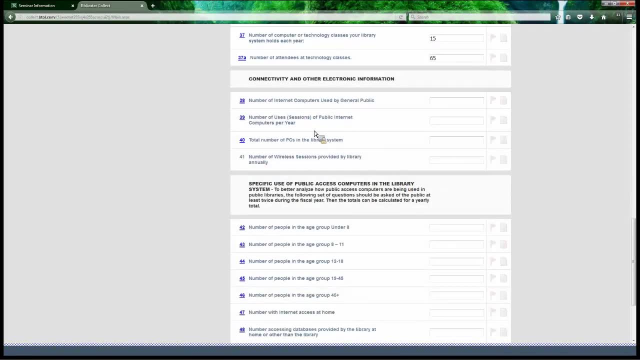 you have 15 computer classes each year and you might have 65 attendees. next we have our number of internet computers used by the general public, our number of sessions per day and our number of computer classes per day, and that's the number of year, your total number of PCs and then your number of wireless sessions. I 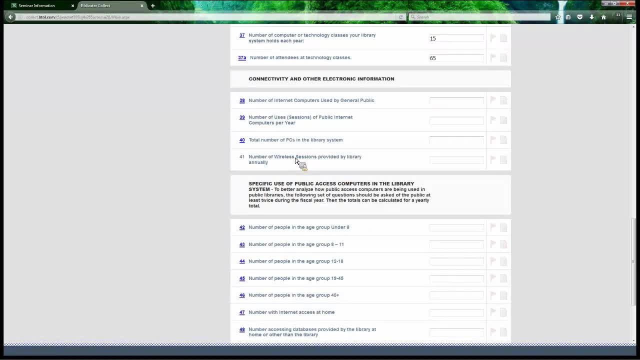 checked back, looking at the report from this past year, and 46 of us were able to answer this question, which is awesome. I know that this is a tough thing, but it's a really important number, because it does show what so many people come to your library to do, which is get on the internet, And if they're using 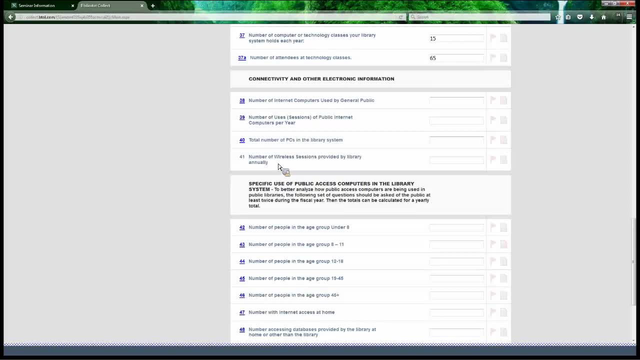 their own device. you want to try to get at the number of uses that you're getting. If you're having technical issues and you just can't figure out how to count this with your router or with a software program that I have given you all a few suggestions for those, then do a manual count. Look out at your library. 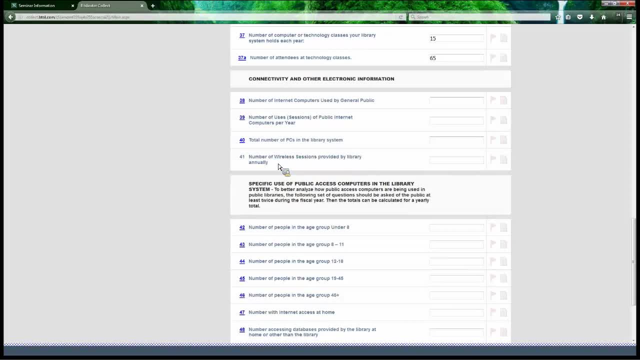 several times a day and count how many people have their iPhones out or their smartphones out, how many people are looking at their iPads or laptops or tablets, Because chances are, if they're looking at those in your library, they're probably connecting to your computer. 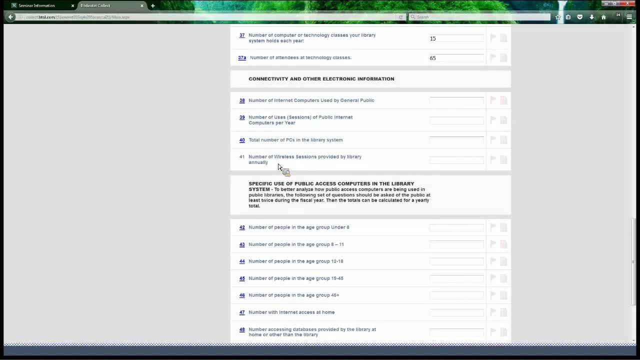 It's really hard for most people to pull out their phone and not click on that little Facebook icon and just see you know how many comments or whatever they've gotten. So you can look out in your library several times a day and count how many people are using devices and that'll at least give you an 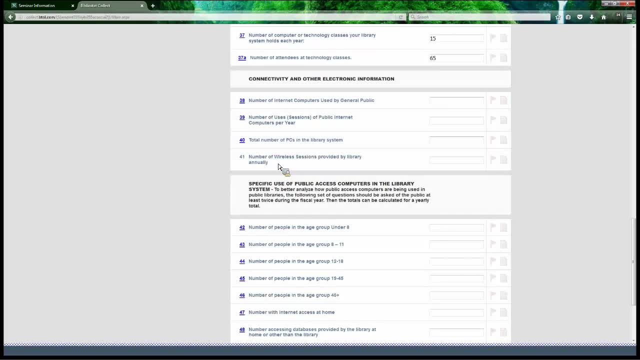 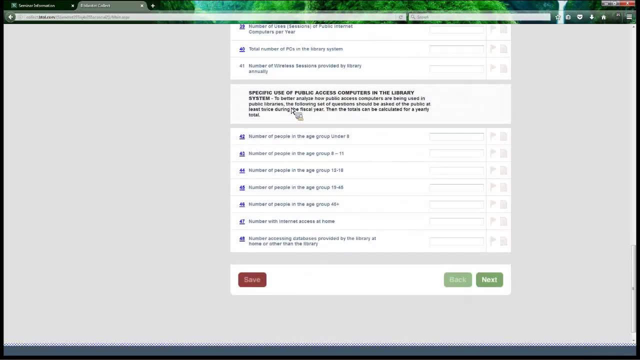 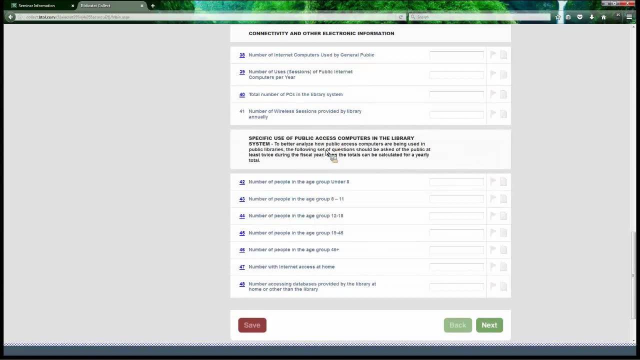 idea of your usage. It's not a great number, it's not the optimal number, but it's something Okay. and then, in this next area, is a very important I think. Just go over this and write it down. Are there any questions about that? And I'm moving a little bit quickly. Okay, for your. 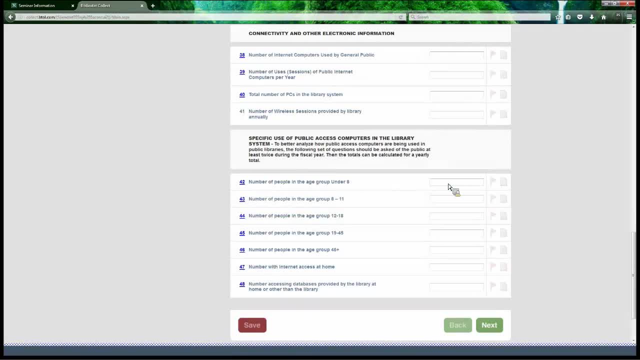 specific use of public access computers in the library system. these are those computer surveys that you put out a couple of times a year. So you want to answer all of these. Just make sure that if you run the survey for a week and you get a certain number of answers, make sure that you multiply those answers. 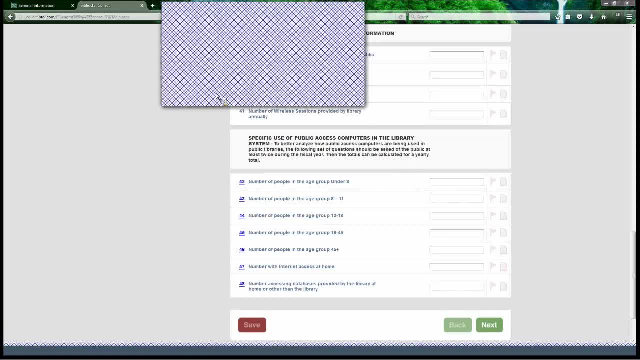 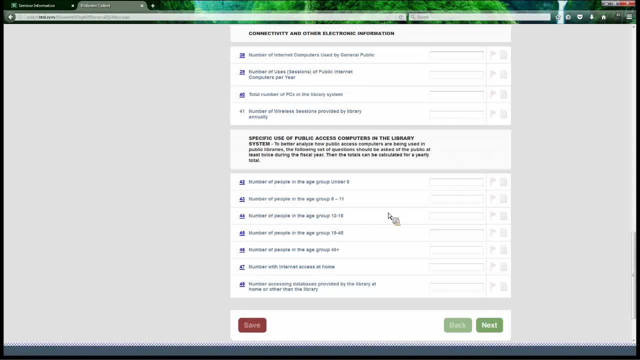 two weeks out of the year. Then you'll take all of your answers and you will multiply them by 26.. So just make sure that you're multiplying out your answers and you're not just giving your base numbers. and the reason that this is important, especially for larger systems, is that if you are not multiplying that, 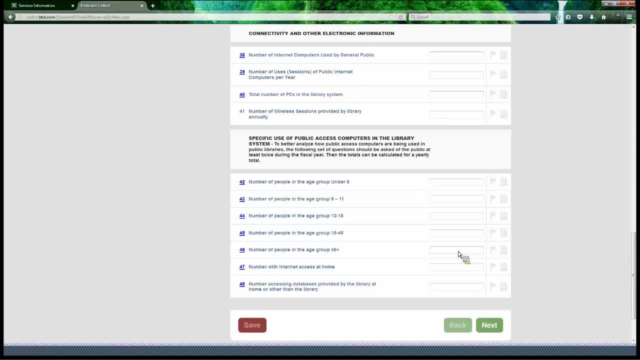 out correctly. it looks like you have very low internet usage or you have very low numbers, for you know some of these important job seeking things that people are doing on your websites or with your computers. So you want to make sure you're multiplying those numbers out to give an accurate picture of what people 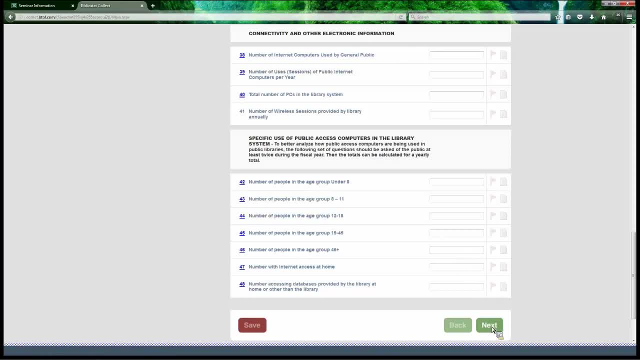 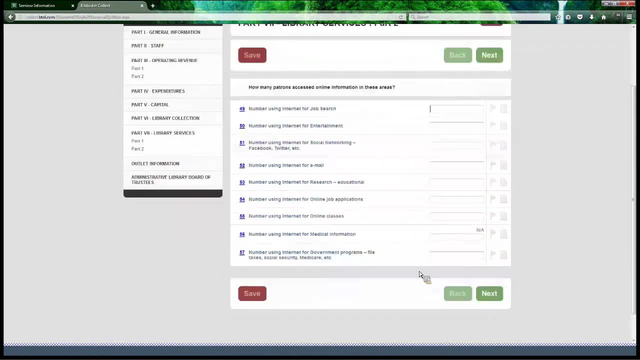 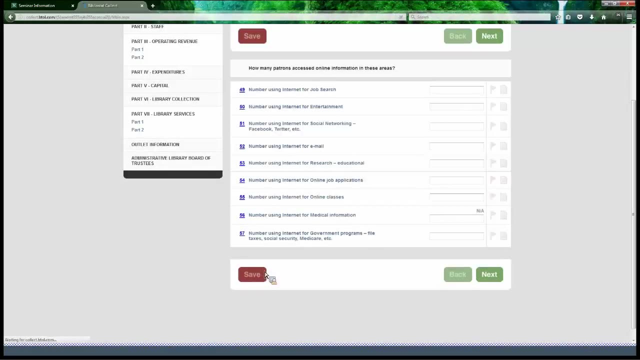 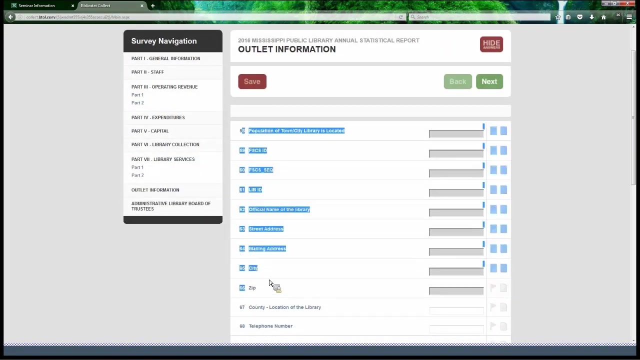 are doing on your computers. Okay, so there are several more questions here. Okay, so here's your outlet information, and you'll see that numbers 58 through 66 are going to be pre-filled for you, so your information should already be in here. If something is wrong, if the name of your library or your 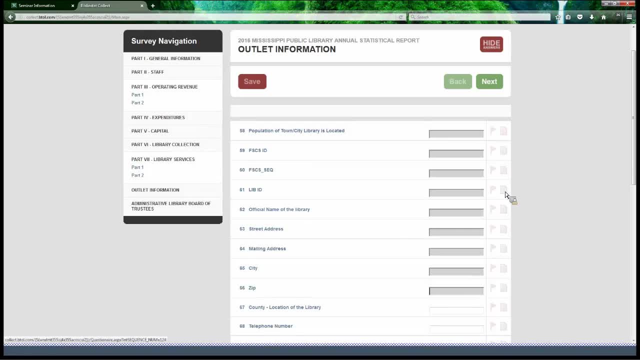 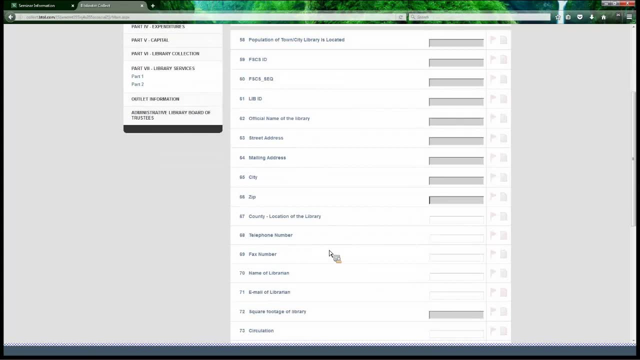 address is wrong. please leave a note for me and I will come back and find it and we will make sure that we put the right information in there. We also have your county, your telephone number, fax name and email of your librarian, the square. 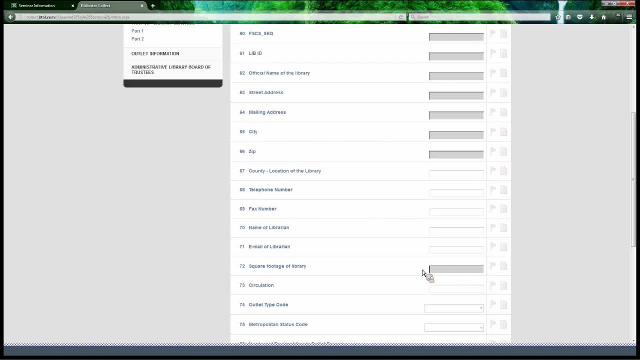 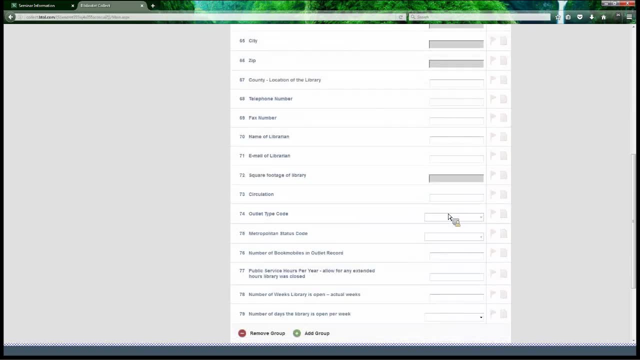 footage of your library that's also shaded out. you can't answer that. If that number is wrong, please leave a note and I'll correct it. We have your circulation at that branch, your outlet type code. this should not change from year to year. so if it does change, and generally change it back and 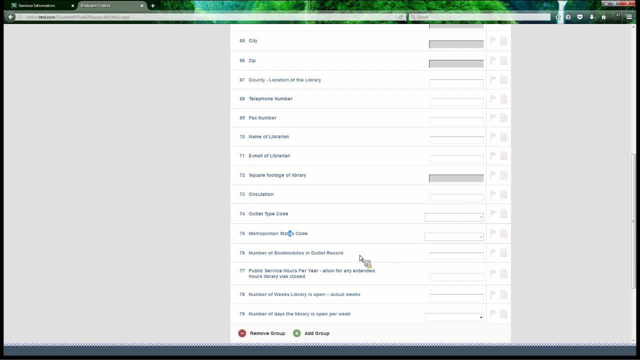 then send you an email Your metropolitan status code and then your public service hours per year. So if you're generally open 52 weeks a year for 20 hours a week, then your number- let me multiply that out really quickly- it's going to be 52 hours per year. 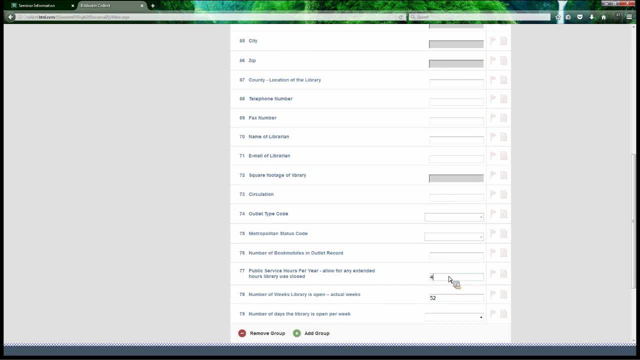 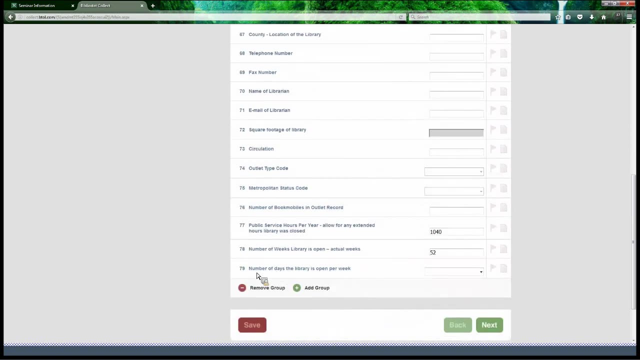 Then it's going to be 540 hours maximum. Oh, no, it's not, that's going to be a thousand forty, sorry, Okay. and then also I'm asking you how many numbers, number of days this particular branch is open per week? if it's open five days a week, it'll go right there. I'm going to save that. 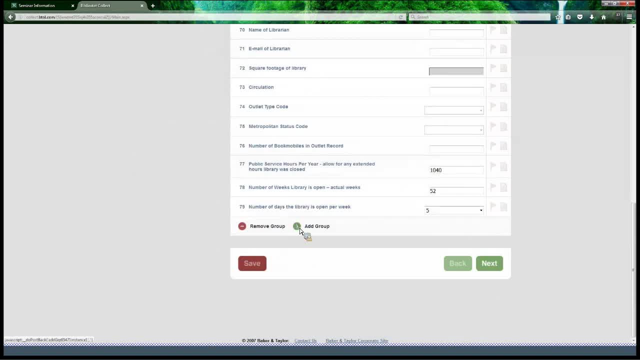 information, Then I can add a group here. If, for some reason, if you normally have a certain number of branches, if you have a group of clients in a particular place that is open branches and one is missing, let me know. Last year there was a little glitch in. 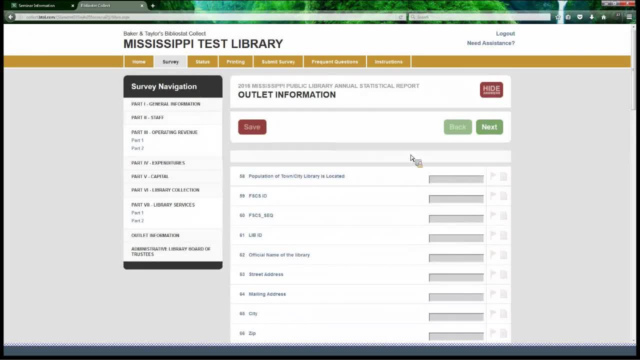 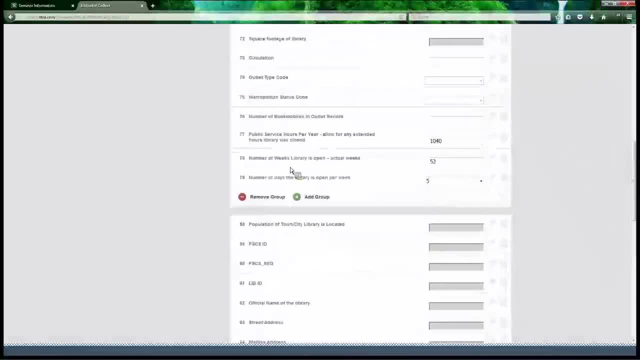 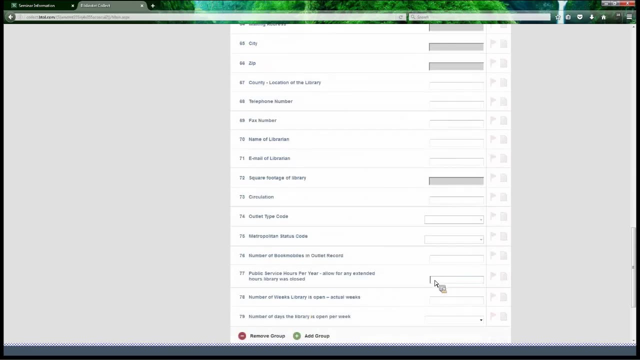 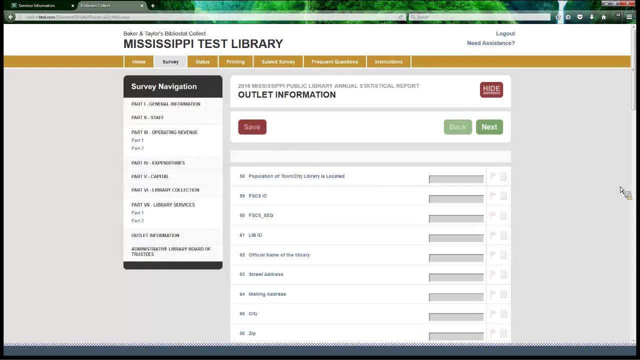 the software and a couple of people lost- lost their branch information. We can get that restored to you. So here we have a thousand forty hours that the library is open per week and then say your other branch is open two thousand eighty hours a week. I'm going to just jump back really quickly to your library services. 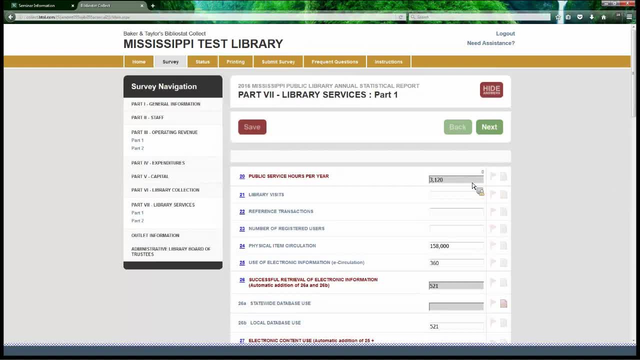 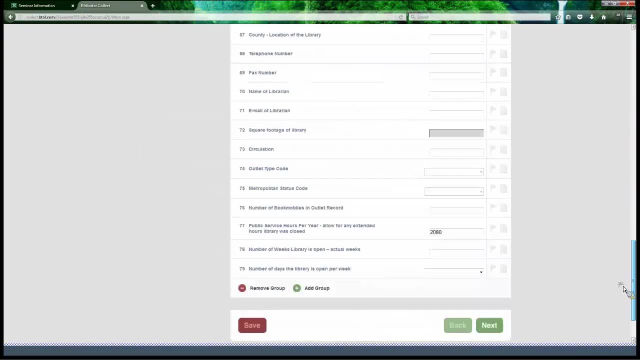 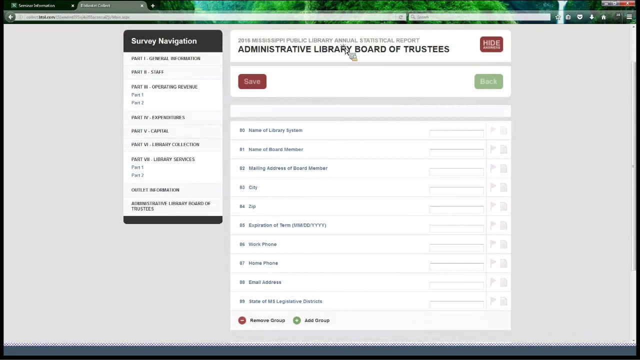 so you can see that that has populated up here. So now you see that it's got the number of hours that you've got, So it comes from your Outlook record. Okay, just gonna save that and move forward. The next information is your administrative library board of trustees. If you sent Loretta an update about your 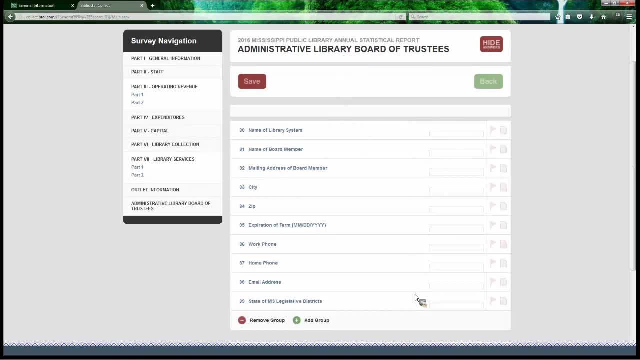 administrative board, then I'll be posting that to you immediately after that. I'm going to click on that, I'm going to go to the administrative board and you can see in the pre-filling this information for you. I know I should be getting that in. 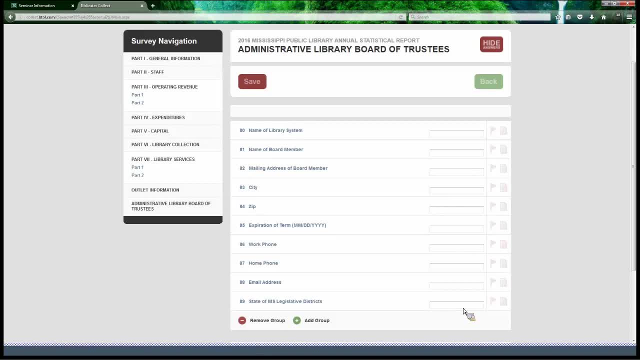 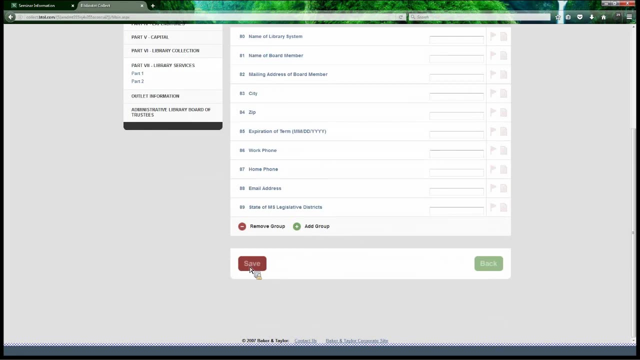 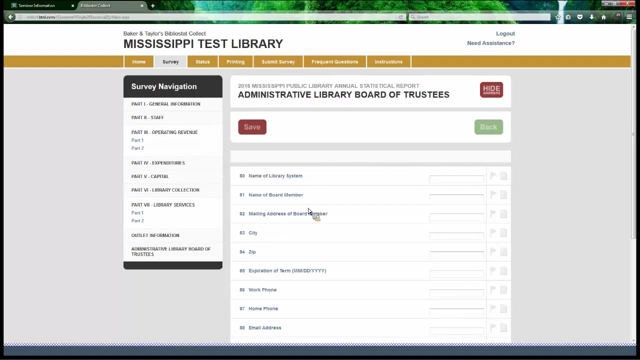 hopefully by the end of the next couple of weeks, but you can go ahead. you'll have that repopulate from year to year, so you can also just correct the information that you've already got in there. We did add an email address for them this year. Okay, so that is the end of the report. So once you get all this, 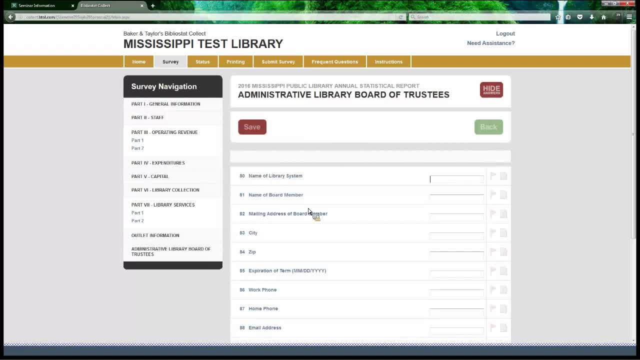 information filled out, what you'll want to do. you might want to print it off and look at it, Look at any major changes from this year to the next, and then you might want to try to submit your survey. So when you click into the submit survey, 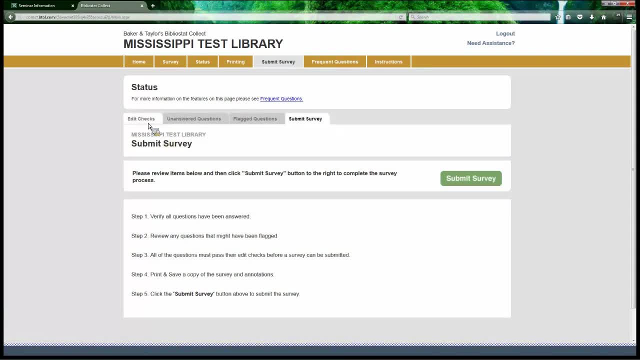 tab. there are four different, four different tabs that you have to go through, so your first step is to verify that all of your questions have been answered. So if I were to click on this tab, I would have a spaces pattern. If you don't have spaces, then you can put all the 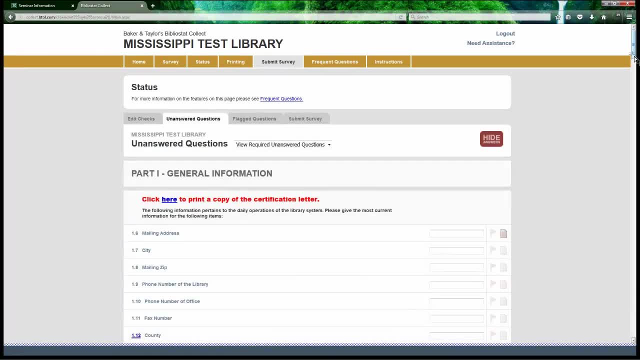 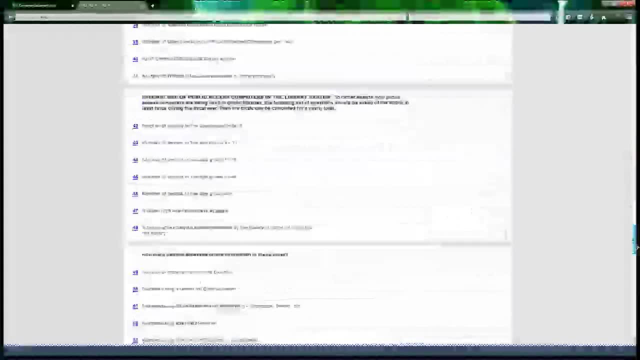 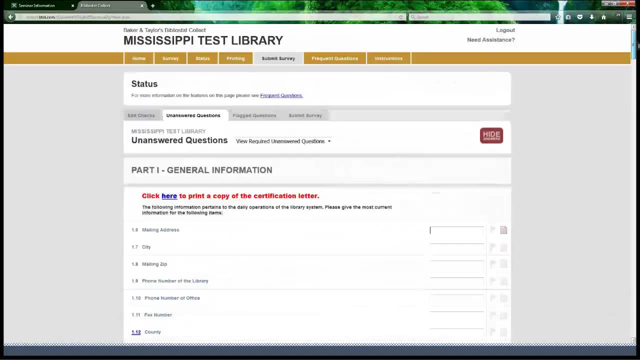 lot of questions in here because I didn't answer that much in my test survey. so you do need to make sure that you answer everything, even if your answer is a zero or not applicable. you need to put an answer in for everything. I realize I scroll down pretty quickly there. all right, and it'll also give you. 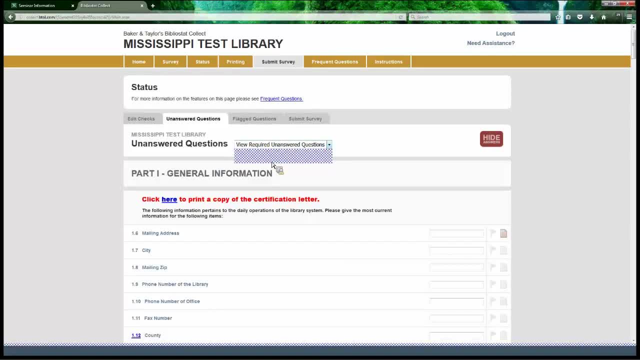 the. these are the required unanswerable questions, and then you could also look at just all, and there might be more. there required are the ones that are from the federal government. you must answer all the ones that they give you, even if you have to put in a zero for whatever question they're asking you. 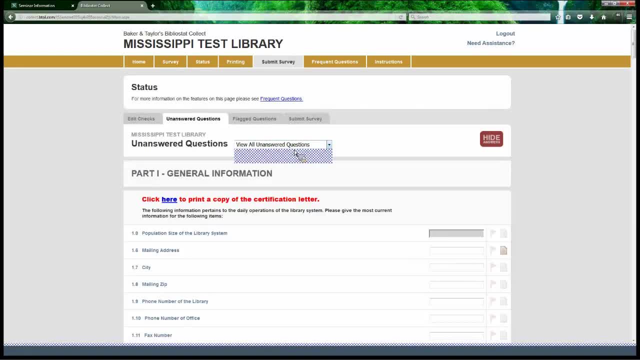 like local database use. if you have a zero there, that's fine, but you need to make sure that you answer it in some way. okay, so our first step was to verify that all questions have been answered. the next is to review any questions that have been flagged. 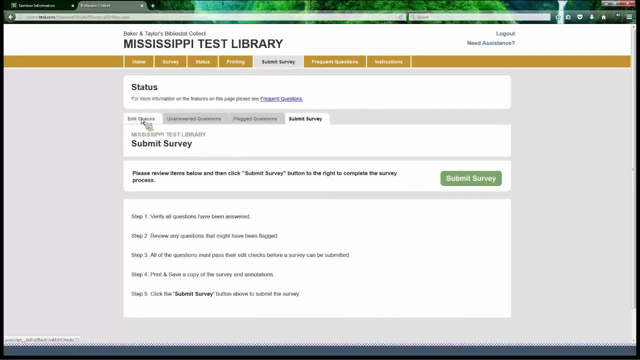 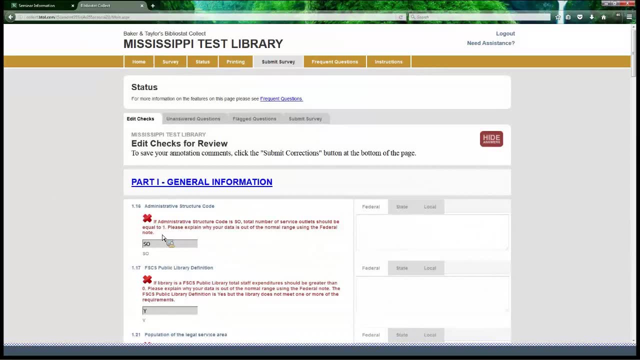 so that might be your edit checks and your flagged questions. so edit checks are going to say: if you don't have, if you have a question that's without, with outside of the range of what has norm, what you've answered the previous year, you'll get an edit check for it. that's where you're going to add a comment for. 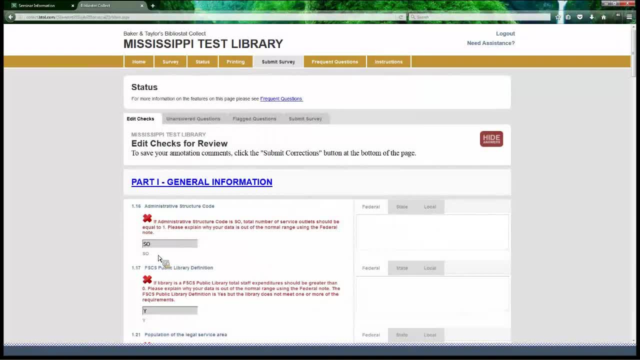 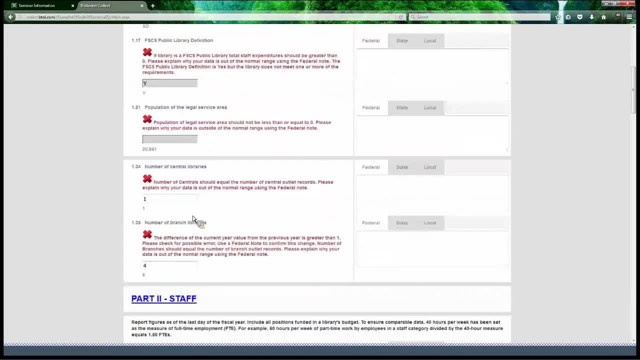 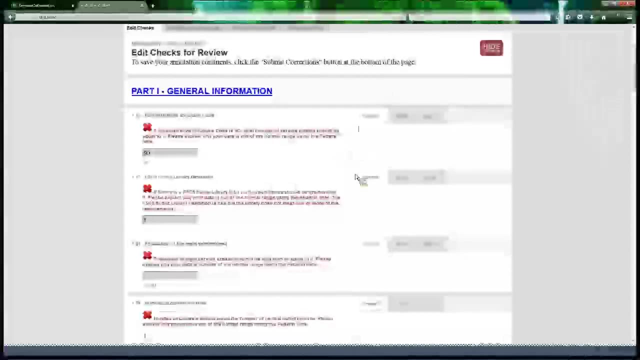 me also. you'll get an edit check if you have changed, if your answer doesn't match up with what the question is asking. so you'll need to go through each of these edit checks and you'll need to put a note in the field. so make sure that you do that for each. 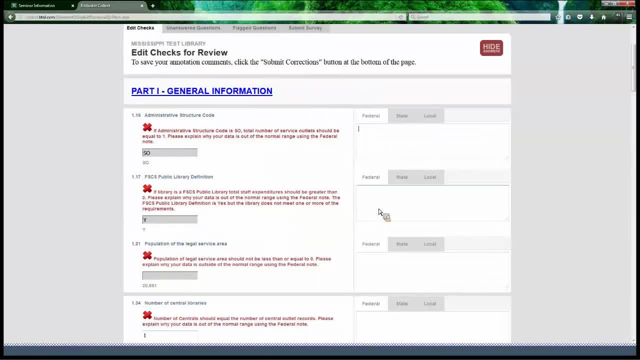 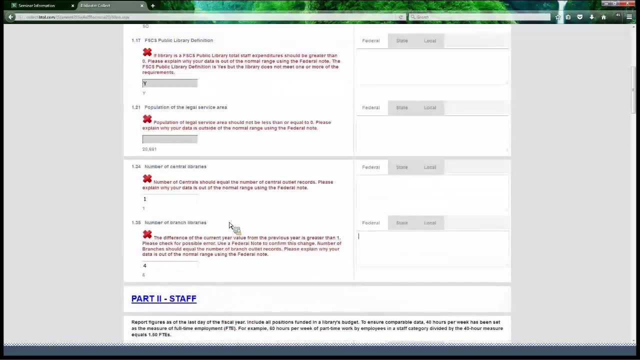 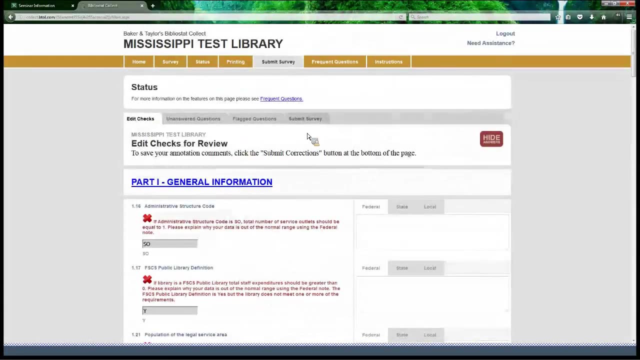 of your edit checks you want to make a note about: either change your answer or make a note to fit in here. that way I don't have to come back and ask you about this in a couple of months. so those are your edit checks, and then we'll also have your flagged questions. these are questions that have major 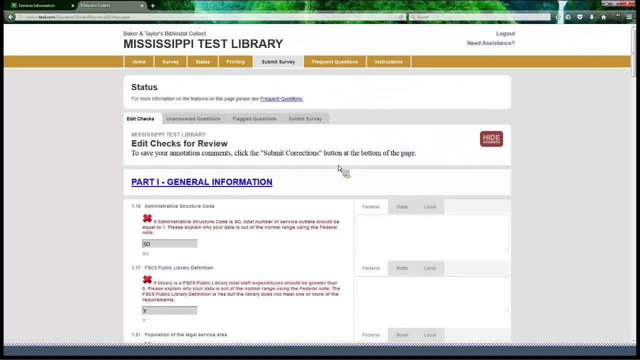 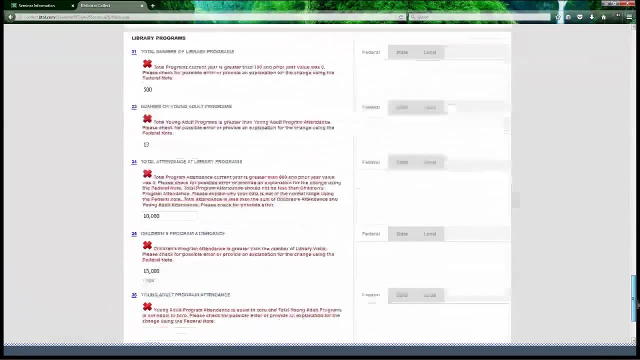 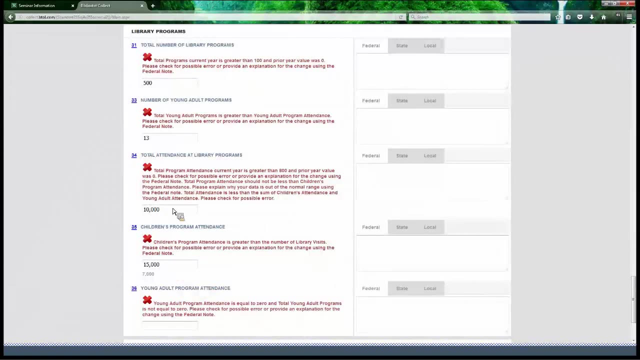 issues and I'm not seeing. I remember for the um, where is it library services programs? okay, so remember where I answered. it says that I said 15,000 children's program attendance, but our total was 10,000. here I wrote. here they say: your children's program attendance is greater. 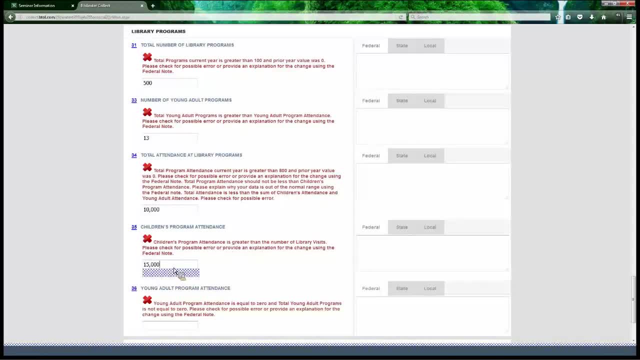 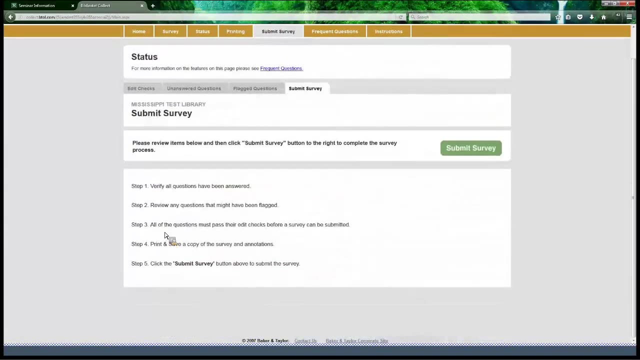 than your number of library visits. so it caught that question: oh, greater than the visits you? oh, wow. so it'll catch any major issues that you might have with one of your questions. okay, going back to the submit survey, the next thing it does is say that you 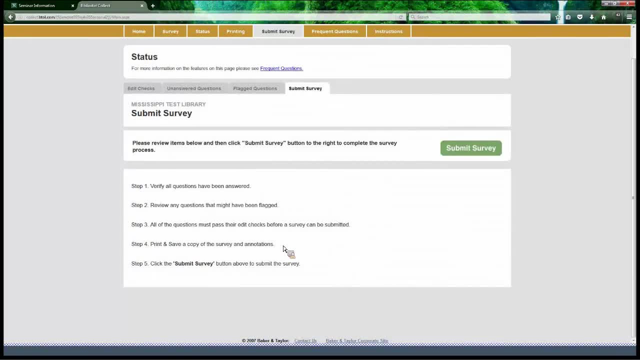 should print and save a copy of your survey and your annotations. that's very important. let me show you how to do that. if you do this, then any information that when I'm going in to look at it, if I accidentally, accidentally delete something, you'll have that answer there. or if you're looking back over and you 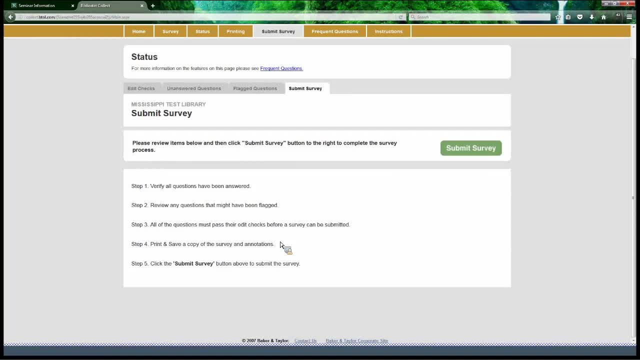 realize that something is wrong, you can check your old number against the new number. or every year when I publish those tables, I ask for everybody to kind of look through their numbers and make sure that they're correct. that's another thing that you can do with this survey that you have saved and printed. so here under printing, 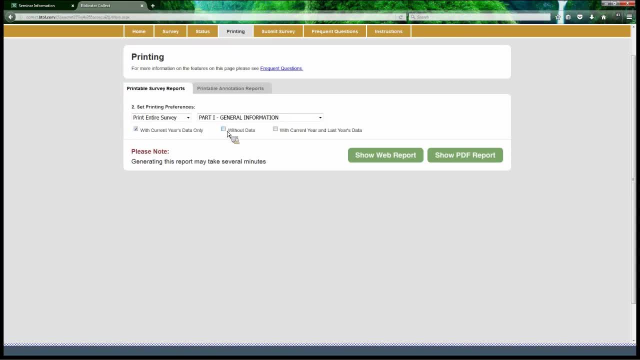 you can print your entire survey, and you can print it with your current years data and with the previous years as well. now you might just want to print a selected section for some reason, but I would generally just print the entire thing. so you can download this into a PDF and print it there, or you can just do an HTML web. 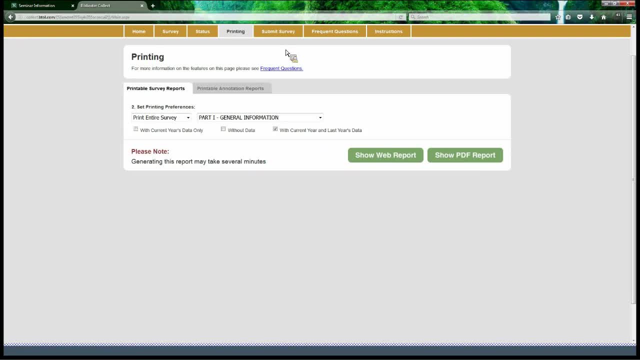 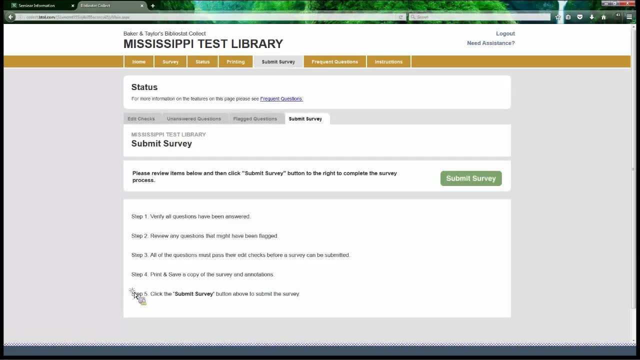 report and print it there, okay. so I asked them if they could put in a step here for you to print and send me your certification letter, and they said that they that for some reason the program will not let them at a step here. so make sure, before you submit the survey that you've printed out, that 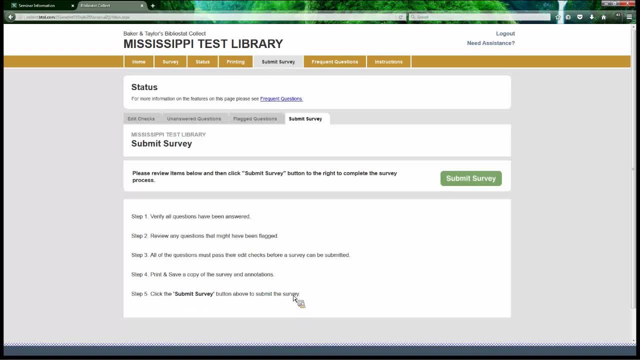 letter that was on the first page of your survey, so that you can certify that you've answered all the questions. and when you're done, you actually have to submit the survey. you cannot this just because you filled everything out doesn't mean it's submitted. you actually had to click. 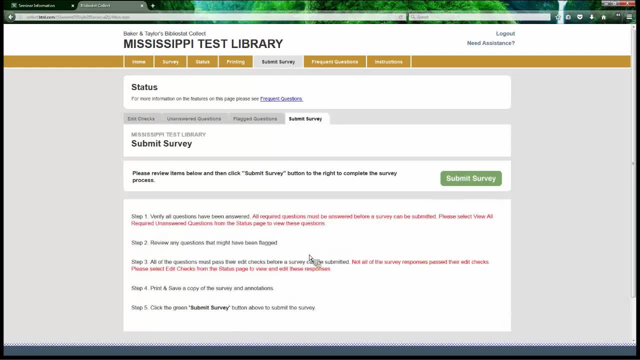 this button to submit the survey and if you haven't done, if you haven't answered all of your questions or past your edit checks, then it won't let you submit the survey. okay, so we're gonna go back really quickly to our PowerPoint. are there any questions before I leave this website? okay, great. 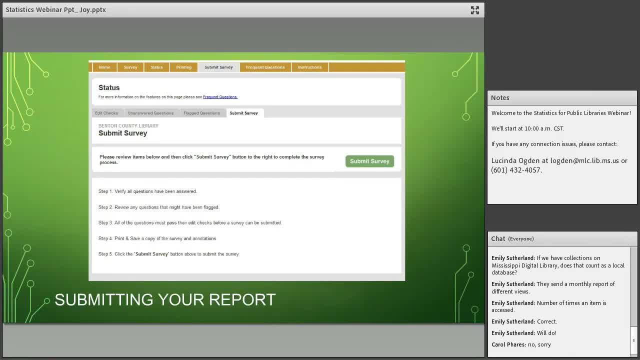 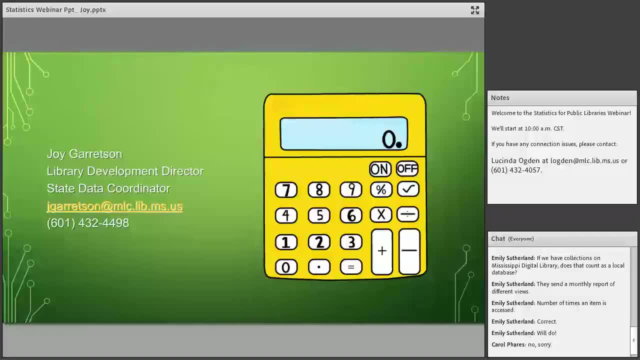 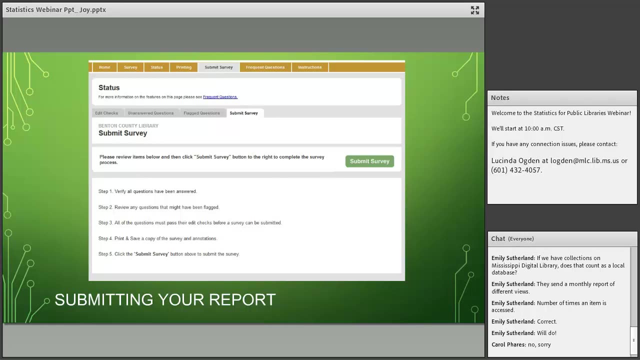 we just talked about submitting the report, so I'm gonna give you a couple of dates. oops, sorry about that, I that's not in here. so, um, the deadline for submitting the report is December the first. make sure that you push submit by that date, and then February. 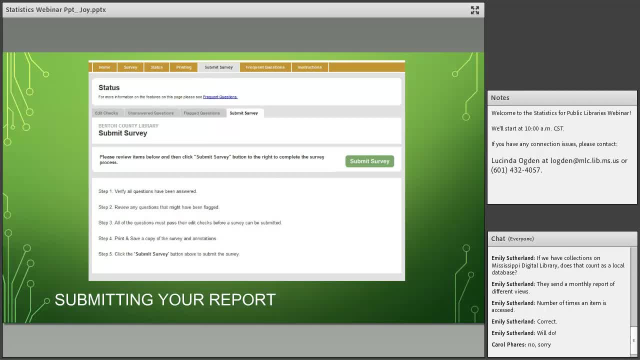 13 is your drop-dead date. that's the date after that we'll start sending you letters saying that aid can be withheld if you do not submit your report, and this generally does not happen. most people get their reports in on time and it's and it works really well. on May 12th I will try to have a rough draft of 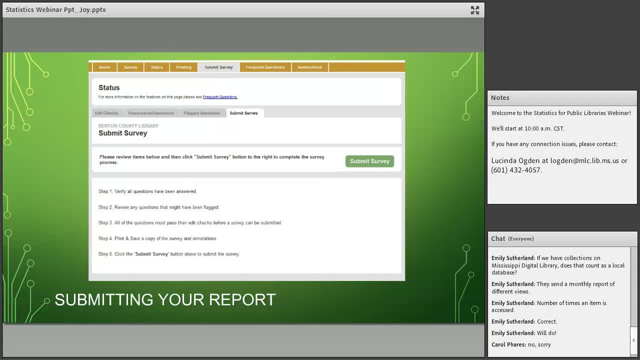 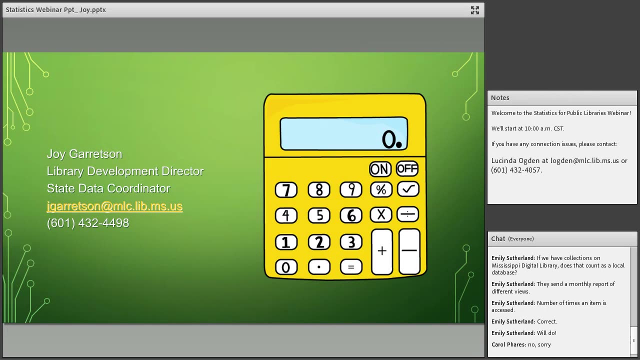 your report tables and have that ready to send out to all libraries. we try to get those in pretty early so that you can make your budget requests, any requests that you might need, and as far as actually filling out and submitting your report. that's all I have. 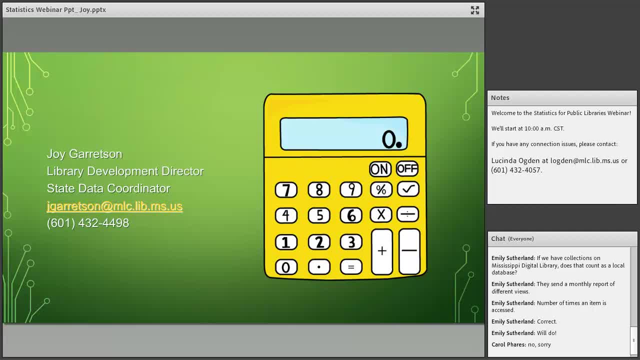 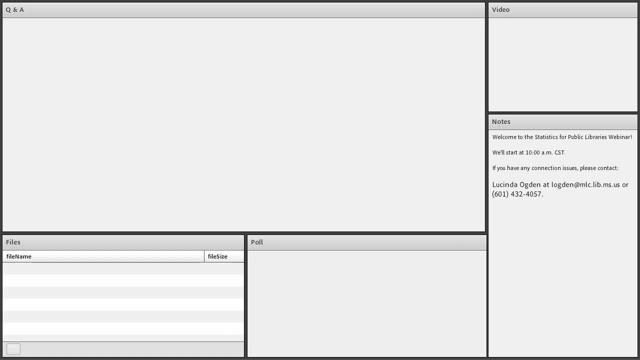 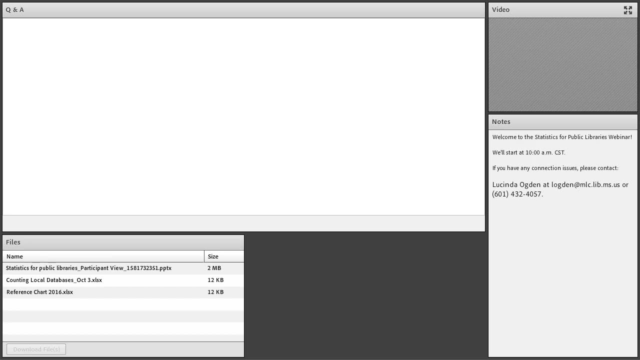 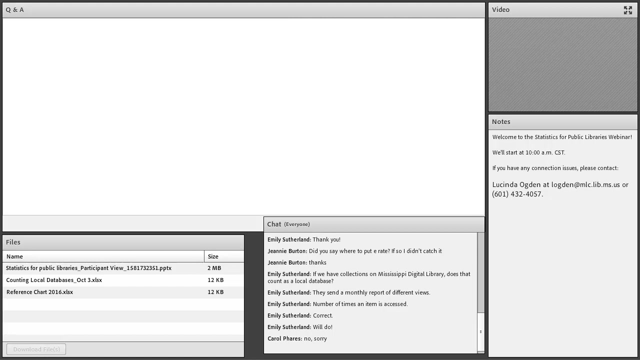 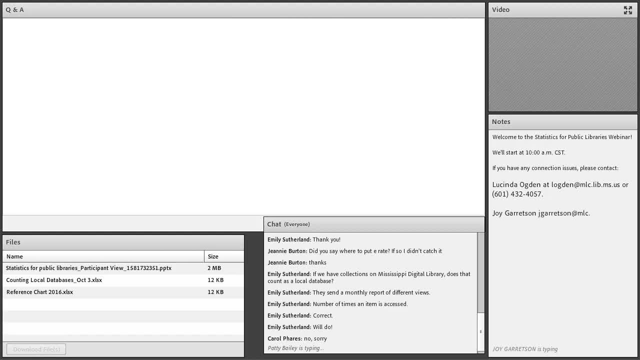 is not on this page anymore, so right here you can call or email and I'll get back to you. over here you're gonna see that I have your counting local databases file, so this will tell you how to count those and again, if you have a database that is in one of those light blue boxes: oh, Patty, um, it's changed. and 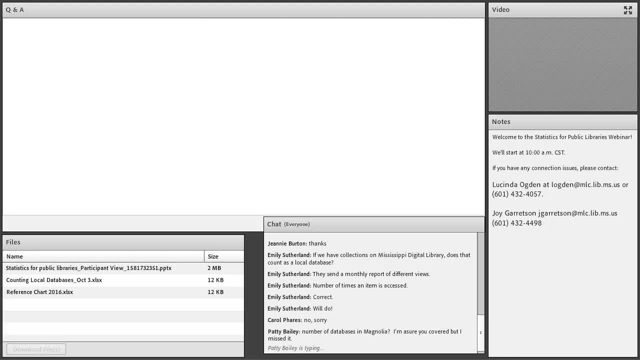 I will fill that information in for you. you don't have to fill that in. yeah, that that field is locked. so counting local databases. the information about what to count is right there. I have a PowerPoint for you here and we have the reference chart so that can help you if you aren't quite sure how to count those reference. 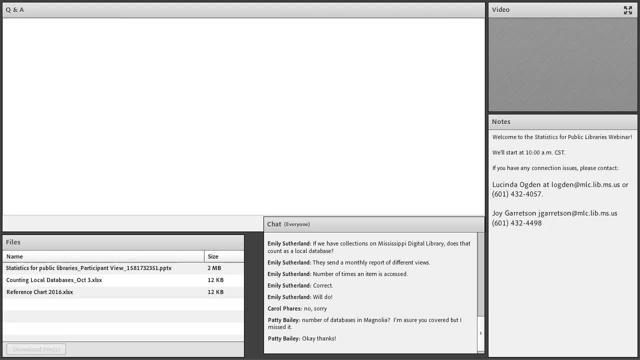 questions. okay, I'll give you all just a minute or two to download these, but thank you for watching and I'll see you next time. you so much for coming in here today. we're so happy to see you. hope you got some information that can help you file your report. let us know if you have any. 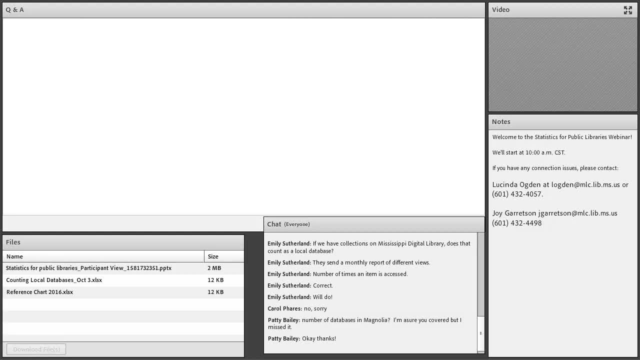 questions. we will archive. this webinar should be up, I'm hoping, by the end of the week, so if you need to watch it or look at any portions of it to help you complete your report, you're welcome to do so. hope y'all all have a great day.